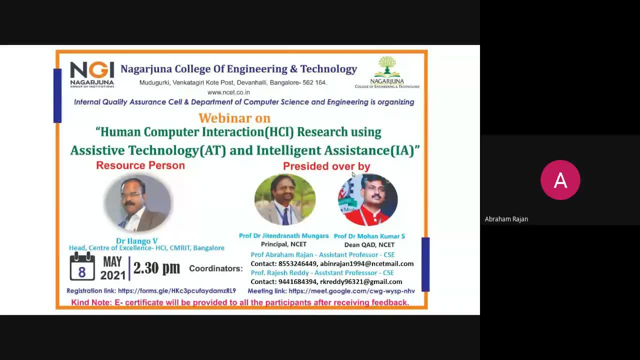 and national professional societies and forums. He is a reviewer and an editorial board member for various reputed international and national journals, conferences and symphoniums. He has published around 16 patents. as an inventor in the area of Information and Communication Technology, Dr V Longo is the author of over 90 scholarly research papers, including 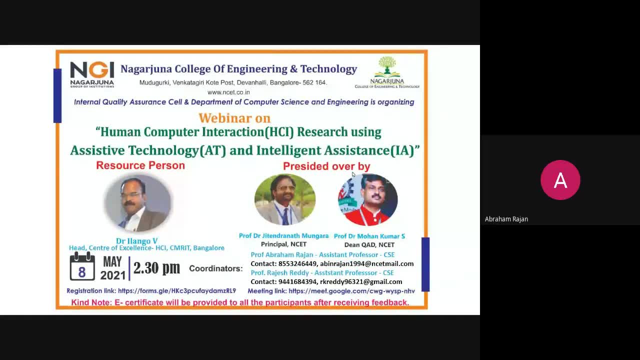 40-plus research papers. Dr Longo does more than Elder, appears to be referred to as former reputed journal papers, which are Springer, IEEE, WSO and Scheme. He has produced one PhD scholar in his supervision in VTU and he is guiding six PhD scholars under Vishveshwaraya Technological University. 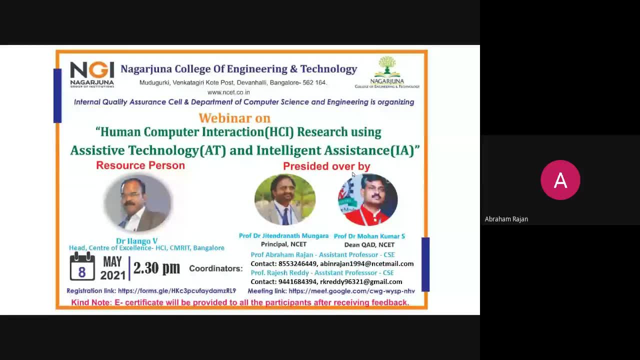 Belgam Karnataka. He has also published books in the area of social network analysis, artificial intelligence, resource management techniques and user interface. He has delivered many expert lectures, guest lectures and webinars on AI and open innovation in India and abroad. 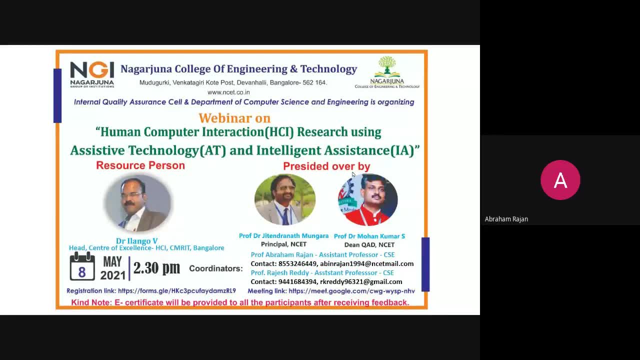 He has also delivered keynote and plenary speech in various national and international conferences. He was a publication chair for IEEE C214 conference. He is also a UX UI consultant. He is also a doctoral research committee member for different universities in India. He is working in machine learning and decision support field for the last 15 years. 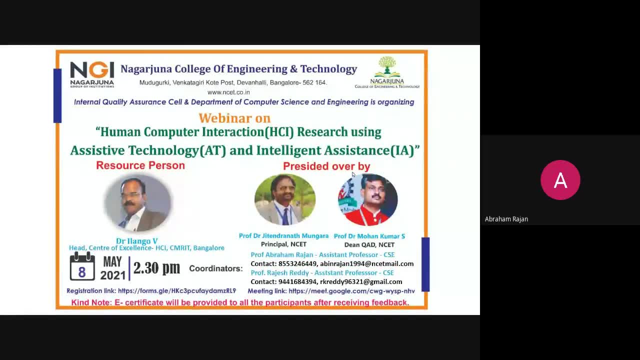 including his expertise in various fields such as model building, optimization, user interface usability engineering and prediction and forecasting research. His current research interests include healthcare data sites and analytics, cognitive engineering, personalization, user experience, medical image and video data analysis. 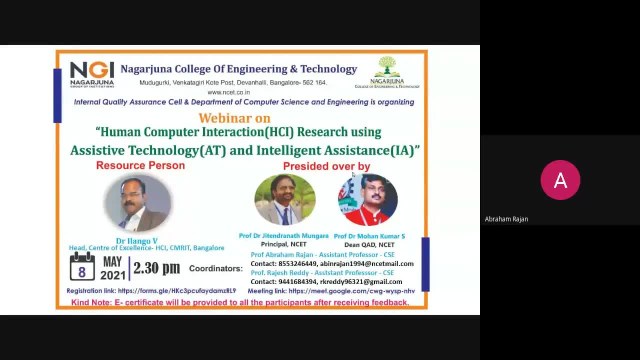 It is my privilege to introduce our speaker, Dr B Ilungo sir, to our esteemed audience. Welcome, sir. Thank you, Mr Abhishek. Thank you for having me on the program and I would like to thank you. 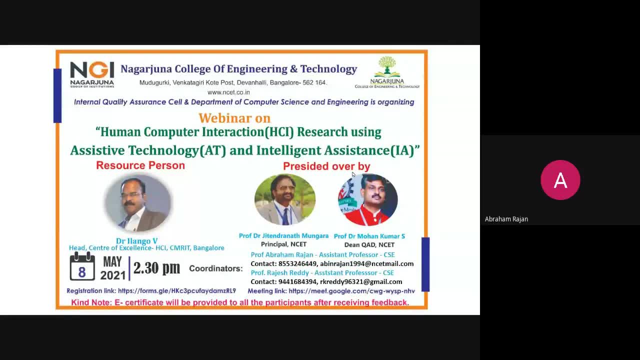 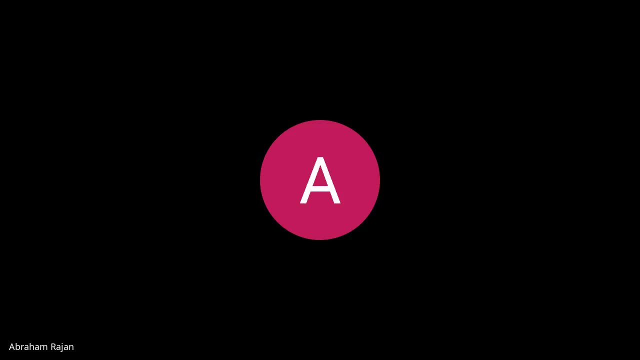 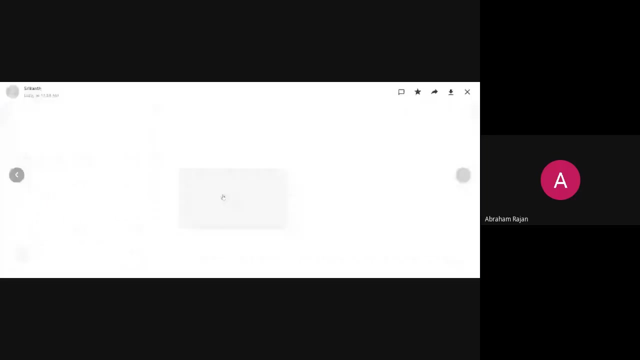 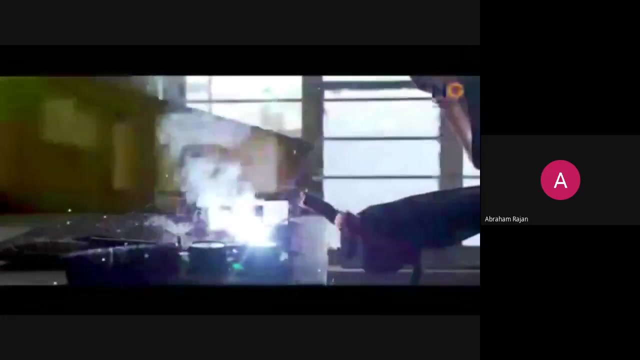 Sure sir. Now, without further ado, we will turn the time over to introducing our Nagarjuna College of Engineering and Technology to our speakers and participants. So please be seated. Dr B Ilungo, you are very welcome. 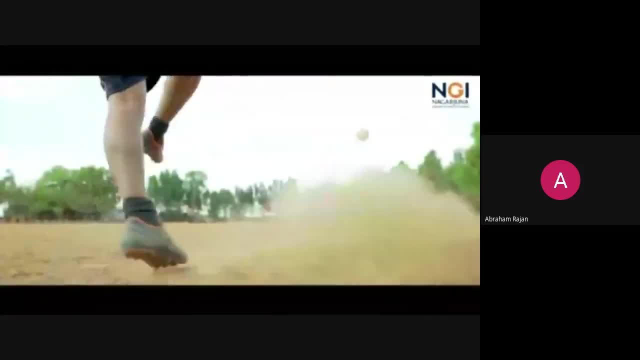 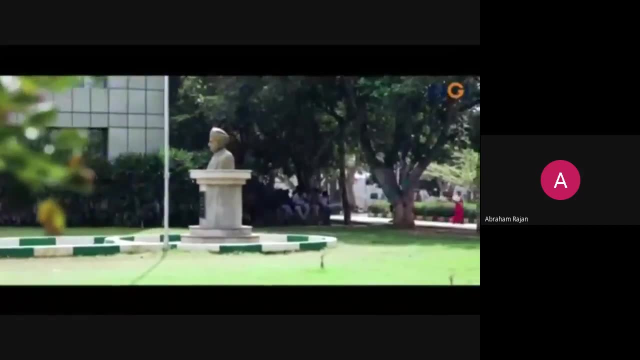 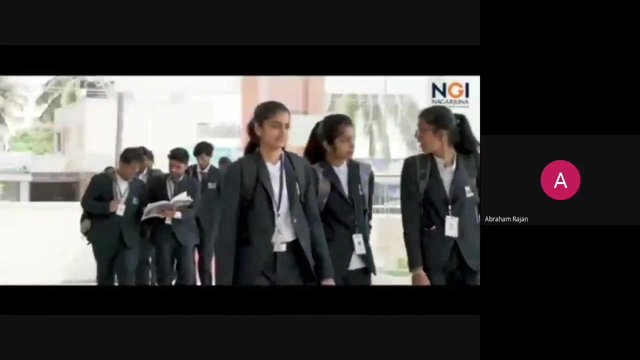 Thank you, sir, Thank you, Dr Ilungo. Founded in 1995 by Sri JV Rangarajo Nagarjuna Group of Institutions, has emerged as a public institution, an epitome of educational excellence, and has stood the test of time ever since. we stand strong on the. 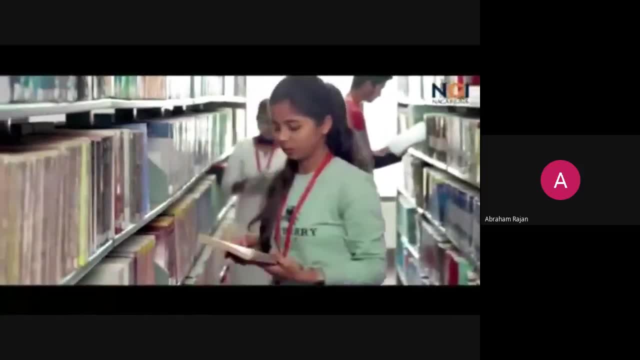 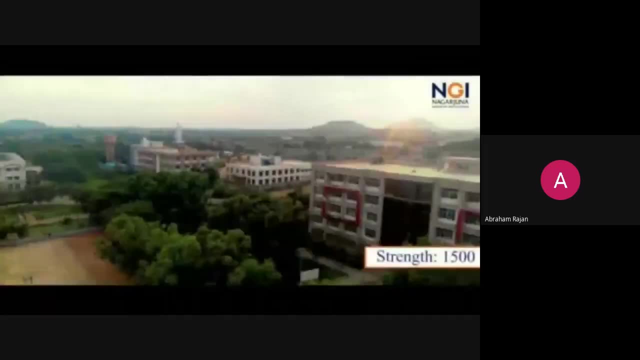 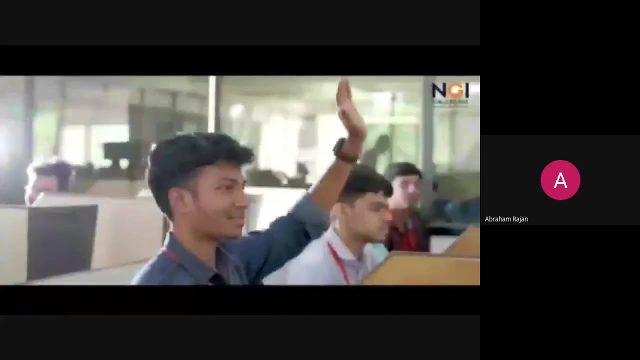 pillars of academic professionalism and educational distinction. our reputation lies in our unique offerings to students via our education. with more than 10 000 students nurtured by 1000 plus exceptional faculty at naga archana, we focus not just on academic development, but also on a 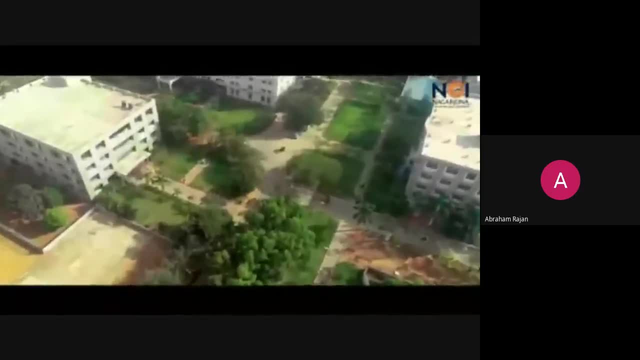 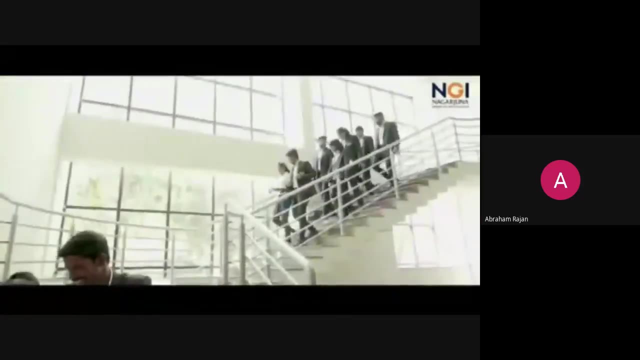 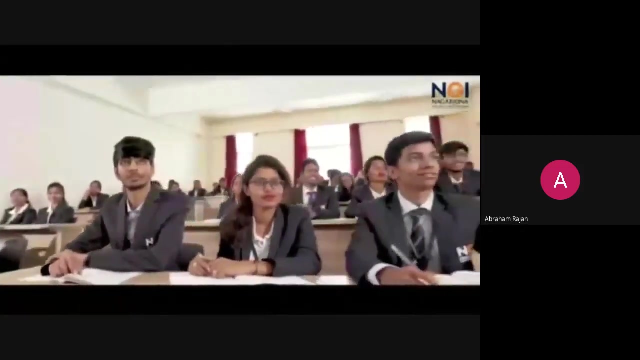 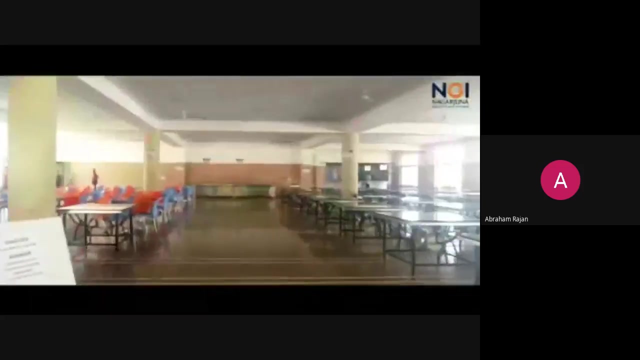 student's overall road. our lush, green, 100 acre campus offers an environment conducive to learning. our sterling infrastructure is equipped with modern amenities: well-equipped labs, smart classrooms, wi-fi enabled campus, indoor and outdoor sports center, gymnasiums, cafeteria, hostels. at nagarjuna, we always aim to create experiences with our learning process. 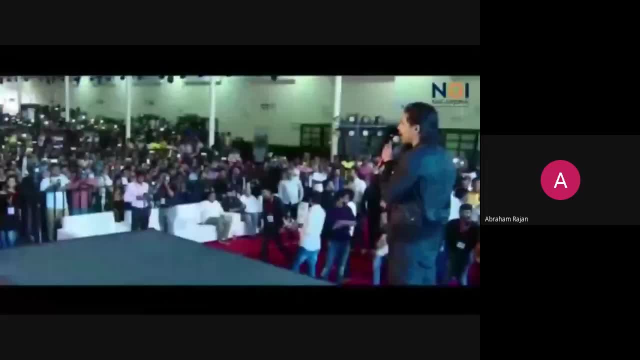 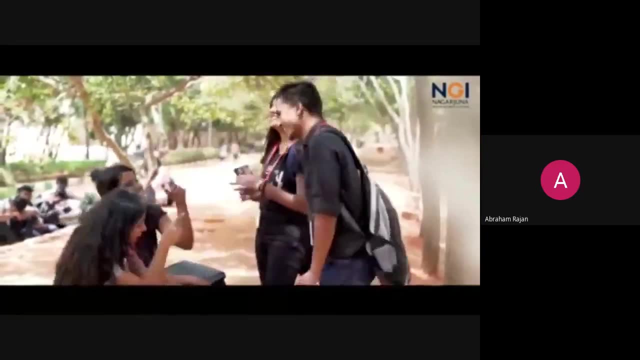 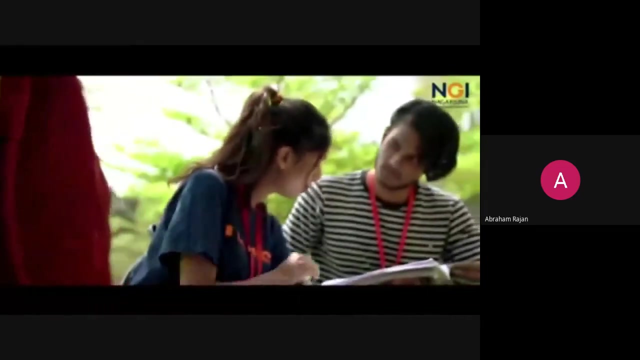 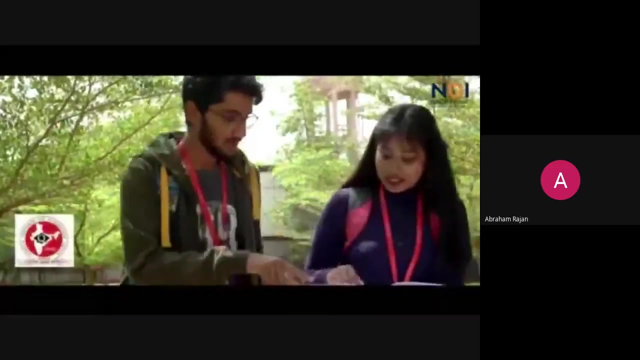 many activities, events, seminars, workshops and fests are organized on campus to enhance the overall development of the students. ncet is our college for engineering and technology. it was established in 2001 and it has been approved by aicte with nbu a accredited courses, accreditation with a grade by knack and iso certified for its green initiative. 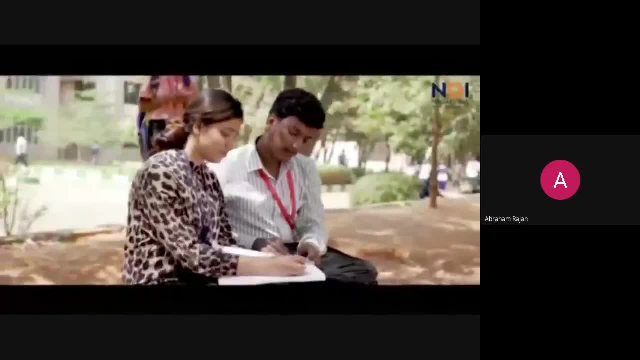 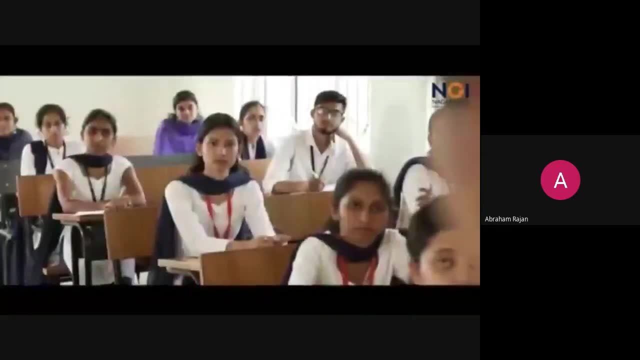 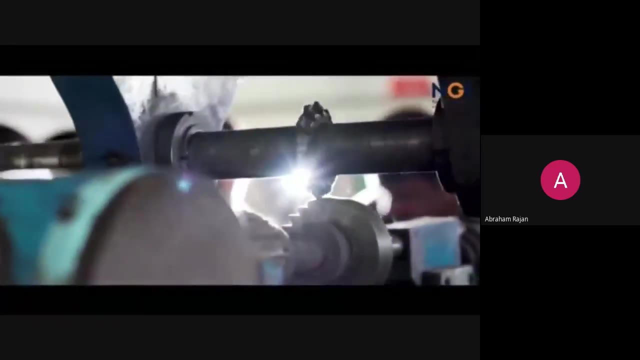 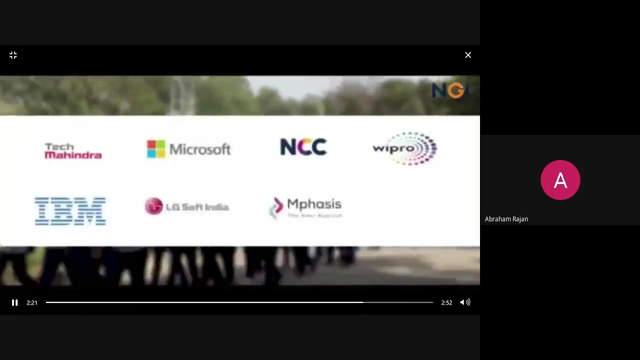 it is one of the most prestigious autonomous institutions in the state of karnataka. at ncet, we emphasize on practical learning as well as academic theories. we follow a student-centered pedagogy and have a project-based learning system to make students future ready. we are associated with reputed organizations that offer excellent employment. 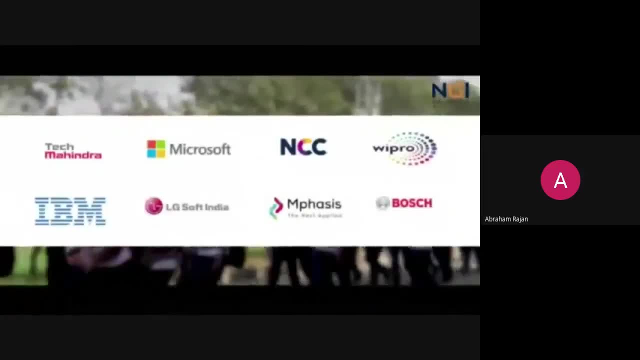 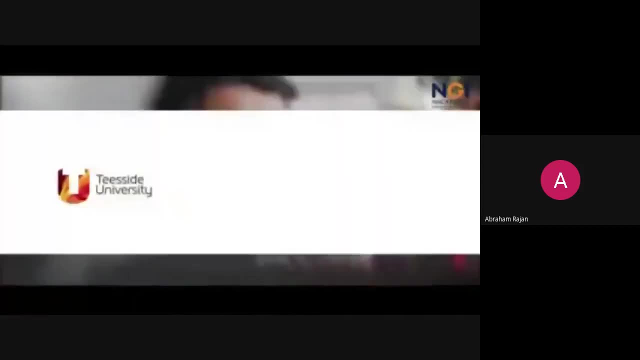 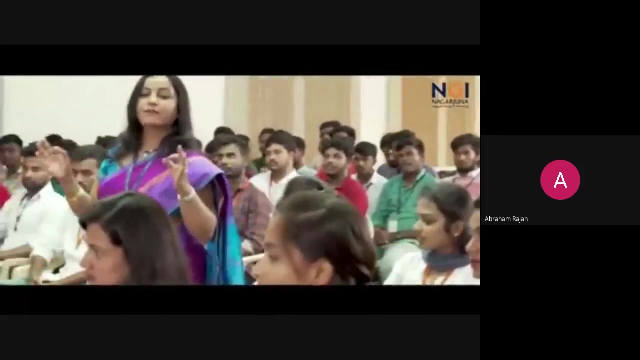 and internship opportunities to our students. the international internship opportunity provided for the students helps them to widen their technological horizon. we are associated with some of the best technical universities in the world. our highly disciplined placement training center prepares students right from the first year on various aspects of the interview. 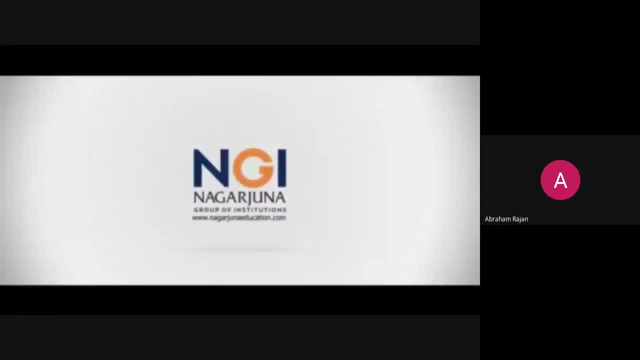 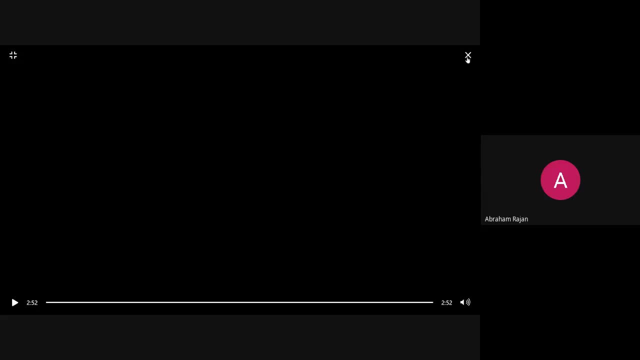 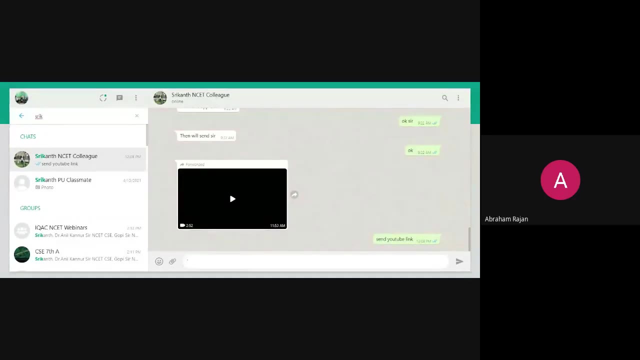 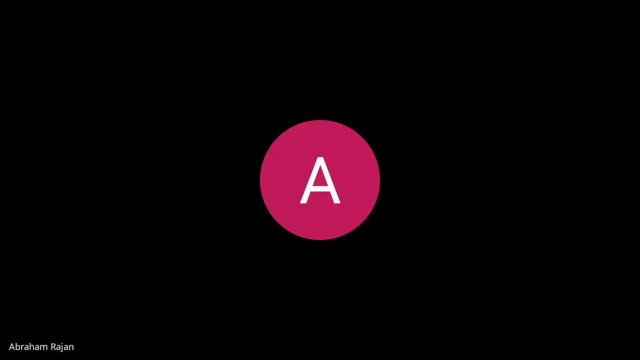 so thank you all. thank you all for your patience. now i would like to request our speaker to take over the session over to you, sir. hello. hello, mr abram. shall i start my presentation? yes, sir, you can share your screen. yes, professor, sir, please, yes, one second. 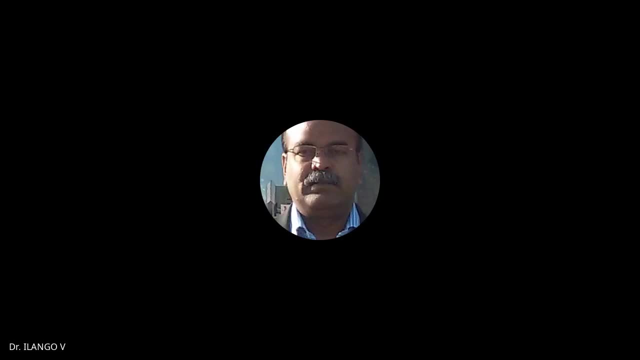 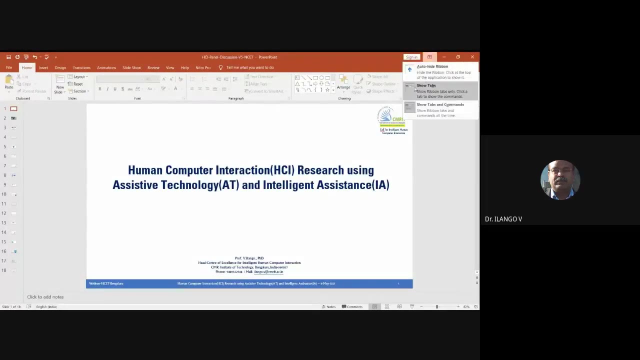 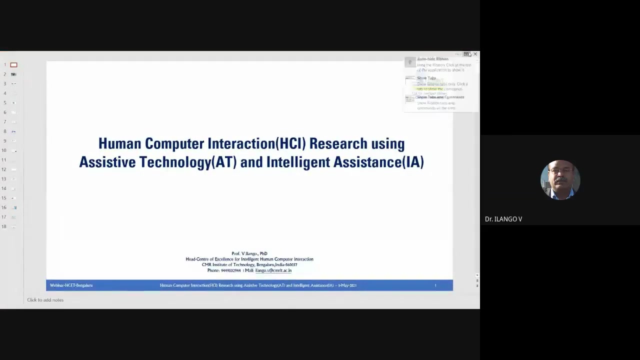 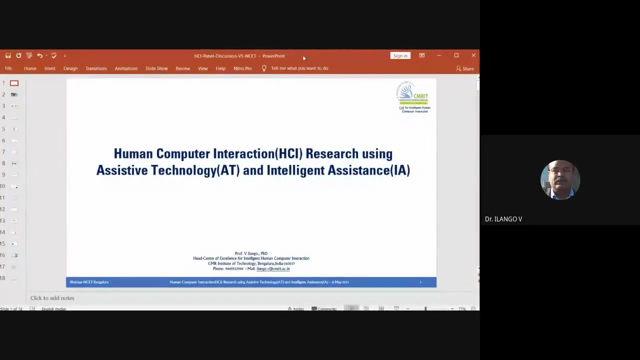 go ahead. so you have started. we need to say that to you. go ahead, thank you, all right, thank you, thank you. the screen visible to everyone. yes, sir, it's visible. sir, yes, uh, firstly, uh, good afternoon everyone. firstly, i would like to thank uh professor, dr djandra mungaru, principal. 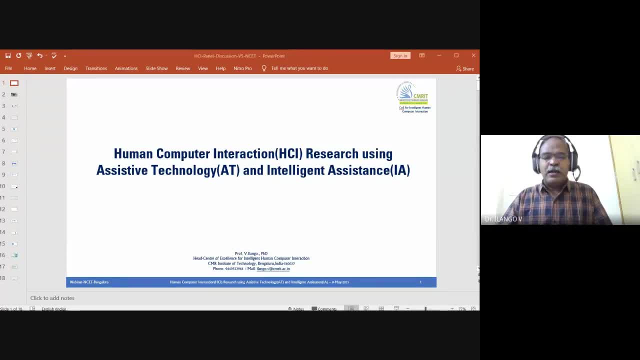 marajana college of engineering and technology and dr professor mohan kumar, dean quality assurance department, uh given me this opportunity to share my knowledge in this uh gathering. so thanks to non-original college of engineering and technology management also, and thanks for the participant for attending this seminar. so i will host now so you can have the question. 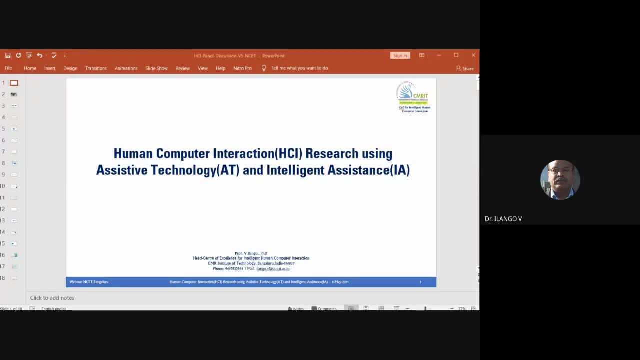 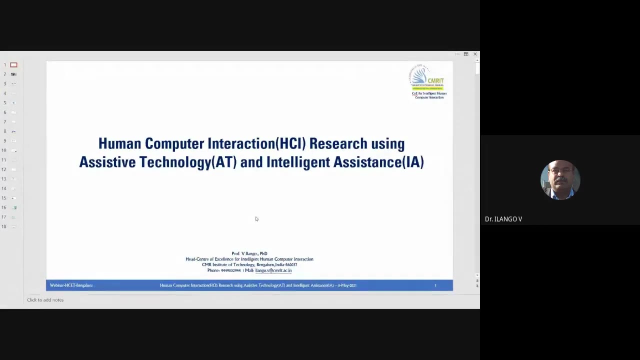 we will discuss the questions after the presentations. now i'll share it. is the screen visible to everyone? complete screen? only are able to see. it's visible, sir, complete, thank you. thank you. before start i would like to have some statistics from the gathering. how much percentage students attending today? 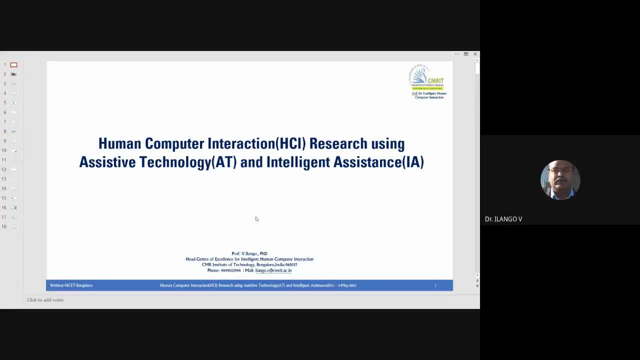 may be 75. 80 may be there. in the 80, 75 uh. graduate student. undergraduate student: how many percentage will be there? anyone can say around 70 for the percentage professor. thank you, super undergraduate right. any research scholars are there? how many percentage will be there? 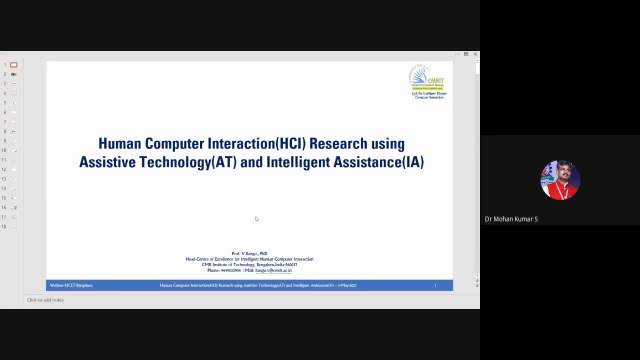 maybe, uh, five to ten percentage professor, because the professors are also research scholars here. yeah, let's say i exclude professor there teaching also, so they have maybe five percent. okay, this is very important. any pg students are there. oh, we don't know exactly. sir, right? no, no insurance, right? the reason why i asked for 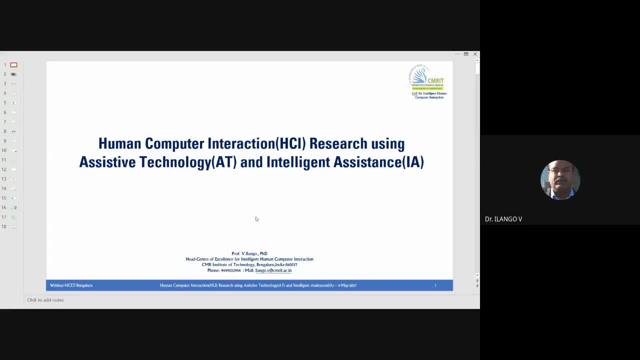 the statistics is very important because there is a always idea class 20th century expert, 21st century bond. so So I am very happy to hear this gathering maximum 21st century. your graduates, probably 2000s, later 2000s only majority of the ex-people who are attending here- go on. that rest all may be 20th century people, but anyway it is good we can have a good debate during the sessions. 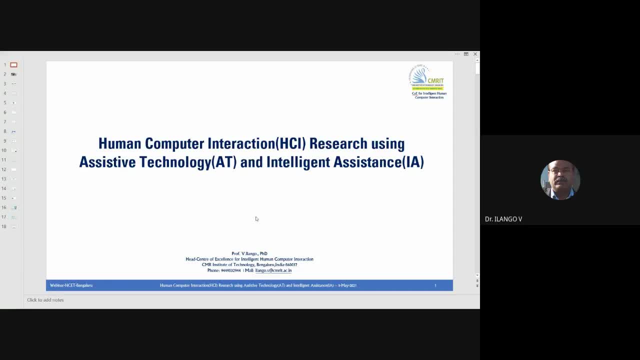 Right. so this is very important, to have the discussions why 21st century is very important. what was missed in 20th century? what is the lot of drastic changes have happened in the 21st century. we must know that. 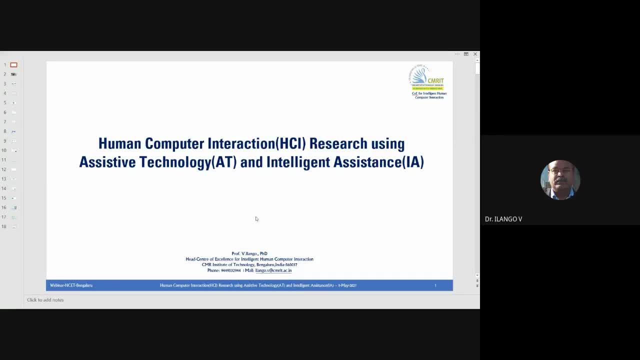 In 20th century also, technology was there. that technology was different technology. today we say that that is absolute technology. 21st century emerging technologies are there. Right, That is really simple and elegant as well as affordable. so people move towards to the technology side than themselves. they are not believe themselves. they are losing trust on themselves- lot of cases we can discuss in this forum- so they are moving towards that technology. if you see that 20th century people are not dependent on technology. technology was dependent on 20th century people, but 21st century people are dependent on technology. 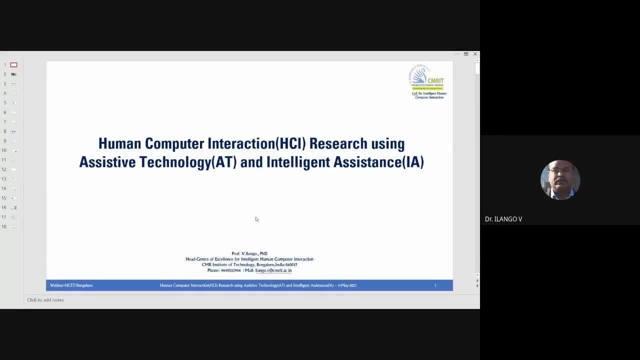 They are not dependent on themselves. so this is the biggest scenario available in the market. in this scenario, who play major role? is it the technology play, or technique play or hardware or any other instrument play major role? it is a big question. 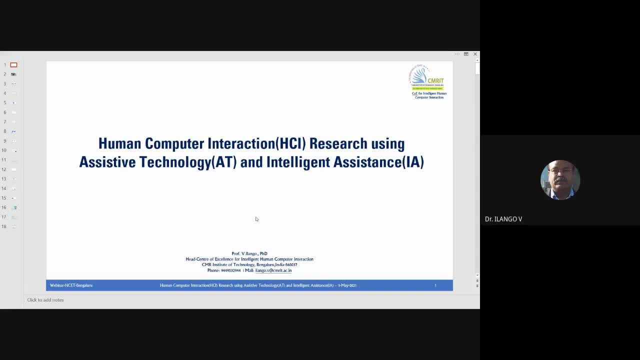 Actually human only play major role. there is an interesting debate: human, 20th century, also human. 21st century, also human. everything is surrounded by human Right Right Right Right. Technology is invented for the human being only, by the human being only. 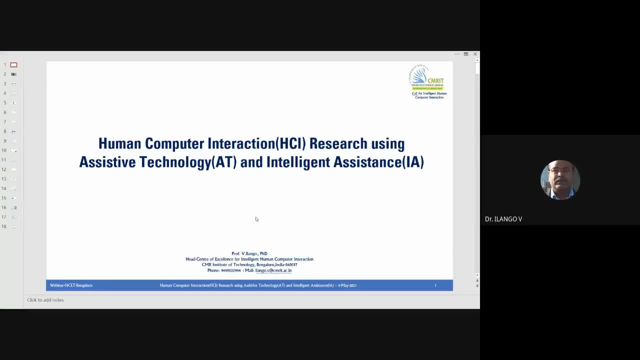 So, though, we are 20th century born, but still we depend on certain technology. without that technology, we are not able to survive today, but without certain technology, we could survive successfully today. so this is the differences available. even today, people want to go for cycling or swimming. people need technology, they need some mobile app or they need somebody's assistance. so why it is like that? 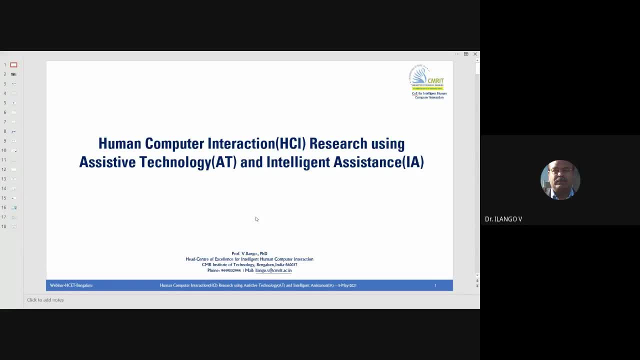 Right, Right. we also went for cycling. swimming. we didn't, did not have any support. the self-learning was more. we use our cognitive ability. we observe some swimmer, we observe some cyclist. based on that, we used to do manually. we learn it better. so asan, today we asked to raise a question: what was low? 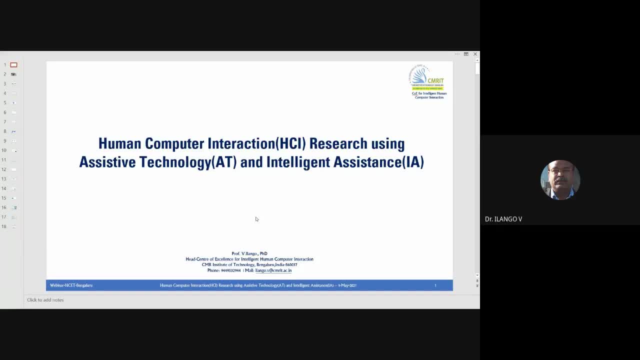 intense standard. probably nobody would remember that. what was learned in cycling 20 years before? today, the cycling can be done. that was the concrete mechanism, the existing technology. emerging technology is teaching how to do cycling, so is it needed? so observe the scenario, then learn and do the cycling. learn from that app or any other dynamic instruction. doing cycling is there. 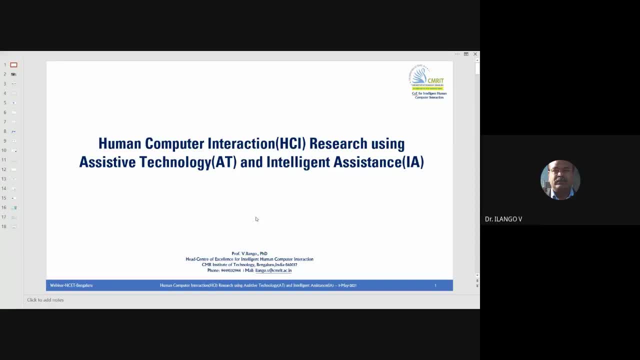 any differences can anyone justify? is a major difference? no difference, yes difference. so so 20th century, probably some of your parents might learn cycling. they observed their elder people through that, they practiced, they tried trial and error, experimentation. they also got wounded, but they like that, they learned it is very steady, strong now. now also they give them. 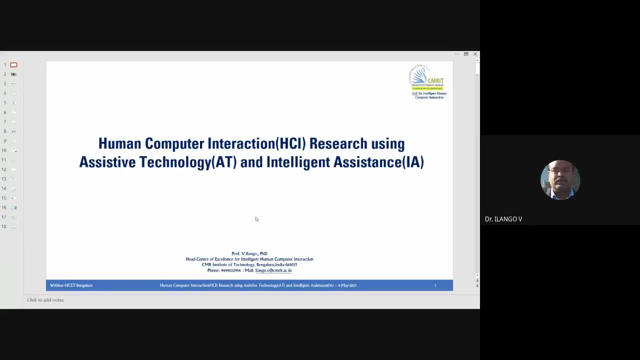 cycling for 60 years people, 50 years people. they used to do beautifully, but is it happening now for that? we go for simulated software. with the simulated software, excuse me, we learn mentally, we learn. then we go for uh, cycling systems presently. is it happening or not? so this is the huge gap, how we have to build this gap right. this webinar is going to address. 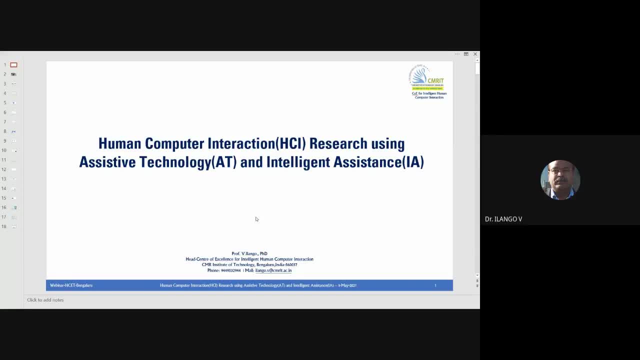 human centric concept, basically, human and computer. how they interact to find solutions for the problem. how they interact to design the product for the problem. what way the interactions are happening. there is a research approach. what is the research approach- a human and computer together- going to do for welfare of the society? 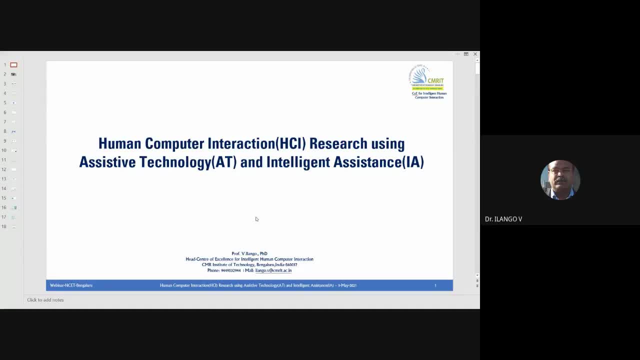 either for construction of society as well as destruction of society. both are happening. restriction also there with the technology conceptions. it up to people how they are, the learning and the knowledge based on that you can optimize that. okay, so in that scenario, 21st century, there is a terminology: assistive technology. 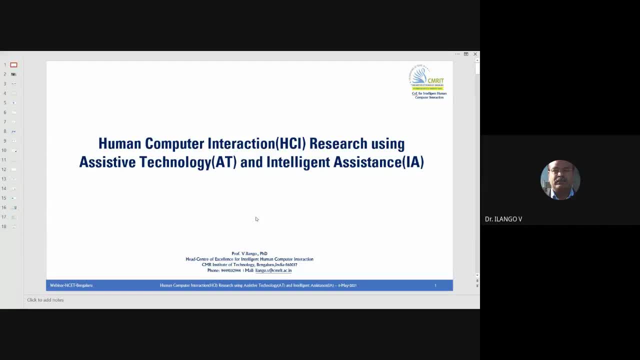 technology. what is assistive technology? we are going to discuss why it is important, where it is by a major role: intelligent assistance: is there any difference between assistive technology intelligence? yes, there are some differences. we will see to that. the intelligent assistant, the technology, should assist people in intelligent way. it should not trouble, just like that people. 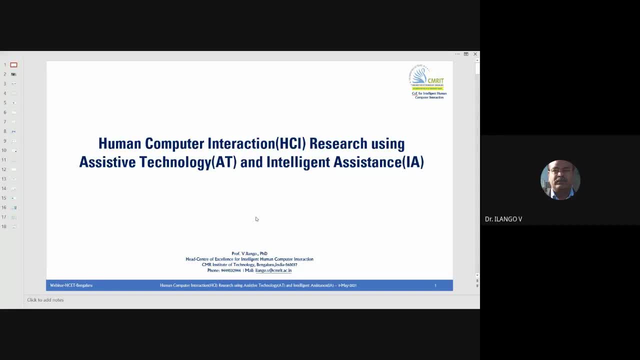 so in the 18th century, stream engine was there train? now, 25th century, electrical, uh train is there. people train is running with electricity. even speed is more so it's intelligent way of functioning there the electric steam engine is a. it's also assistive technology. 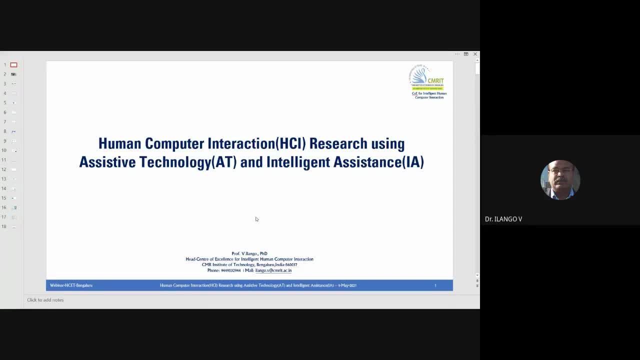 carry so many luggages from one place to other places. so what is the intellectual gap here, what is the challenges available here, what are the research availabilities, research problems or scope to do research available here? this is the way the sessions will go, maybe for 60- 70 minutes time. initially i will tell about conceptual idea and then case studies. 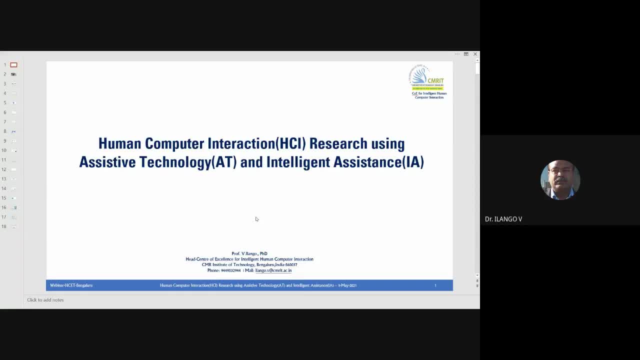 then i also real project which we have done, which we are doing it at present in our research area. we will be. i will be showing some demo after that. anybody interested to interact for the research mindset or research workers, you can interact. we will focus them right. so this is a basic. 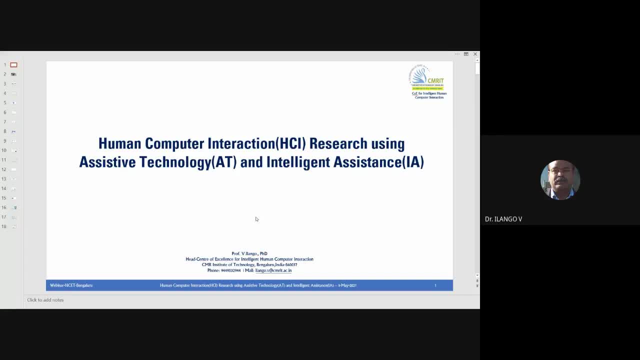 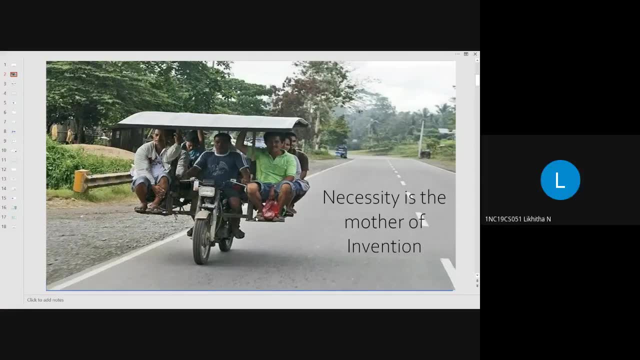 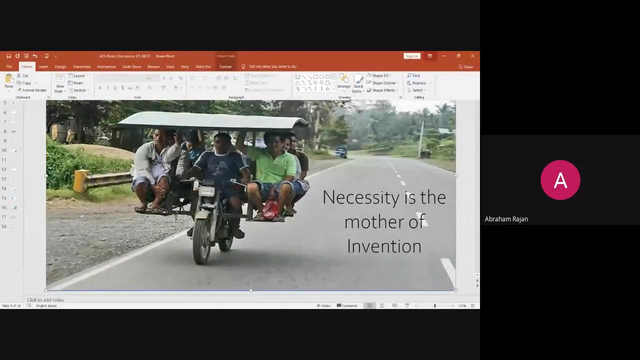 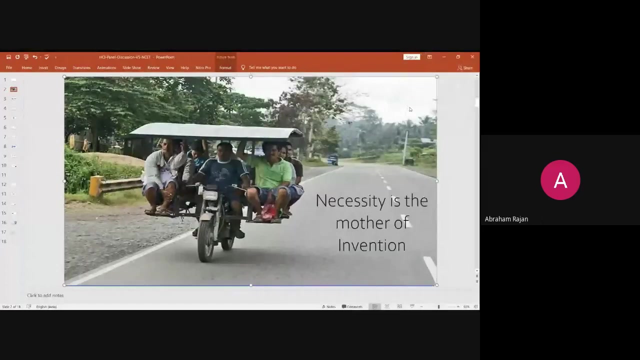 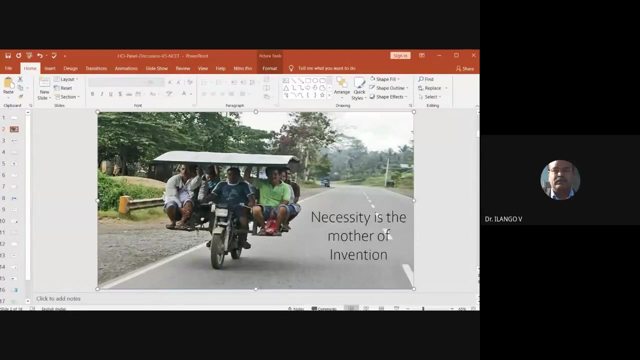 introduction for everything. when you talk about research, the basic thing is innovation. you need to be innovative. some voice disturbance is there. excuse me, somebody can mute nikita. mute your mic. you can continue, sir. sorry sir, you have to unmute your mic. sir, sir, unmute your mic. yeah, are you able to hear my voice last five minutes? yes, yes, sir, yes, sir, just. 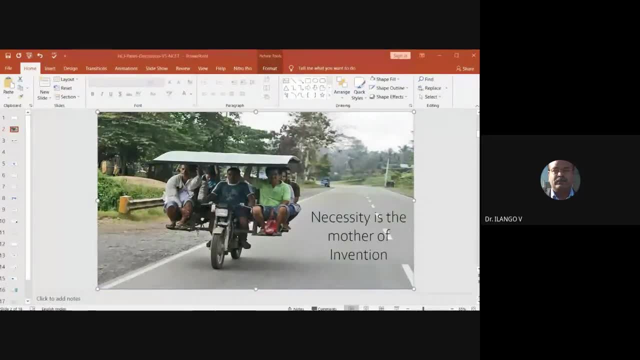 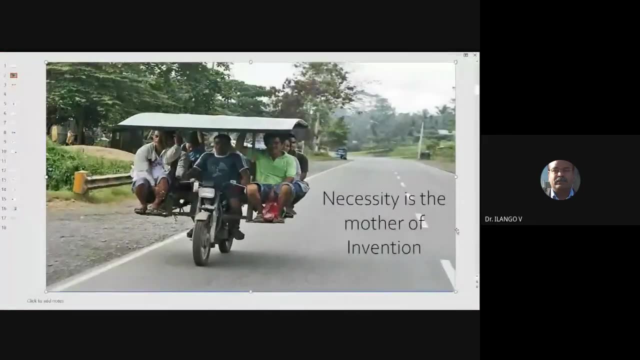 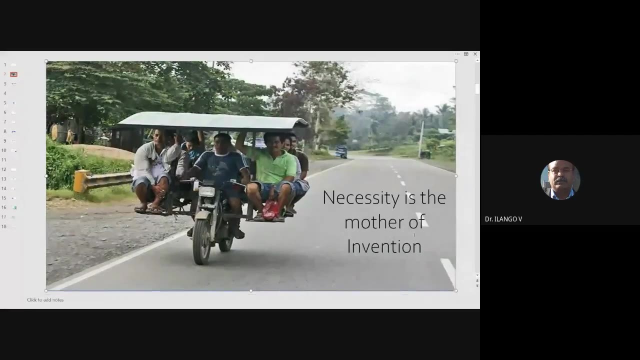 now. oh fine, fine, anyway, it is working. okay. now you need a mixture of the audience for theия ab initiatives. now can you hear me? yes, sir, okay, yes, now it's fine. yes, sir, right. so anything is there. present 21st century. there is a plenty of requirement. requirements are: 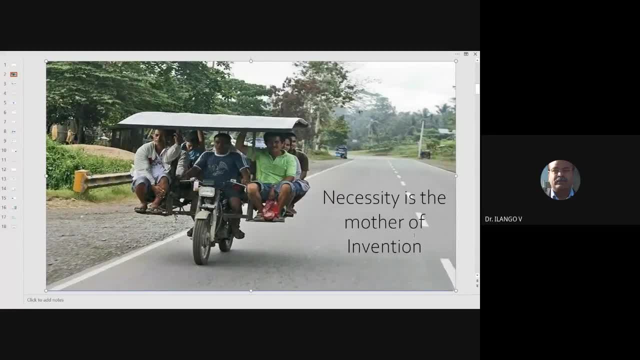 plenty thinking or plenty Assistive technology, intelligent assistance- should we find more or should we stop with that? Self-satisfaction is there already. whatever is existing in the market? okay, we will stop with that. We should stop like that. No, We need to go further. We need to go further. 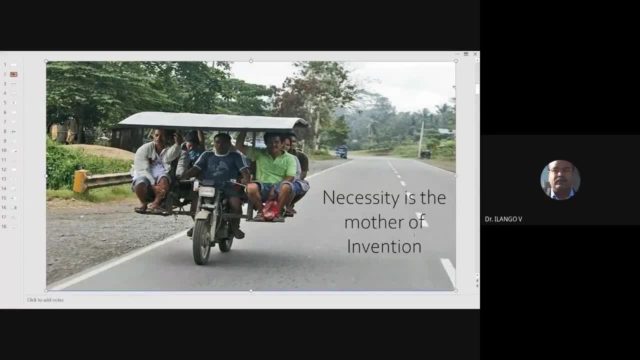 So many groups of communities are there. Each community, there are certain requirements. We need to find that requirement. What would be the right requirement for them? We need to develop, We need to invent, We need to construct a prototype. So this is the present scenario. Just look at this picture. It's an ordinary motorcycle. 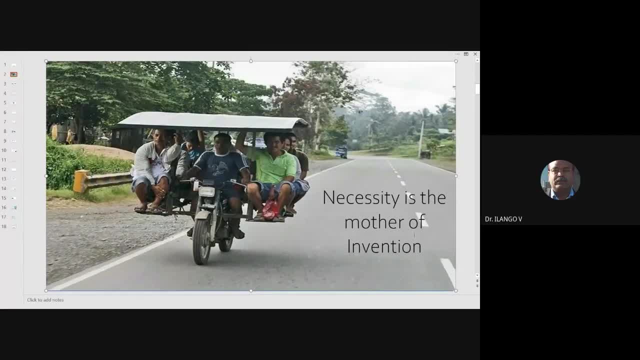 The motorcycle. if you go in a normal way as per the motor rule, you can go maximum: back side two people, front side one child, small child. Maybe four people can travel. See the gentleman how he has invented new idea. So almost seven to eight people are traveling in this motorcycle. 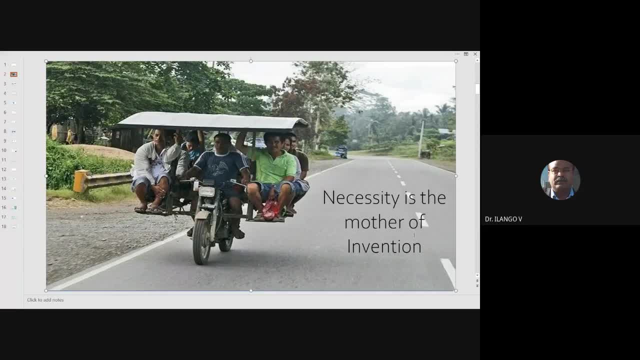 This was invented during pandemic 20 March. to today, somewhere in northeast India, This has been invented, So it is very much appreciated. fuel consumption: seven people travel, even auto. we cannot go this many people. but this prototype is not been accepted. 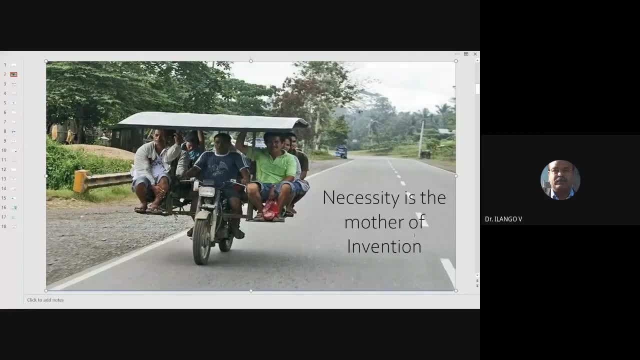 There was a criticism. See the utility, usability of this invention. It's really appreciatable. Many are going, many beneficiaries are appreciating that. but constructively, this is not been approved. This has been discouraged. This is not the right way to invent that. 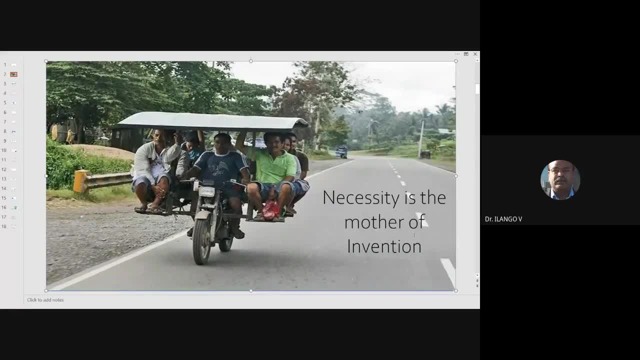 So what to do that? Why people Stop this kind of invention? Is there any mechanisms to do that? Yes, So anything we do the invention should be done in the concept of a proper methodology. So let us see how to do the methodology. 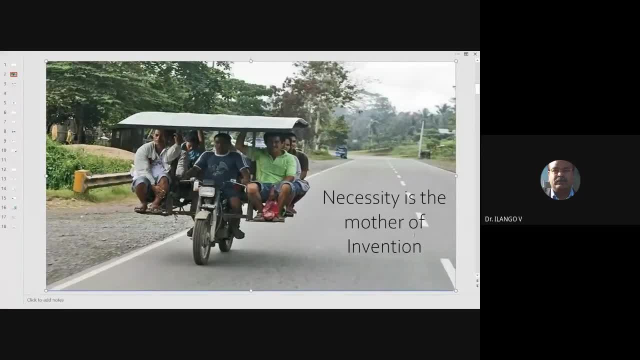 But this invention is appreciated by tech Mahindra. Anand Mahindra is appreciated this inventions. Probably he would like to motivate these people and educate them to come up with the formal prototype. If it is fine, he may be going to develop. 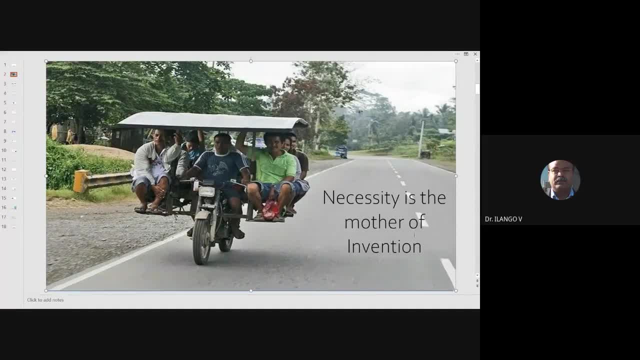 He may be designing a vehicle, he may launch it in the market, but this is less petrol, maybe battery vehicle. So this is an invention point given to society. Someone can modify this prototype, or the same group of people can modify. They are not educated. 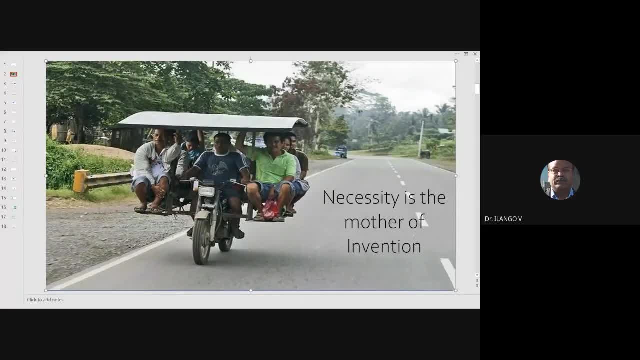 They are not educated as we are having knowledge, but how creatively they have done it. So this is a way that the transformation step took place in the 21st century because of the cognitive engineering. The cognitive engineering is brain related. For that we do not have any formal education, so any formal qualification. anybody can think creatively. anybody can design creatively. anybody can make a product creatively. 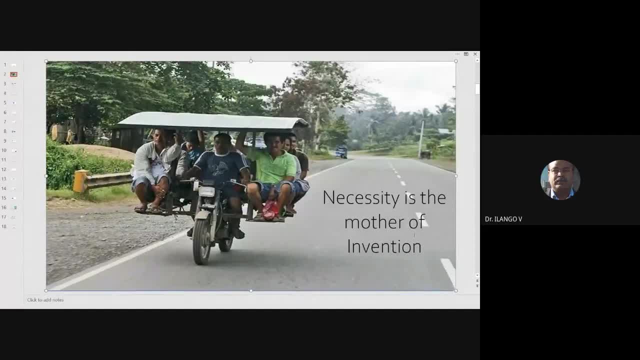 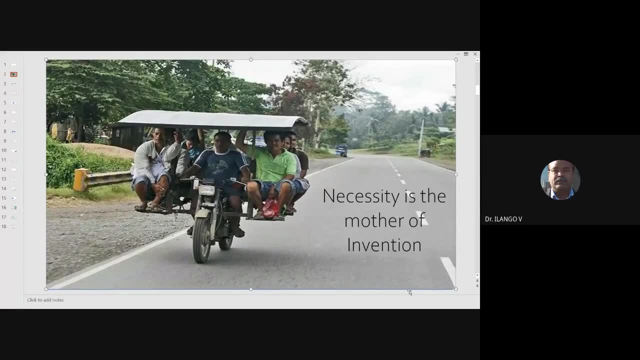 So 21st century cognitive engineering play a major role. That's why so many inventions, innovations, are coming into pictures. It's fine. Let us justify how it would be possible. See the evolution of computing, since you are from computer science. 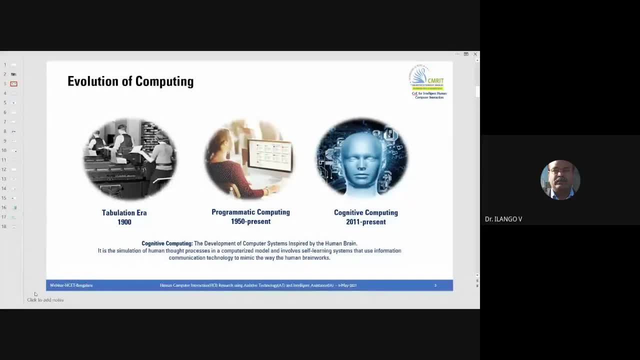 The evolution of computing In the 90s, the last century probably, people were using maximum of table the entry data and calculating values like that. That's a population up to 1970.. The population was thereafter a new, new desktop rating system concept and the character user in this concept. 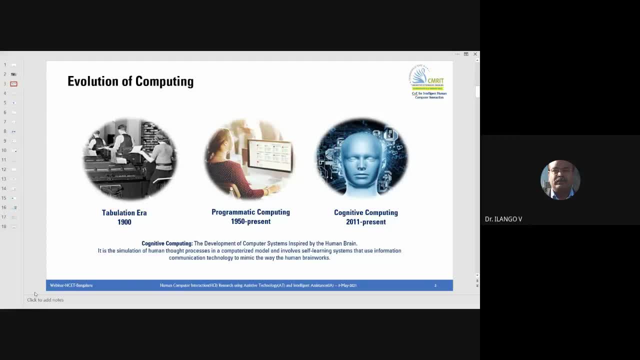 And the database type of software came into the picture later in 1980. New type of networking And later in 1990, the system started. The programming concept started in the mid of 19th century, 1950 onwards. The programming concept still exists in the market. 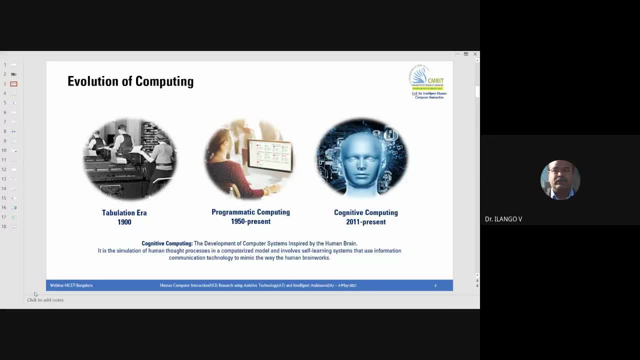 Programming concept is going on. now Different types of programming concept came into the market. No SQL without coding We can generate the script like that. Many things is there. We are learning that. beyond that, One more interesting thing: I told that 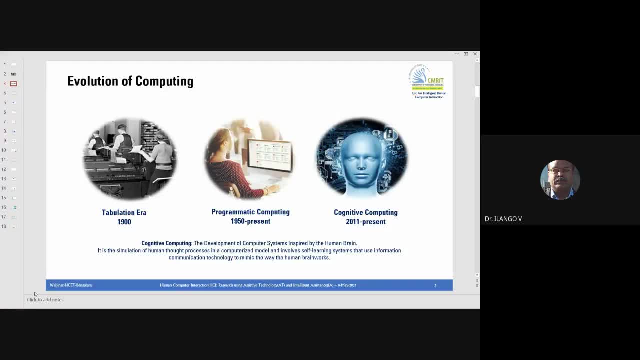 Cognitive computing. Later in 2011,. cognitive computing came into the picture. Cognitive computing is nothing. It is a completely brain, like a human brain. How it works? like that: System thinking simulating the action activity performance by the individual human being. 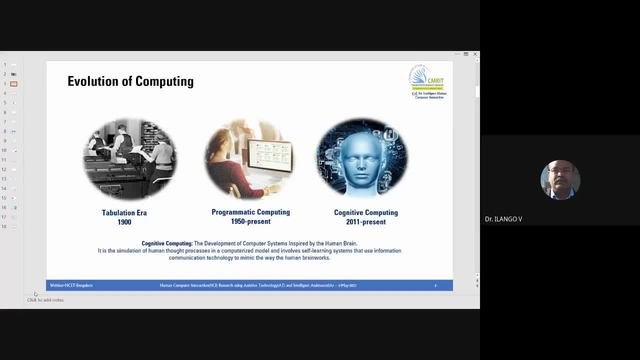 We can build a model. I think some different way, Like that. Mr Abraham and other principals and deans are thinking in different way. Everyone thinking is different, But brain- how do we make different thinking into synchronized way? Generic characteristic can be taken from each individual human being. 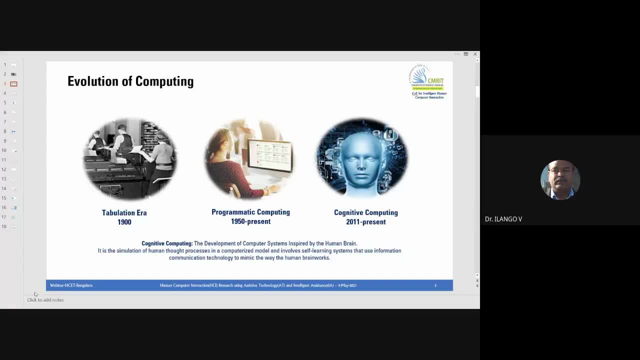 Can make a new model. That model can be executed. If you go over 7 million people thinking, then 7 million model neuro schema we need to construct. It is so complex But people are trying to do it today using different mechanisms like deep learning. 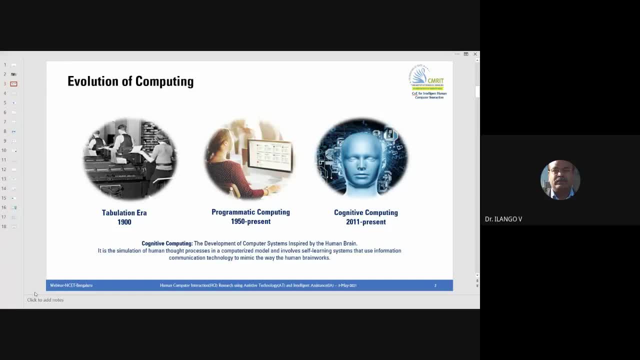 Beyond that, also brain and computing like that, There are many other computing, high performance computing, always coming to the picture. They are doing it, They are optimizing it, But they are not able to be efficiently effective, At least for similarity based. they are constructing the schema. 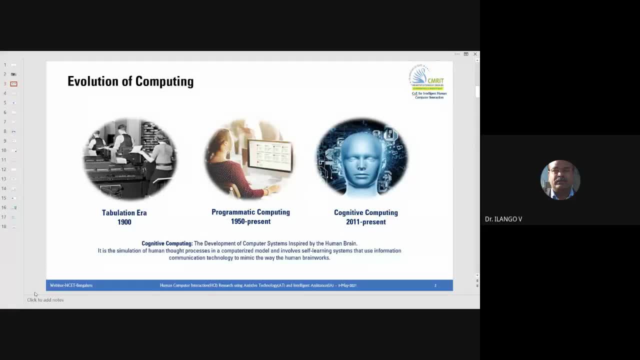 It is a wonderful mechanism. cognitive computing, Another synonyms you can say artificial intelligence. So through that technology people are getting transformation, They are getting more facilities, benefit for their day to day life as well as societal point And also life also. So what is cognitive computing? 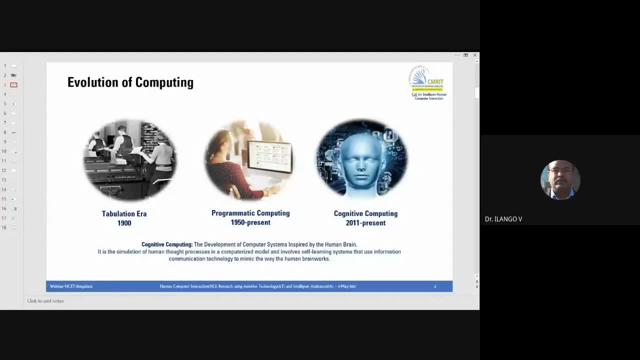 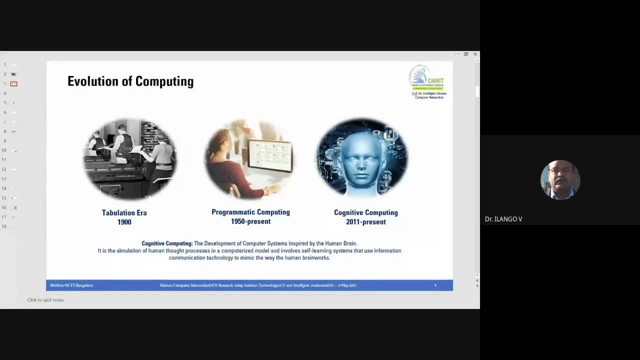 The development of computer systems inspired by the human brain. OK, It is a simulations of human thought processes in the computerized model and involves self learning system. So I told you in the beginning 20th century, we learn cycling without anybody's knowledge. 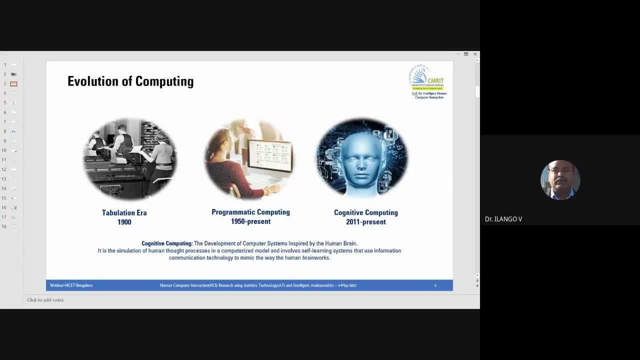 We observe somebody how they are pedaling all thing up. So we try with the small big cycle. We fell down, We got hurt, everything slowly We get experience. Then we become an expert in the cycling wheeling all we will do it. 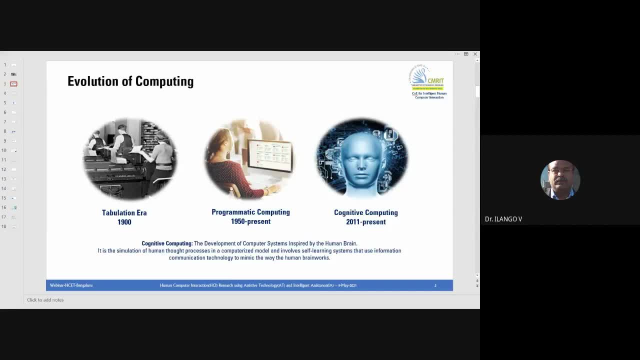 But today we have ad, we have video tutorial- so many things Through that we learn. Of course, people are learning quickly, They are doing effectively, No doubt about that. But however, that was the classical experience. This is a modern experience. 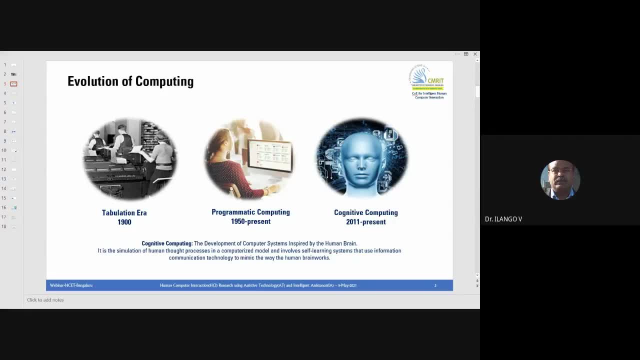 Both are fine, But ultimately the experience which was there, 20th century. You will not be able to get into 20th century. There is way, But your purpose is solved: Cycling superbly, doing pedaling A good thing. 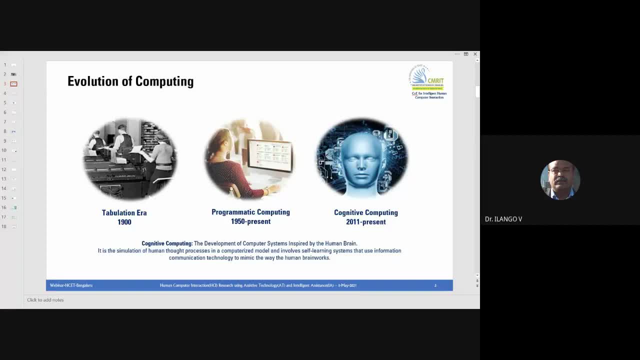 That way loading and making packages. That experience is really missing. present scenario for cycling: Even there is no back seat in the cycle. There is small seat for a cycle rider. today, So many compact system came Those days: Hercules cycle, Atlas cycle- big, big carrier. 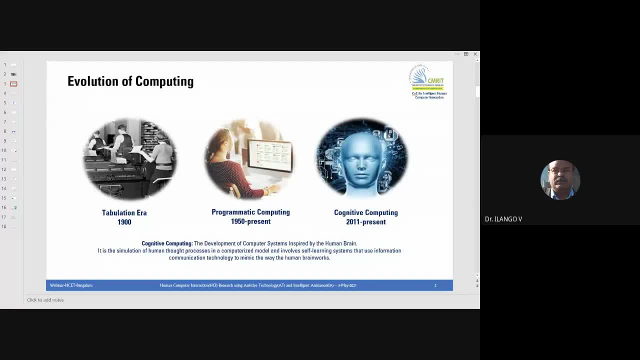 We can keep 100 kg rice That side. we can drive Like. that was the modernized mechanism. We did it. Now it is not available. Small cycle which can be kept inside the ground, or 5x5x5 size space also. 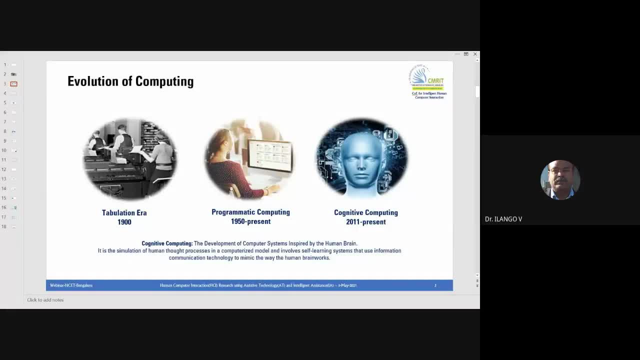 Right. So, however, we have to make a model, simulated model, computerized model- Each individual- I told 7 million people is there in the upper assumption in clover- All person thinking is different. Each person's neural schema is different. 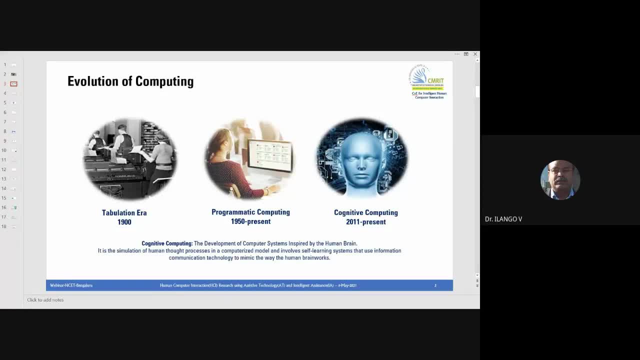 I mean brain. The function is different. So similarity wise, we can make, we can make one model. Dissimilarity wise, we can make, we can make one model. We can go for a multi-meter system, fused mechanism, Very complex. 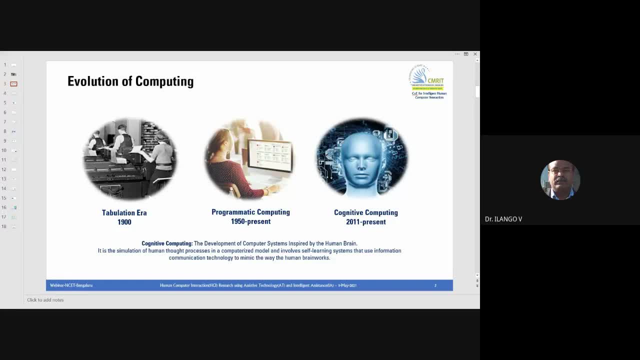 People work hard. They have done superbly. We should be very proud. Our computer science, our IT group really hats off to them. They have done super thinking, super modeling. Now we use that to use for day to day purpose Right. 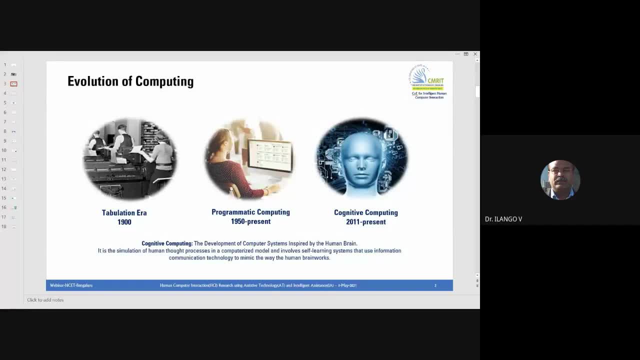 So this is an interesting thing for information. You know, to mimic the way of human brain works, how human brain works, So many robots have come to the other. In fact, recently the 2019, which was an antenna in December. 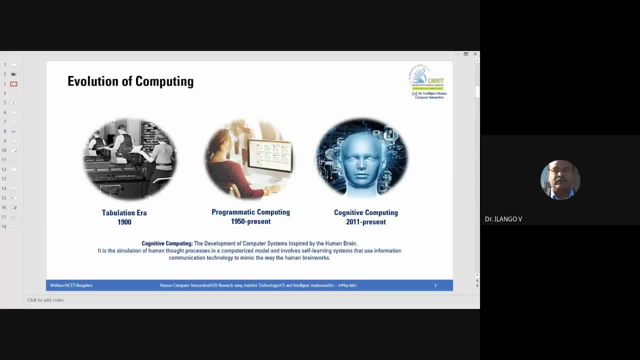 COVID-19 was there. thereafter So many innovation came, or touchless machine came to find the symptoms of COVID-19 and the robot serving people who affected- patients Also, I say human beings- having so many innovations. Okay, The system there is like that. 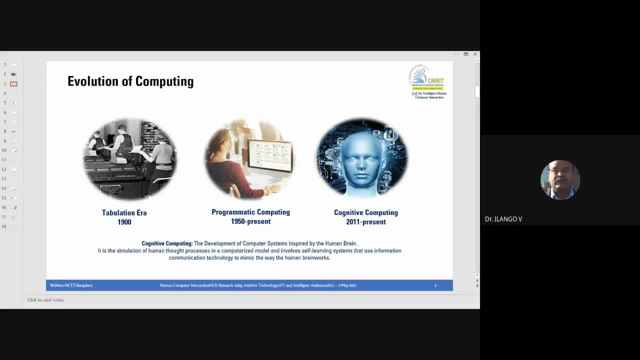 It may continue for another 20, 30 years thereafter. Some other mechanisms may come to the right time We need to do. human play a major role along with the computer. How do we do research in these things? Very carefully, human input interaction was such. 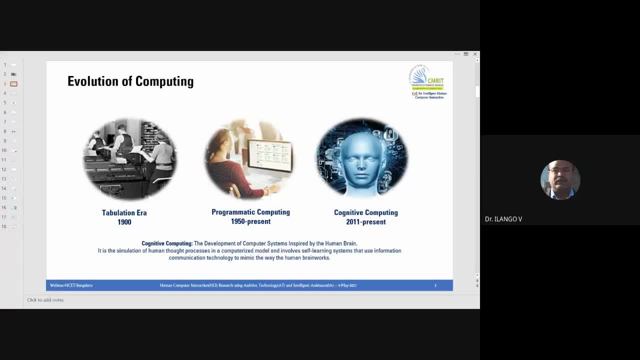 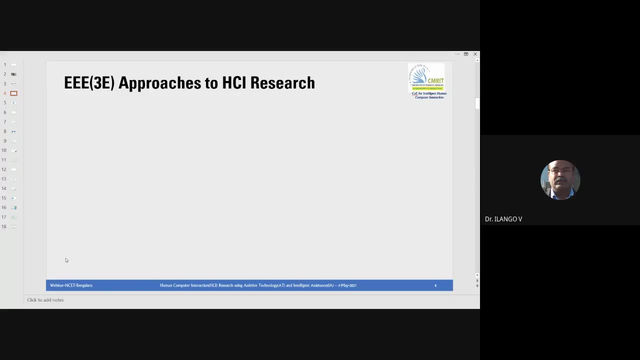 How. that is the biggest challenge we have. We need to optimize that. This is interesting things in front for a century, Right? So there are approaches, as we discussed human-computer interaction research, there are some approaches, formal approaches, approaches, three, three. you can say triple e, up, triple e. the first approach would be the empirical. 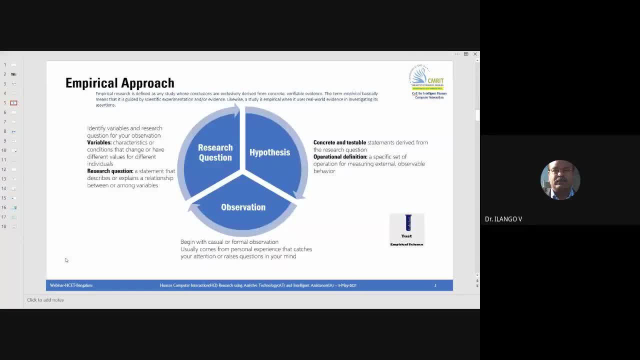 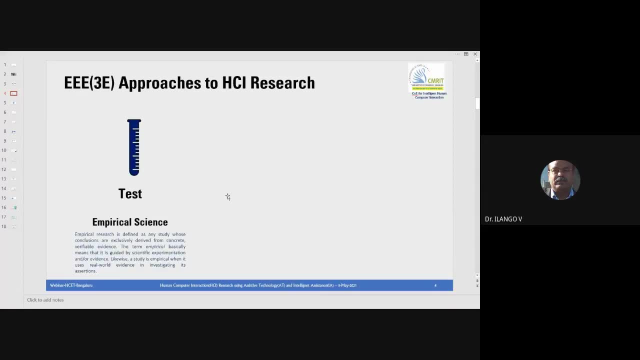 approach, empirical approach. so the empirical approach is a very interesting approach. so empirical approach, it is nothing. but we cannot believe just like that. whatever finding you say, we need some evidences. anything you do, we need some evidence. evidence based in mechanism. that is a empirical approaches, it's a scientific. so mechanisms also. for example, if you say for it, 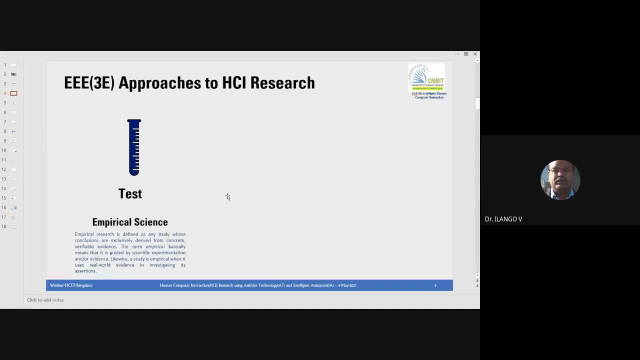 now somebody tested positive, somebody tested negative is very peculiar resulting. see here the negative result as the symptom. same positive result, also the same symptom: top is there, old is there and there is there, and fever is there. for a person, normal person, who does not have covid tested, rt pcr test is done. it. 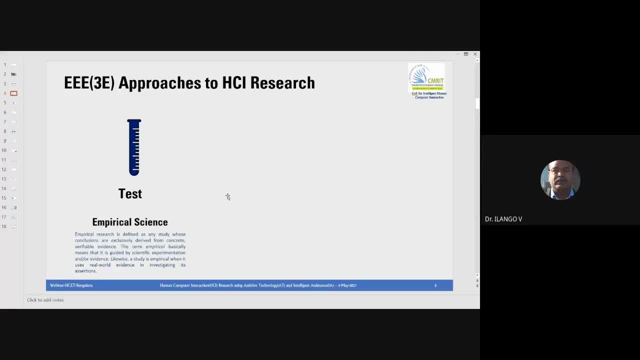 is being given. result is negative. the other way around: other person has got symptom, he's been declared as a positive person, he's also has got the same result. how possible? so where is the evidence? what way you tested? you tested only with the nasal saliva, all this only, or you went beyond. 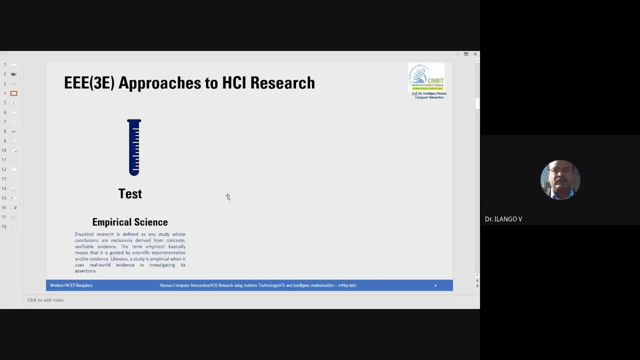 this is positive, this is negative. show me the proof. so we need to show the proof of laboratory test. what was collected sample? the patients are responded so somebody will not have the trust of the test result. i have all these symptoms. what positive person has symptom? i'm scared, but you. 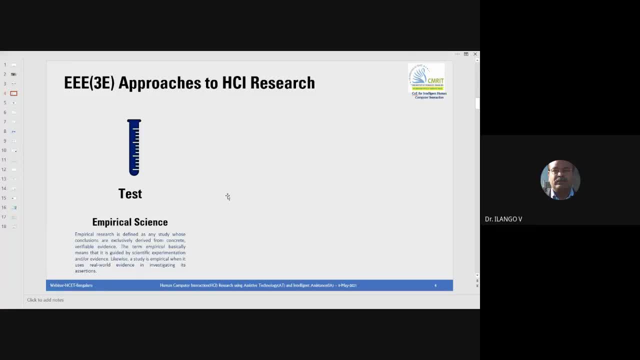 are not done proper testing. so i i have doubt. then they go for blood testing or something x-ray also they are taking somebody going for pulmonary testing now. it's now another don't know ct scan test they are doing now the ct scan testing. it showed some clear-cut picture, so 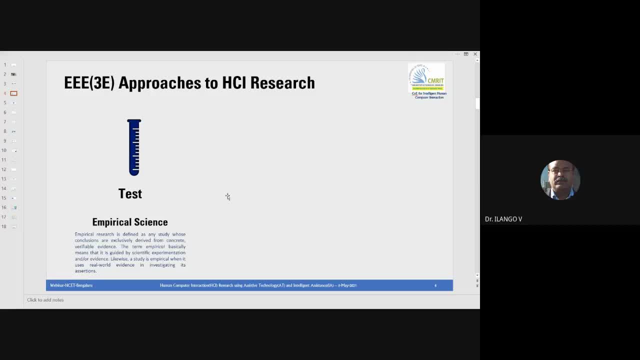 then they're confirming. okay, i have done artificial tests: ct scans, x-ray and pulmonary test. now i am confirmed. there is no. this is for me. i have to escape, but this is the way the mechanisms are there. this is a empirical approaches in that for every mechanism there is a computerized 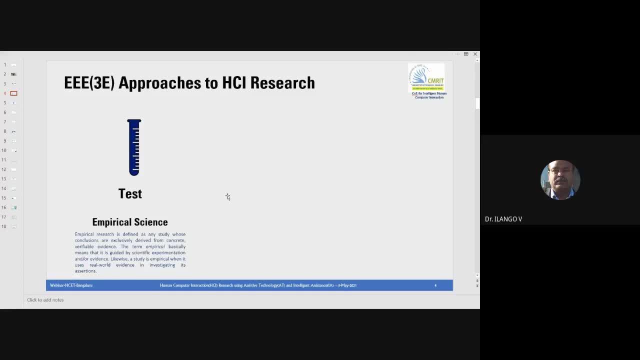 testing instrument. if you go pulmonar pulmonologist they will ask you to blow with instrument if the blowing pressure will be captured in the screen. so there is a computer interaction, human computer interaction. the report will be displayed right when come back to ct scan. here also there is a reading meter, reading everything: pulse rate. 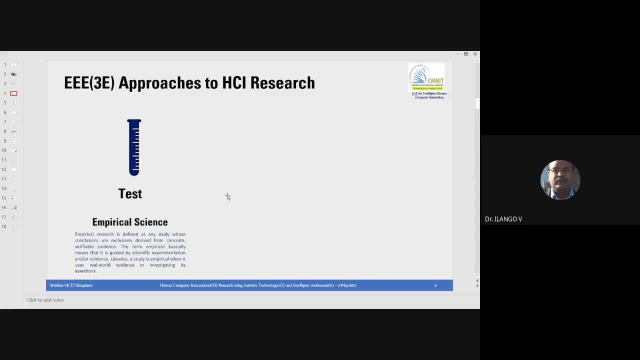 like that, only even blood test. also, there is a computerized screen, there is a data will be displayed about your blood. this is tissues and cells everywhere. this has been automated, customized computer computer software invented for human being, human being interacting. finally, report is prepared by the pathologist given to concern people. so this is a very 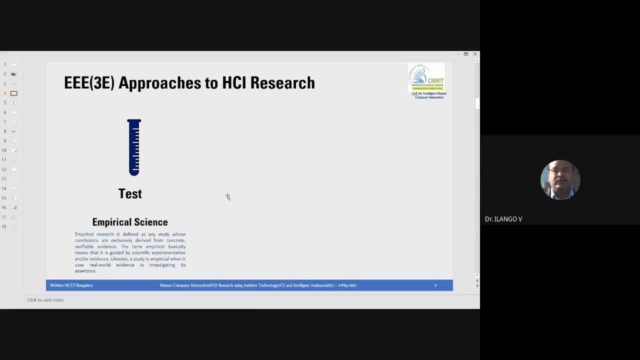 interesting thing is when come back to human computer interaction, no research will be accepted without concrete evidence, concrete proof. so we must do systematically- there are analytical approaches, the collecting right from beginning, collecting sample forming, the posting, everything. we must do that. but this is a interesting things- empirical science or empirical research, one of the 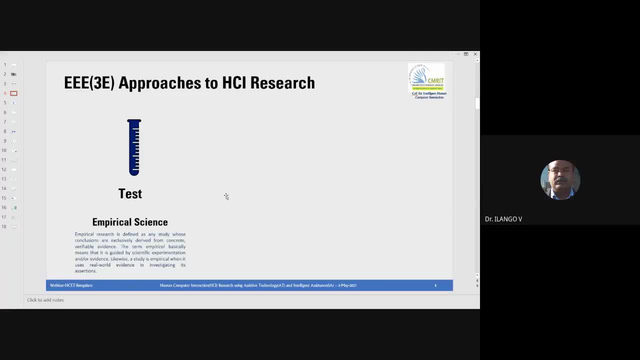 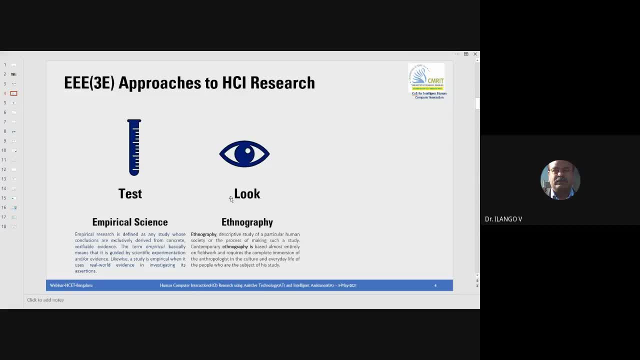 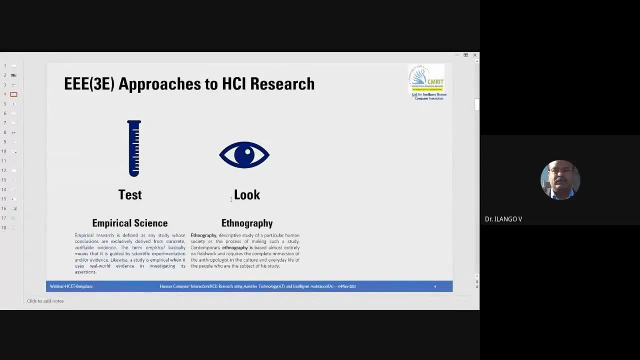 we need to go to field observation. if you say that tendulkar is play awesome, he's 500 ball 100 run. he's hit 50 balls, 70- then how they do, though. we observe video clippings when we go to the field and observe. 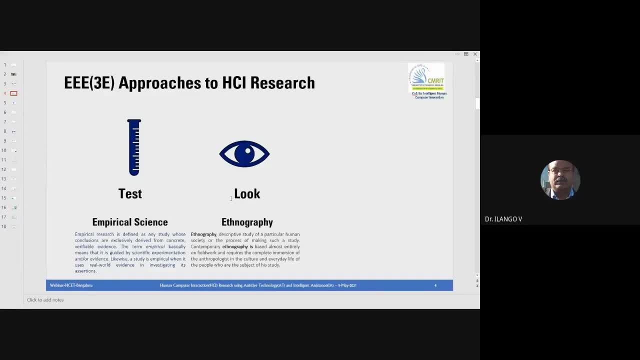 it. that field is different. that's why people go to auditorium. they observe. they are enjoying everything. it is, for example, like that: anything is there. the field study is very much important. it's an observation. ethnography is an observation. you are observing somebody doing work. what kind of? 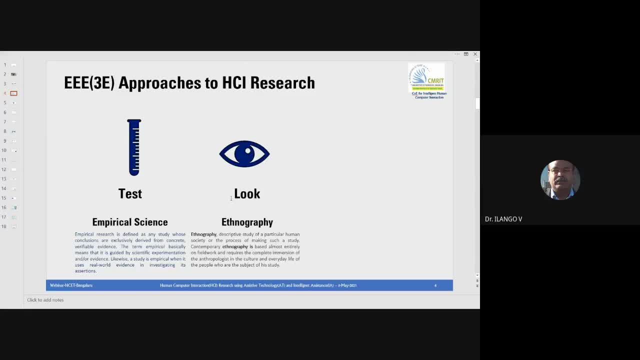 work they are doing. if people are making a dosa, how they make dosa. this is a way we need to make a dosa. you are registering, you have some pattern, you are coming back and you are trying how to make those the next day or immediately. also, so, through observation, quickly learn self-learning, then coming. 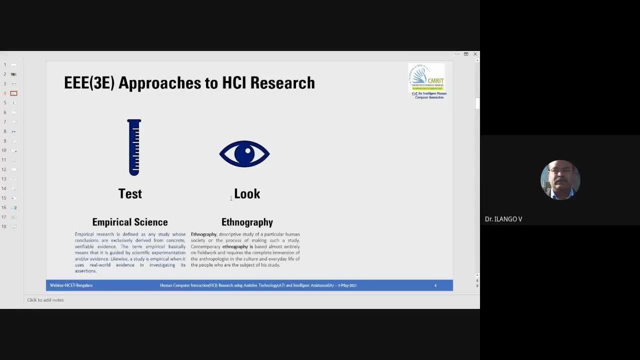 to practice that. so this is one interesting thing. ethnographic approach is a very powerful approach. and come back to human computer interaction. most of the human computer interactions research will be done by ethnographic observation. so if you can't say i have idea, i am going to do some invention. but 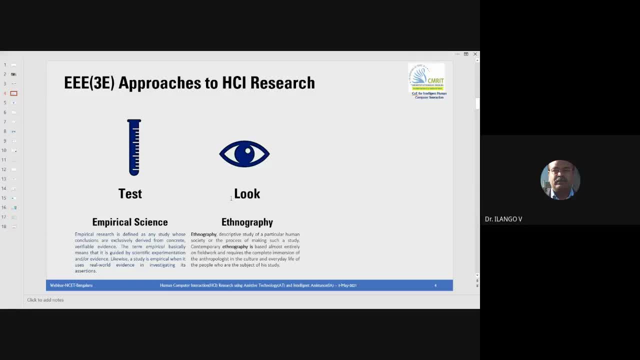 think critically this idea: for which community? for whom i am going to do the research? it is for me or my society? i mean to say community means it's for farmer or it is not farmer, it is for street vendor. it is not for street vendor, it is for electrician. no, it is not for electrician. 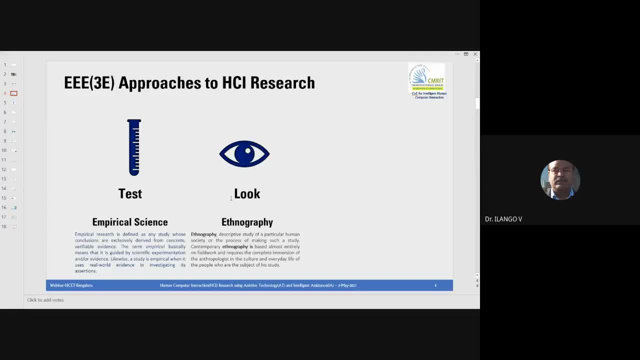 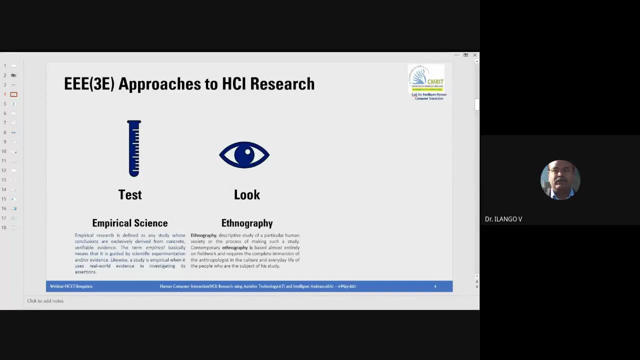 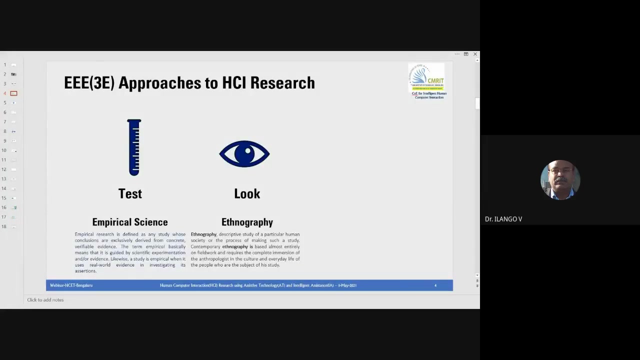 it is for drainage workers. no, it is not for drainage work, it is for, uh, this one scientist who worked in atomic energy sector. so these are all the community people in this community people. so, uh, you, for this type of community, you have to think, you have to design. so you have to go to their field. how they do it when you go to. 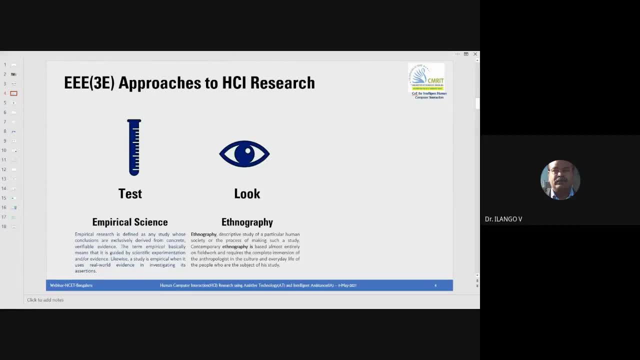 irrigation system, how they have to irrigation system. you observe that so complex. oh, why don't we solve their problem? this much time they are taking this much water they are wasting. to optimize water saving also, as well as energy savings also, let us use iot mechanism. so after 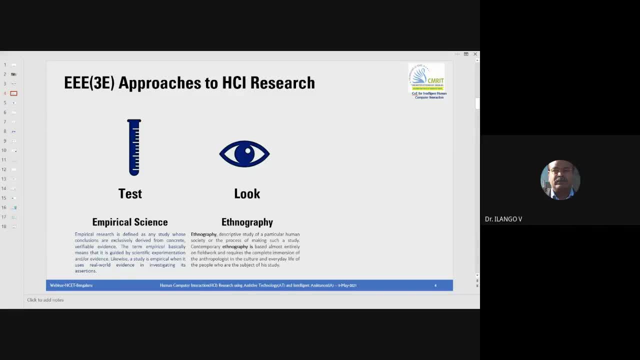 observing in the field. you are coming back and you are thinking of designing something like that everywhere it's happening. but again, you are a human being, you are observing another human being, community, so respective community. you are providing solutions for the community. you have the empathy on a community. for that community you are going to provide solution. so ethnography. 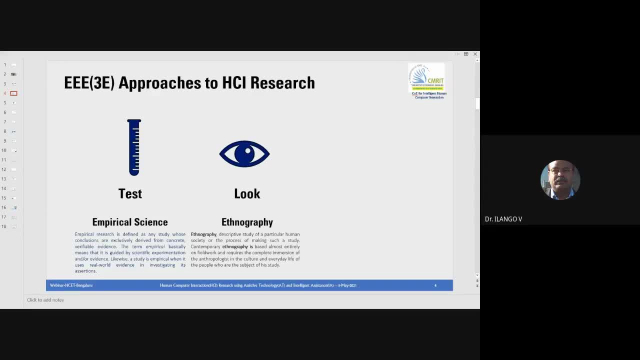 coming into that way, the pictures. if can carry forward that empirical also ethnographic and empirical together, you can move forward. it will be wonderful. uh, result also right. so another important third is engineering and design. so you have to make it right. you observe it fine. when you got idea this is a through iot, you provide. 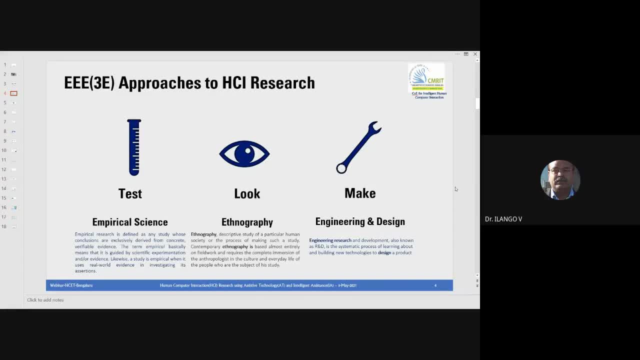 the solution, or image processing, whatever it is. you can collect the samples, data collections, all things, either qualitatively or quantitatively, whatever you like to do do it, but ultimately you need to have end product. how do we make end product? so engineering should come into picture. 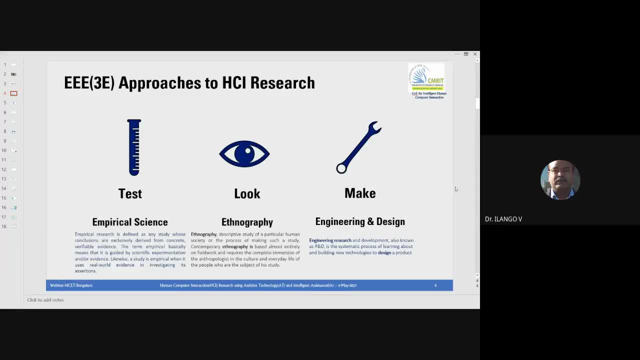 engineering research, which it is a systematic approach of making a product design. you can't just like that make a product and which is not usable, which is not useful. also, just like that, if you come in the market you give to them. who will buy? that cost also matter who will use it. 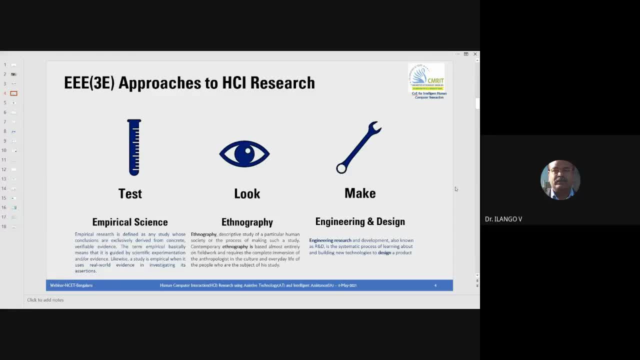 so it is very difficult to do that now we are having the smartphone. yeah, right now carrying phone. it is very difficult now we can't keep it in the packet. here and there there is dangerous factor. but it is excellent devices costly, also our telephone. so it is very handy, you can keep it in. 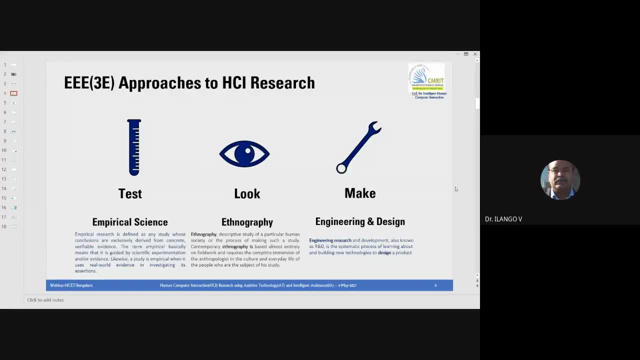 the packet. earlier, button system came mobile- very, very handy. anybody can carry forward button system mobile. it was useful texting various excellent device. now touch screen came. there are various sizes. that it's okay. it depends the people how they are capable of using the device based on that. 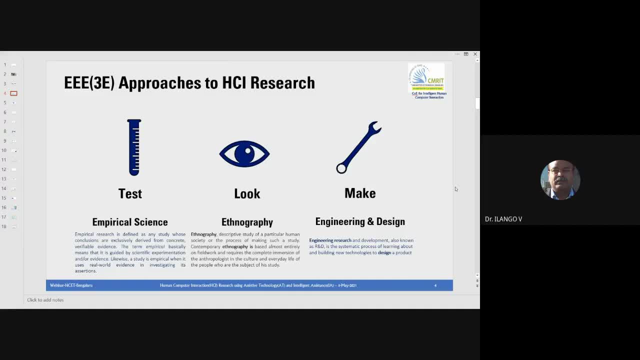 now. so mechanic operation will become very easy. but maintaining the touch screen, holding the touch screen carry forward, is a little risky experience. people are doing successfully right. so engineering design is important. systematic approach. this is a very meticulous way. we need to follow systematic approach. if you are making electronics as a product, you need to follow electronics. 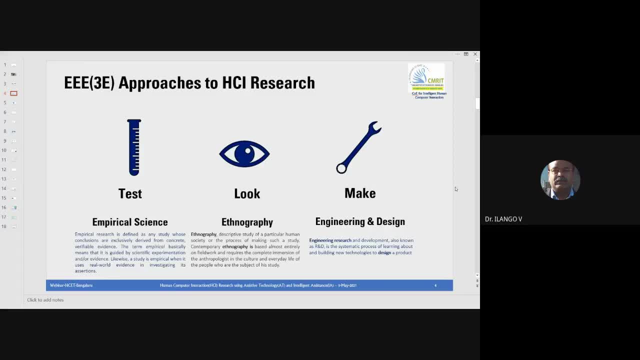 community, community engineering system, how this approach is available. mechanical device: mechanical device: there are some approaches. electric, electrical device: there are some approaches. so you have to follow computing science, there are some approaches like that. every engineering discipline, there are certain approaches. the approach can be amalgamated, put. 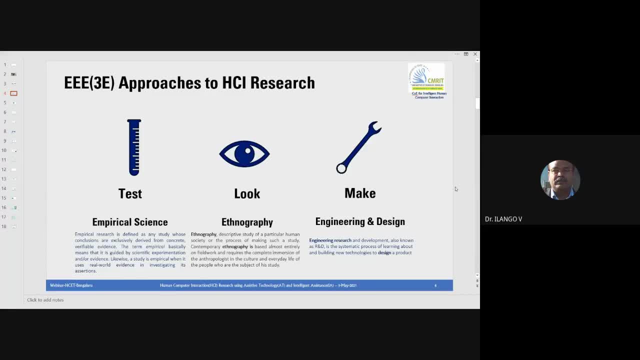 together and formulate a methodology to design a product which you are thought, which you created, which you invented, so you can go ahead. so that is very important things. it's a challenging engineering technology, wonderful mechanism, present scenario. this is very much secure. according to government of india, making india scheme is there in the scheme. so many innovations are motivating for. 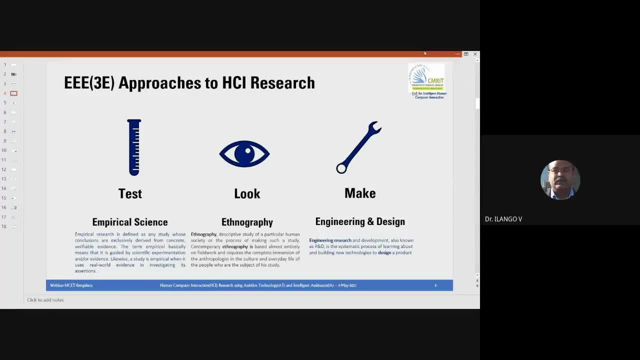 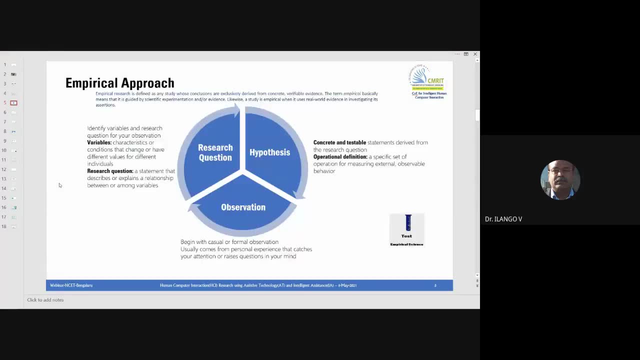 engineering students, engineering community, so you can come forward for various society requirement. right, these are three approaches. i just glimpse- this is in detail how the each approaches can carry forward. so when you talk about empirical research, the empirical research, as i said, told you, observe it. after observing you get some spark. why, what, how, like that you will get the questions in. 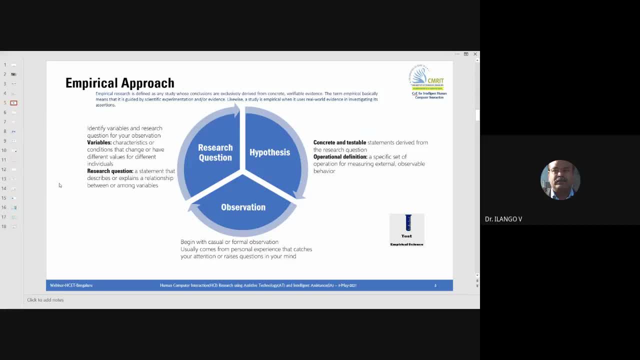 your mind after getting these questions, you are thinking carefully. you need some variable. the moment you observe everything, you cannot do it. so even for covet testing, you for you are finding some new devices. what could be the variables here? each sample, they take saliva. if they take uh mucus. 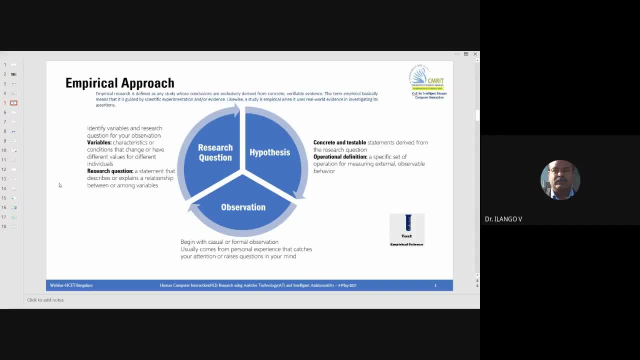 whatever it is, a bladder or any uh from the liver, this could be the variable. so you pick some variable: primary variable, multivariable, or see the univariable. one variable itself enough to test it, to confirm for it or not. no multiple variables required. multivariate experts: a multi variable is required, as a multivariate at least. 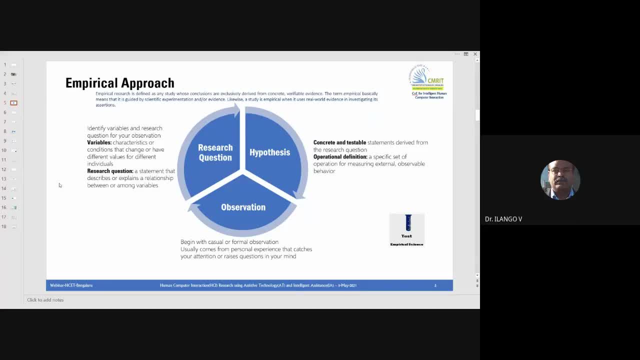 six variables, collect six variable, confirm the six variable. there is a variation or there is no variation, then you declare it as asymptomatic or symptomatic. so this is a the variable to be chosen: dependent variable, independent variable. so earlier also, even three years, five years before also, if anybody has cold cough, body pain, you go to doctor. they say it's a viral fever. 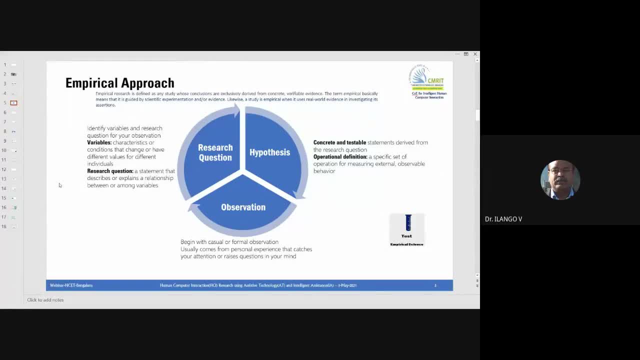 they'll use some three days in the course or two days code, it will be all right. the same symptoms available in during this pandemic also, people are scared suddenly obviously level down 90, 94, go betting, find the bet like that, so many casks are available. why this chaos happening? 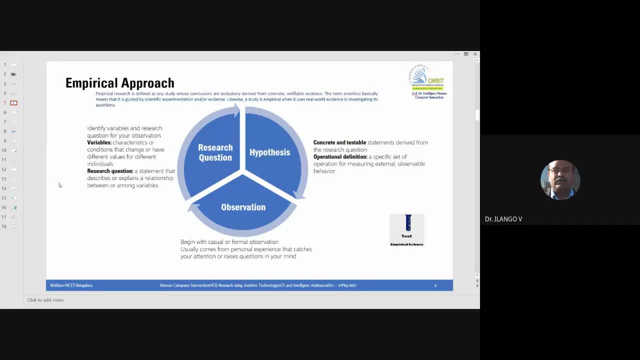 that means your systems are not constructive system, so we are not able to prescribe a proper diagnostic mechanism. it's the biggest challenge. is it that the question arise to you? we do not have proper diagnosis system. is it that? or we are not having constructive way of forming, concluding the result with the proper sampling, do we not have? 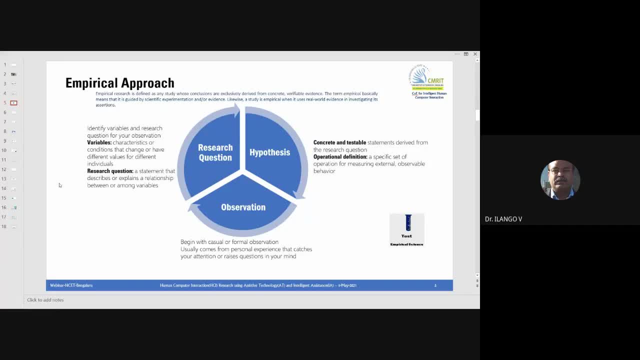 proper interface system, software system or hardware system? what is the way to do that test? so 42 hours they are doing it. is there lesson in the particular, anything else to be done? whether the result will be accurate? so these are all the questions arise in the picture. so you need 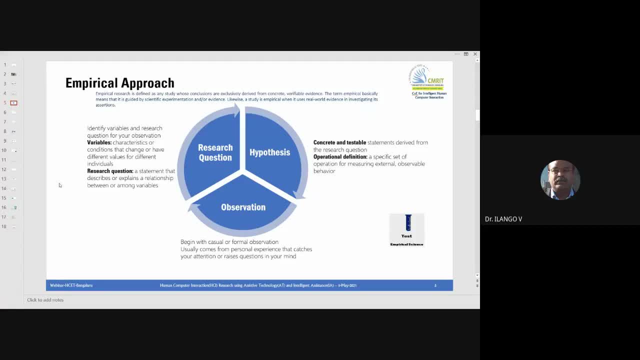 to form the hypothesis. so the moment you observe you cannot say that people come, they are having the code. what can you decide? this person has come back. form the question, go analyze it, then fix some hypothesis. he went, he might have traveled somewhere or he might have touched somewhere. i might met some. 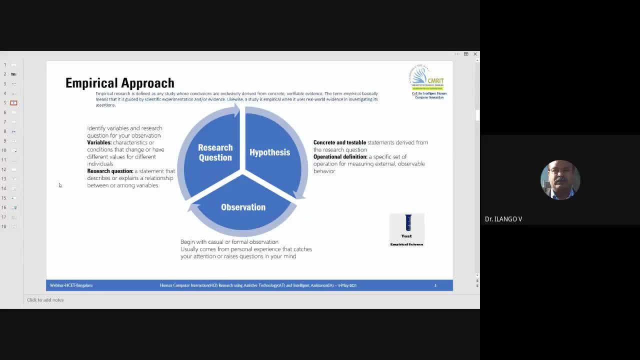 patient. our hypothesis one, hypothesis two, hypothesis three: no, this is not there. this is not there. this is not there, then which one will be there? patient family has got affected. that's why it's came. no, then, what else you mean from: colleagues are traveling. he was traveling. 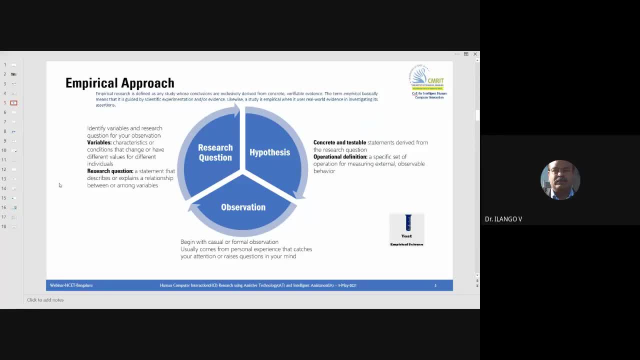 with public transport. from there it might have come. or he went to grocery shops from there it might have come. these are all the hypotheses, but still now, what is the exact one? we do not know. it's an assumption, hypothesis based on some assumption. you form it, you, one by one, you are. 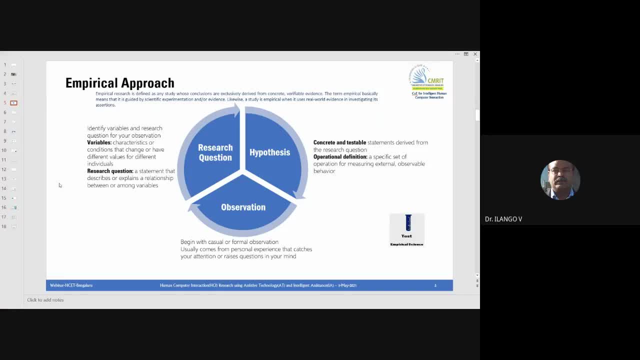 verifying that. so, one by one, you are verifying. this could be, this could be, this could be. finally, what was that? what was the reason? yes, we found the reason. he took a patient who got affected, positive, positive, took admitted in the hospital. he drive in his car only to emergency. 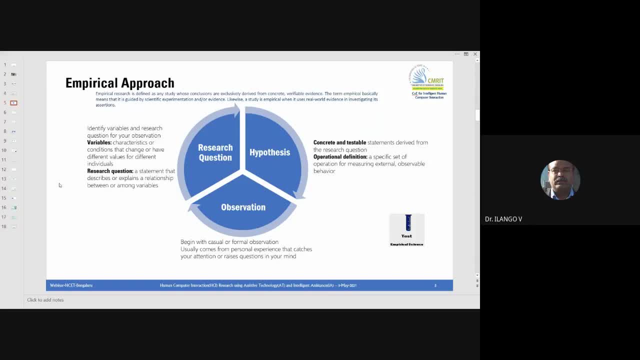 while traveling two hours journey, the virus are something is not affected for this person. this is what the true. oh, okay then, so operationally, you are concluding with the observations. so, empirical research: your big challenge is quantitative approach, qualitative approach. is there one quantitative approach based on the 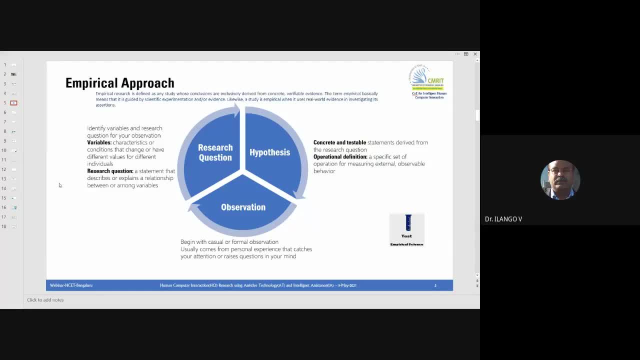 numerical statistics. numbering based on the numbering system. qualitative approaches based on the verbal verbal approaches, so forming the verbal yes or no, like that. there are certain norms based on certain norms. you are going for analysis. both are very important and come back to the empirical research. but qualitative research is more tougher than quantitative research, so you 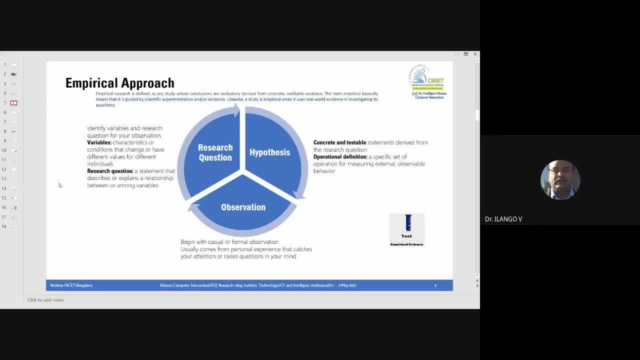 can have thousands of record, one lakh record with a numerical number. easily you can analyze a field model, simulated model or deep learning model. same model only if you have ethnographic observation. go to field and ask: are you using irrigation, irrigation or spray irrigation? they say spray, yes, no, like that. you will take statistics. you 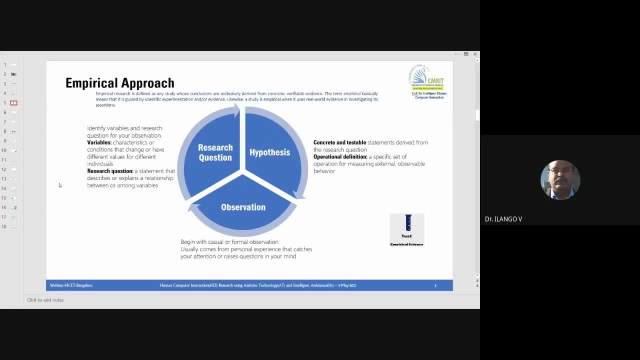 come back to lab, how you will analyze that. either you have to convert the qualitative data into quantitative data or you should go as it is: the qualitative data. it is little complicated but it is superbly doing us and today, for which you know they have done excellent research with. 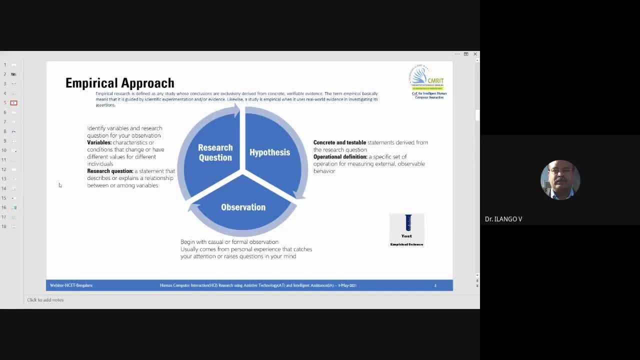 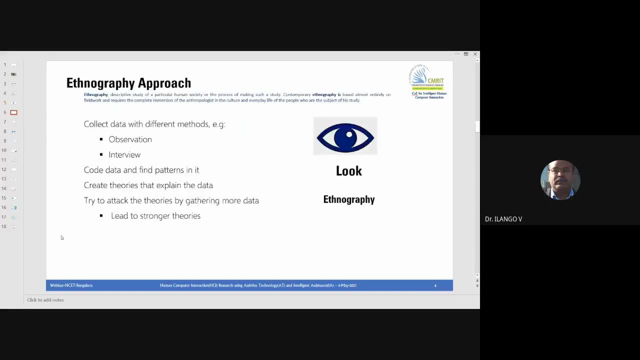 empirical approach, uh, qualitative approaches. new model has come, various tools have come right. so this is the interesting way: the american research and computer interaction, people observing. the second interesting thing: i told that ethnography, in the field, anthropologists, there are people study about certain community, uh, community communities who say people living 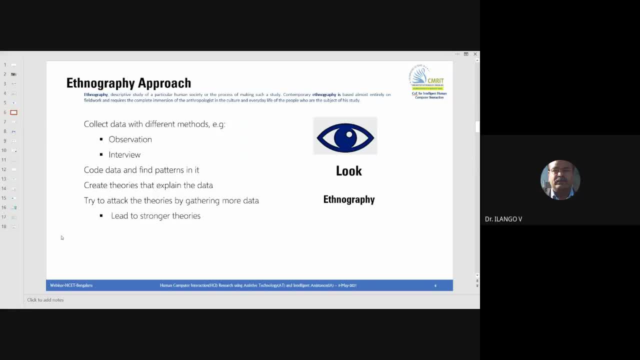 in the society. their requirement. tribal is there, the tribal also. different type of tribals are there in india itself, maybe 20, 30 types of island. there are some different tribals are there in entrepreneurship tribal in karnataka, some tribals like that in northeastern nagaland. 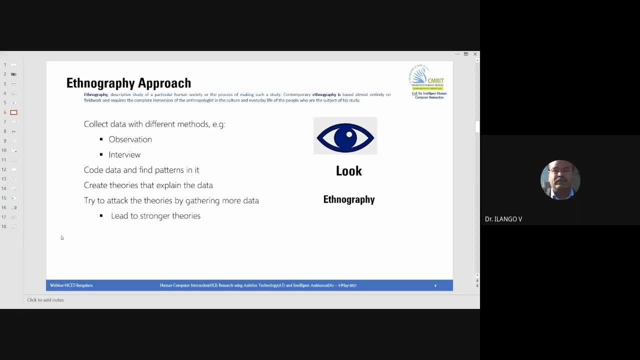 kalaga. there are some tribals. each one has a different type of living style, so what would be their requirement for them to support the technologies, for example? i am saying that so this is what i studied. very contemporarily, we studied in the field. anthropologists mean people who study about people, society. you can take their support, their support and build. 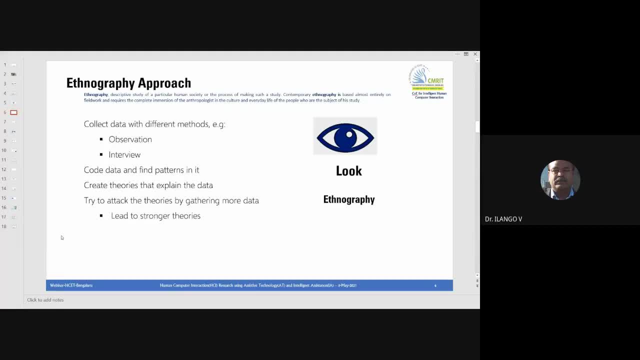 so collect data with the different methods. uh, when you go to observe the field- observation, then interview- you can talk to people as i told. irrigation, drip irrigation or spray irrigation, yes or no, it's an interview, personal interview or online interview. you can collect and collect survey questions also various observation and code. 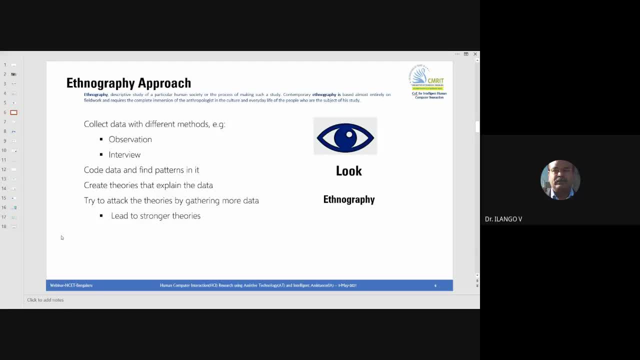 the data on pine pattern, feed into the system, build some pattern from the data after that, so create theories. there are so many theories. ethnographic theory, anthropologist theories are there. you can call, for example, let me say, the ranch kota theory. it is a mathematical theory. 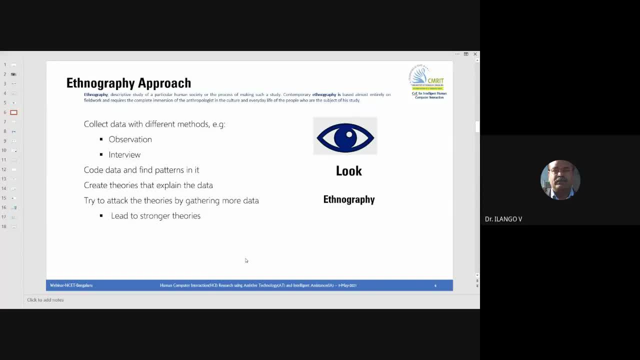 and simulation. there are many theories- uh, we can have any kind of theorem. mutants- uh, law is there you can use. these are all the things it's feasible to use. what is their contribution? okay, we'll map with the conclusions like that, try to attack the theory by gathering more data, so minimum data may not be feasible. to conclude, 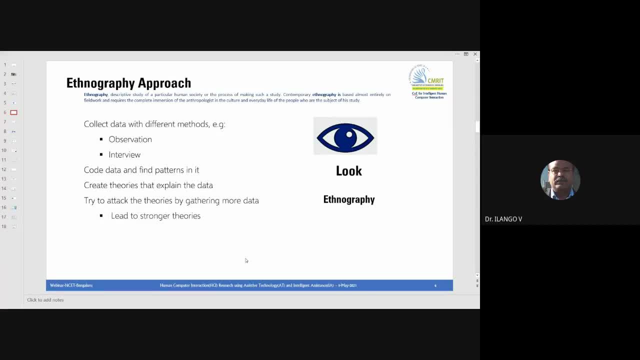 you can go for large data, multivariate data, to conclude that your research lead to strong theory. so you can also form your own theories during this ethnographic observation. so most of the time when they are not validated, and later they are not very good, so that's why they are very difficult to 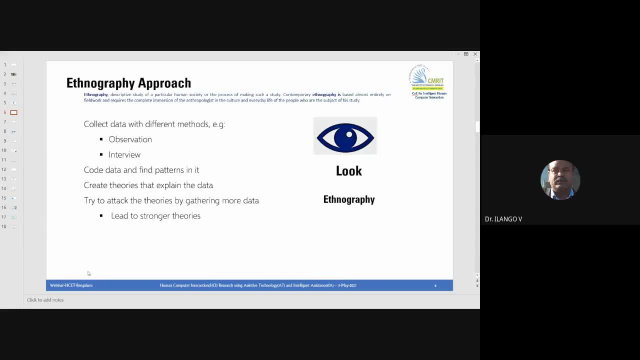 do uh to they. problem is when, if they are not there? if they are not there, how are they going to solve their problem? so it's very difficult to verify the reality of the problem. so, first of all, is this theory that this is a very analog format. this is a very long-term theory. in fact, it is a very 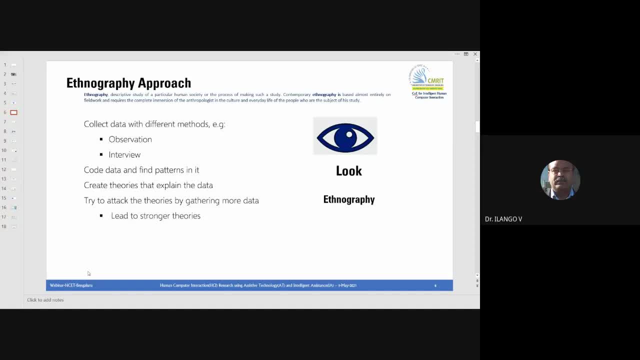 long-term theory, but it is a very long term theory and we are using a lot of different theories as a 40 years old. as we are supposed to do this, this message wrongly typed or it goes to somewhere. what to do that? So these are all the theories available. 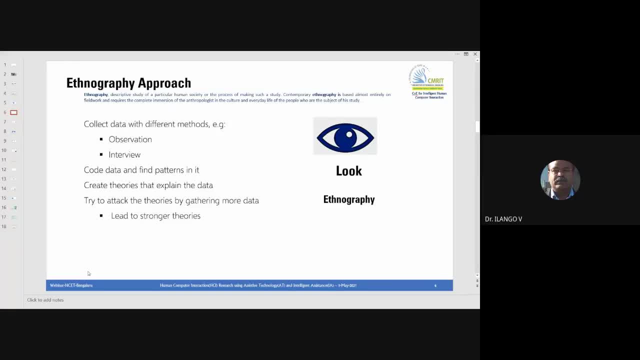 So today when we type SMS or WhatsApp message by mistake we may put male, man, female, like that we miss some messages. it will become wrong meaning. It may be giving the wrong meaning. So this is the problem. So you can say: are you coming to college today? 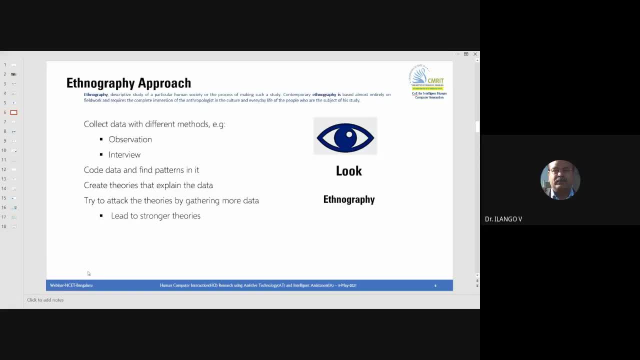 This is a normally colloquial statement When other end read: friends to friends is okay. peer to peer. If I send to student, it's okay. If student send me the same message to me, are you coming to college today? 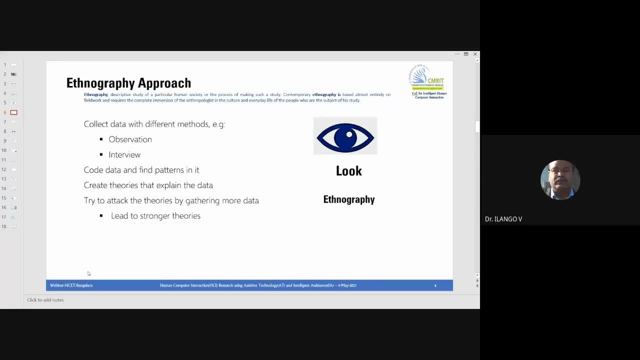 I will really get irritated. What is this? There is no respect for me. At least you should say, sir, hello, are you coming to college? So this is the way the misinterpretations are there. The age group, So ethnographic observations, will optimize all these type of things. 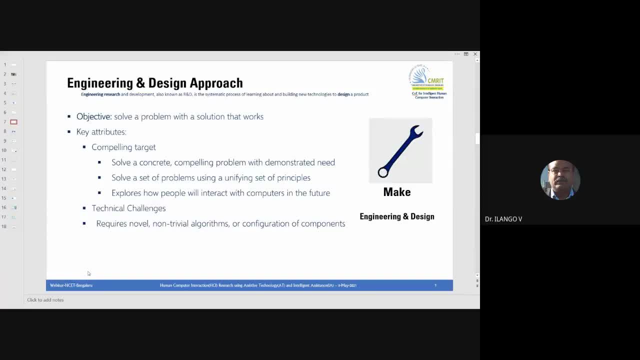 Very interesting research. Finally, last E, Engineering and design approach. We need to have some objectives, even go for engineering and design. solve the problem with the solutions that work. I told that you are doing for agriculture field farmer, for what you are making: the product design. 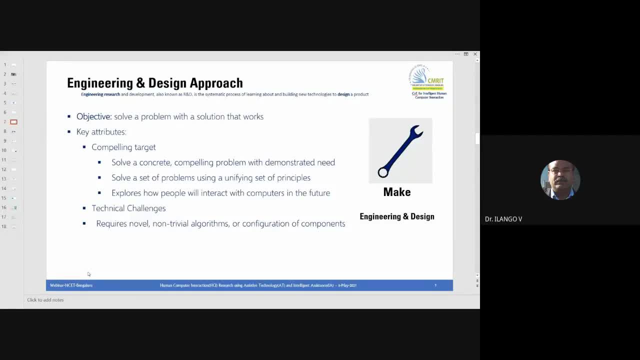 It is for only irrigation purpose or farming purpose or fertilizer, like that. You should have very specific objectives. Then you have to go Key attribute. you should be having compelling target: solve a concrete, compelling problem with a demonstrator needed. solve a set of problem using a unifying set of principles. 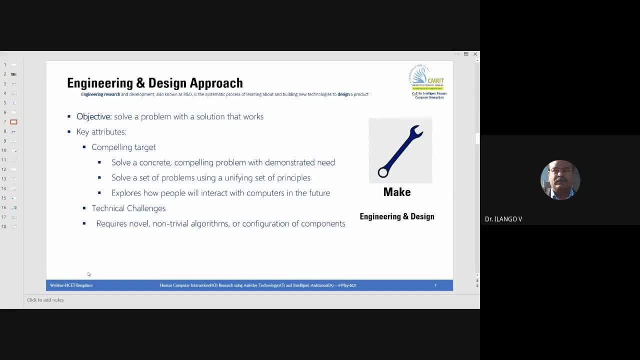 You should. you will be having the principles. Without that you will not enter into the field. explore how people will interact with the computer in future. Say 20 years before in Indian agriculture system the computer was not much use of that. 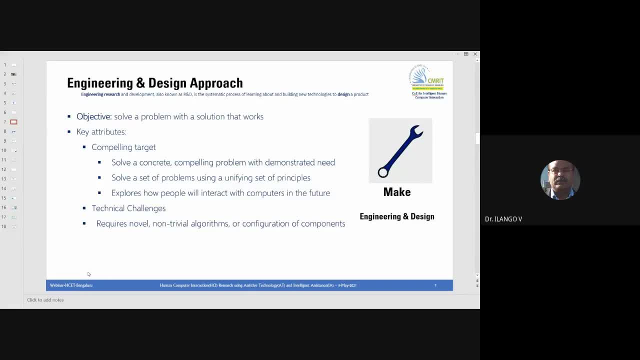 But today a computer is effectively used more places for from home itself. You can switch on your motor from your. your field is the 10 kilometer far your agricultural land. you are at home. you can operate automatically the motor pump. 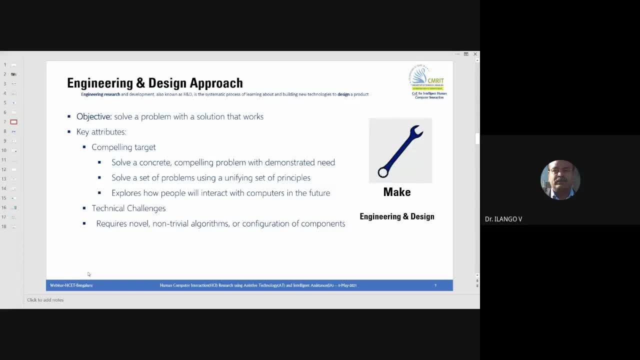 It will go and spray water. everything is there three hours, two hours. then you can automatically off. that you can monitor. So it is one way, efficient and effective. and drone: recently drone has come to market to spray fertilizers or observe that the stealing ability or controlling security purpose. 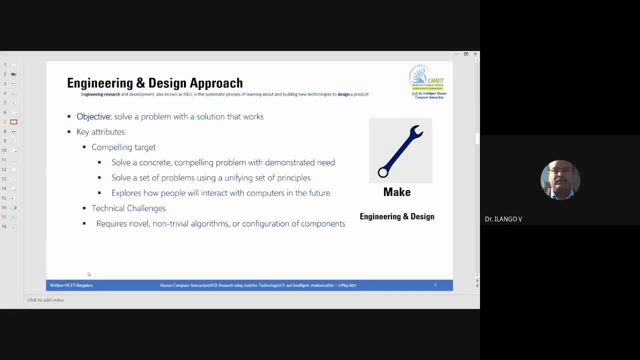 There's drone, mechanisms are using that, but these are not there. Recent Here, 21st century, the chairman, people accepted, even people want more than the 20th century. mindset is changing. So though however that mechanism come, technological challenges are huge. the drone, how many? 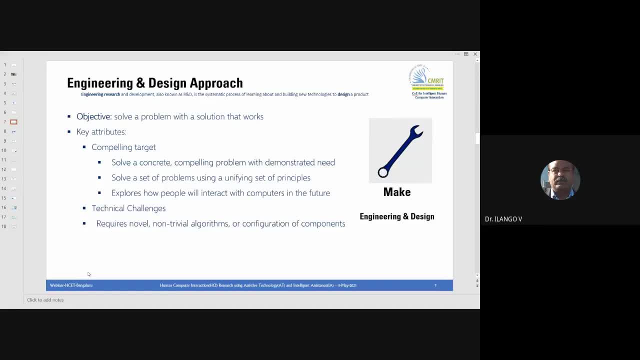 people are able to operate it. who can operate it on agricultural farmers? a landlord? he cannot keep a drone operating systems in his home, He has to outsource into some company. you can only give fertilizer but machine will come by somebody out third party will operate it. 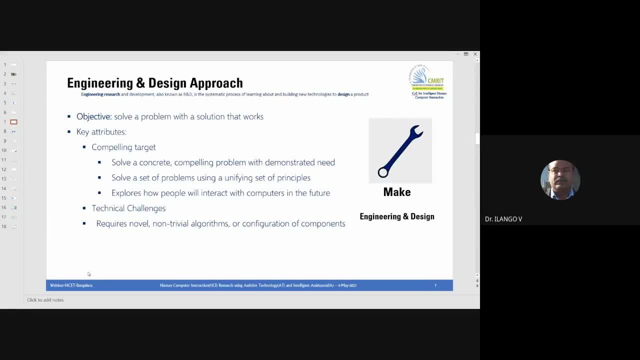 Many other tasks are there. fraud will happen, cheatings will happen. So these are all the things to be addressed very carefully. technology comes, but how optimistically the technology or people are educated properly to operate the technology. They have self learning mechanism. they are able to handle sustainably themselves without 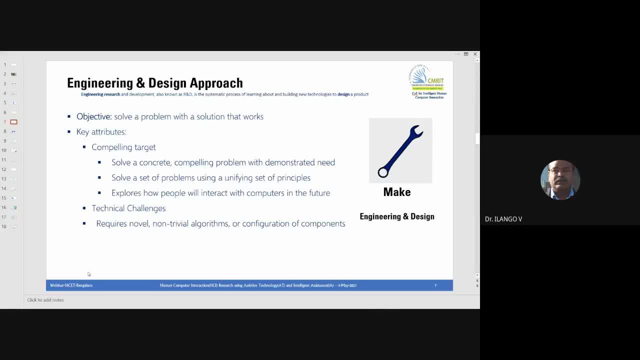 any problem then it is good, This is coming, this kind of mission activity maybe another 10 years, 15 years, everything will be literated, educated about technology usage. So require novel non-trivial algorithm or configurations component. 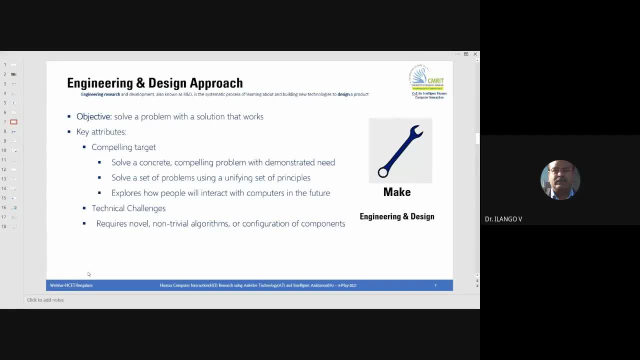 Yes, obviously computer science. when you go for hardware optimization, you need to have interesting mechanism. Who knows that? CPU was there. central processing, now GPU have come, graphical processing, TPU also available. What and all going to come? we don't know. so voluminous data comes. people started nowadays. 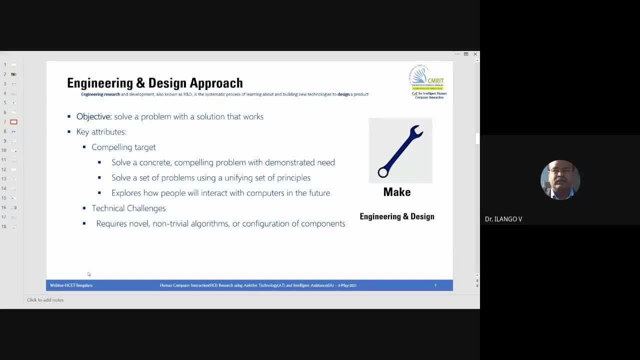 maximum. people started to use GPU, N-media GPU like that. They have come up with some graphics card for animations, multimedia gaming purpose Beyond that also is there. So now cloud is providing GPU systems like that. algorithms are there, coming, it's unlimited. 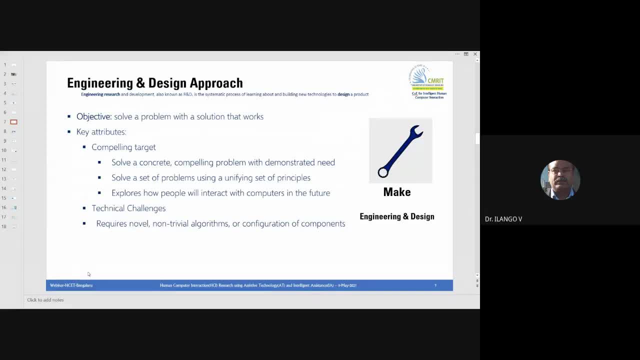 we need to think very broadly. as engineering graduate, we should learn many things other domain. we have to implement it into our domain. So this is a 3E I recollected. So this is a 3E I recollected. 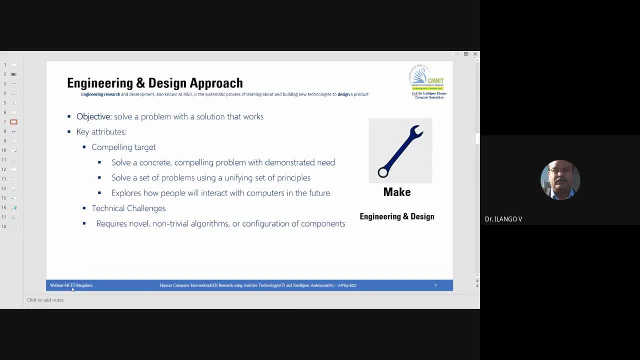 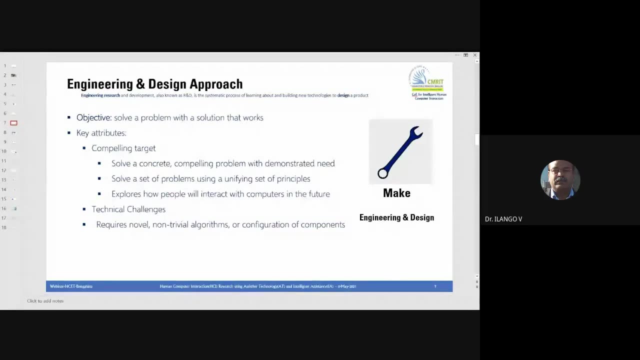 So this is a 3E, I recollected. Can anyone say what are the three approaches for human-computer interactions? Can anyone answer to me? Can I get your attention? please Excuse me? Yes, sir, please, sir. 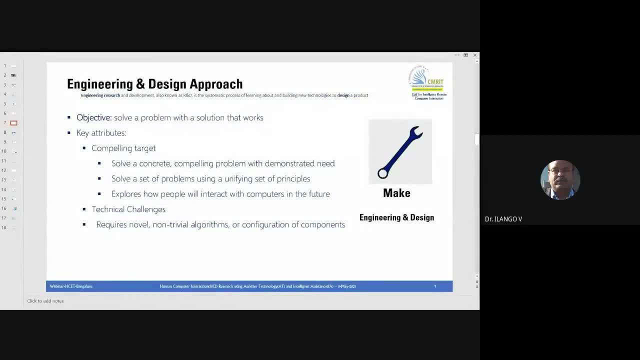 Can anyone answer student side? what are the three approaches? human-computer interaction approaches? we discussed last 10 minutes, 15 minutes. anyone can summarize What are the three approaches? I'll repeat the question, Hello, Hello, can you hear me? 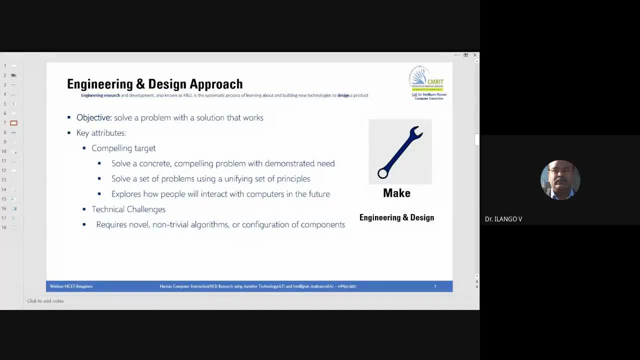 Yes, sir, Yes sir, Students, Students, any student, please answer. I'll repeat the question we have discussed last 10, 15 minutes: three approaches of human-computer interaction. What are the three approaches? Can you hear me? 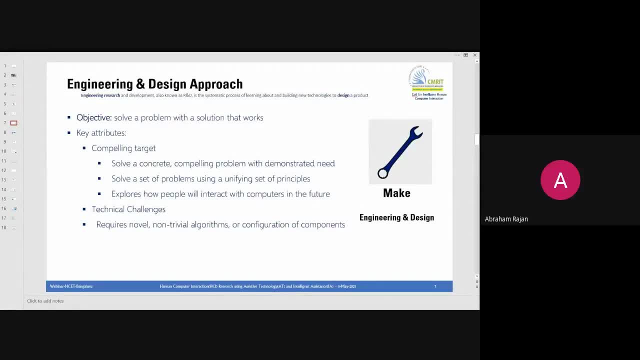 Yes sir, Yes sir, Can you hear me? Yes sir, Can you hear me? Please answer, OK, Can you hear me? Yes, sir, Can you hear me? Yes, sir, Can you hear me? Yes sir, Already one approach is there in the screen, So you need to think up two more approaches. 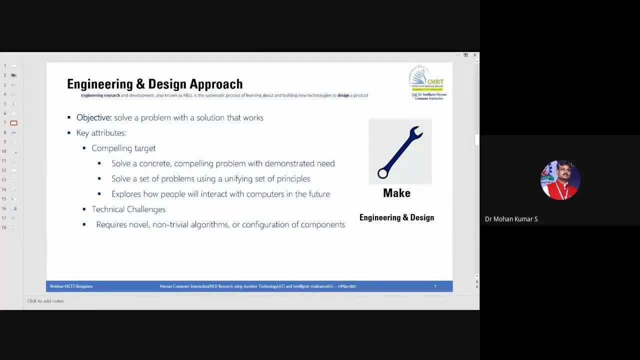 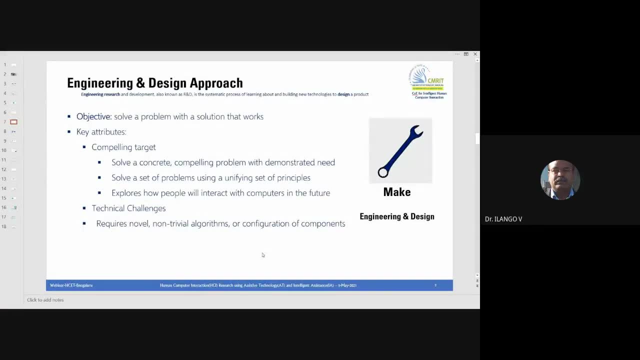 Empirical and engineering design approach. is there One more? I gave tips. Students should tell That student will be declared as a good student or top thinking or critical thinking students like that. What about cognitive approach? All are cognitive thinking only. Everything is integrated with cognitive only. 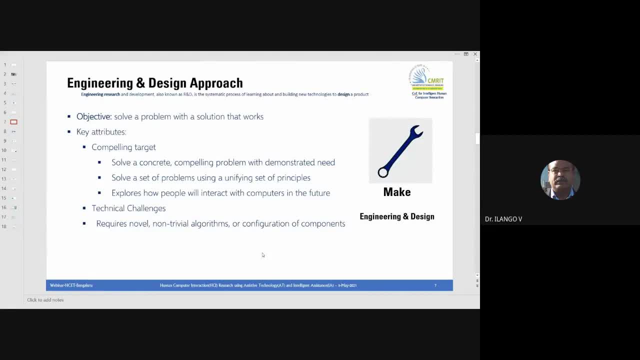 Exclusively human computer interaction research. If you are going to do research, it cannot be done by one individual. It has to be done by a group of experts. So one expert will be expert in one area, Another expert will be expert in another area. 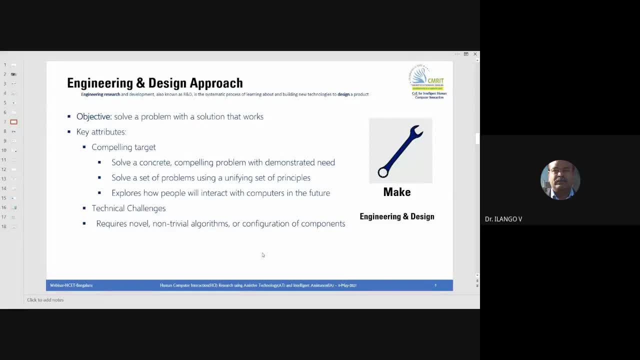 Like that only Since you are engineering student. you are studying computer science, engineering and information science engineering, So you will be able to write. You will be able to write algorithms, or designing and fabricating with Arduino or certain type of system called Android. 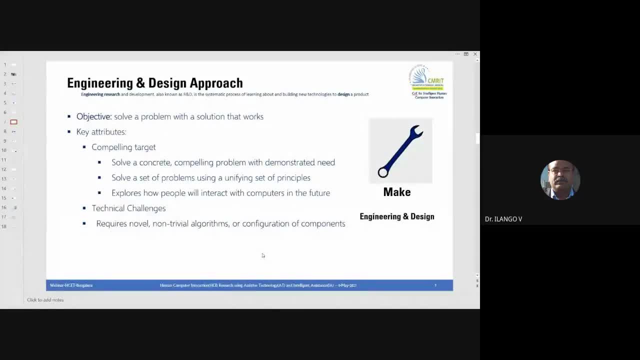 Like that, you will be able to fabricate it. So this is your expert area. Like that, another engineering Civil engineer comes. What they will do with coding system, Arduino and Android system? They may also do wonderful, We don't know. 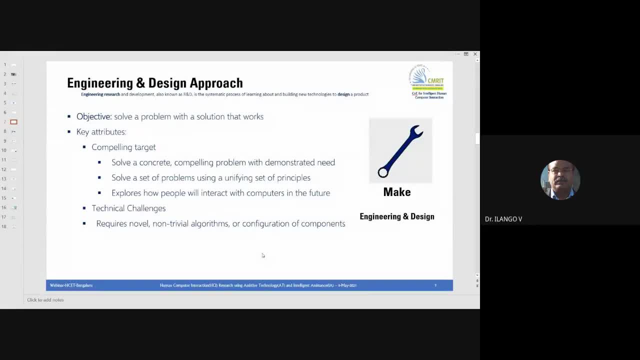 Mechanical engineering also may do wonderful, also Web tech, engineering. What they will do with Android and your coding system. Yes, They can come and ask you To write a genetic algorithm, How to optimize it, Like that many things. they may ask that. 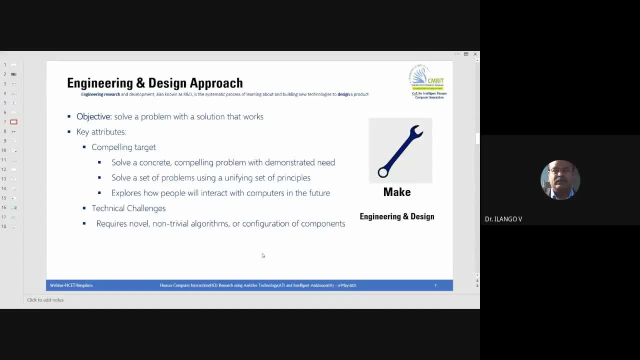 So what is that engineering? It is a very broad area. You are good in your domain, So you have to integrate with all other engineering discipline. You have to go for common designing For some group of society. Likewise, how do we go? We discuss, as professor said. 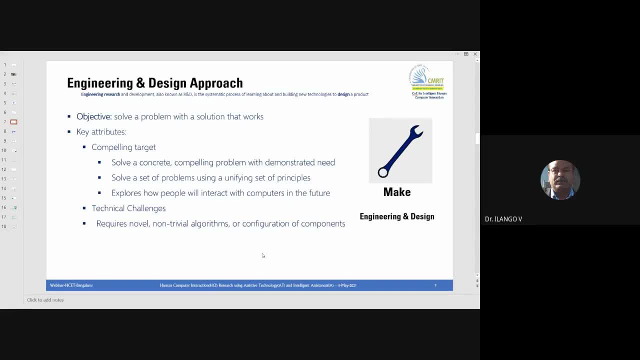 Ethnographic approach, Then empirical approach. The three E should work together. Only we can come with a constructive product which will be long lasting, Which will be accepted in the society. So this is very interesting thing. All of you remember that. 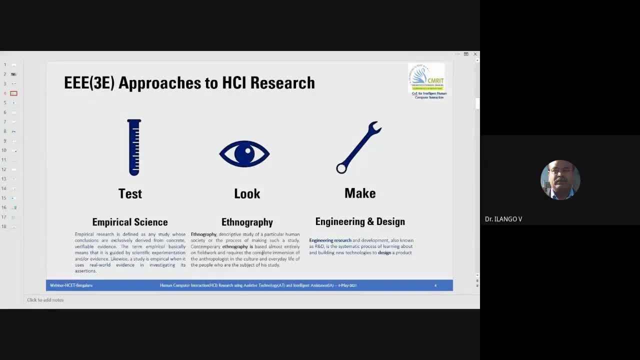 Human Compute Infrastructure. There are three E's there Only Symbiotical approach and Ethnographic approach and Engineering approach. Engineering, basically, people think in the market. those days, Till 2010, people were thinking about engineering: Designing: mechanical engineer, Automation engineer, Electrical engineer. 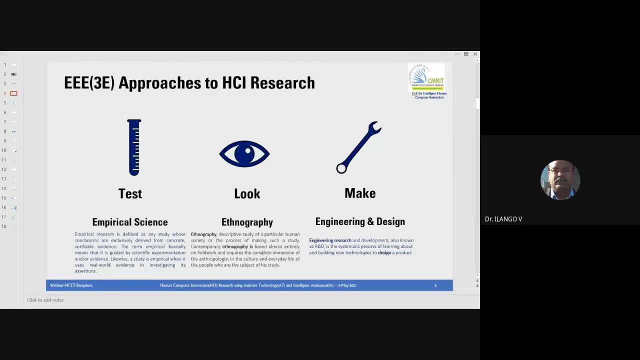 Electrical engineer has got lot of booms Later. sorry, 20th century, 20th century, only computing science engineer has got demand, Then other automations or mechanical engineering, Software engineers. This is what the scenario change now. Ultimately, software engineer also work in mechanical products. 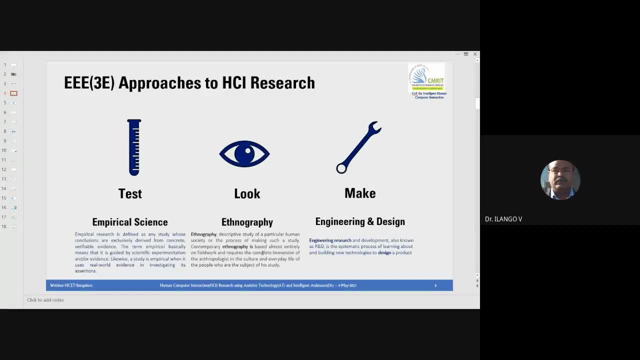 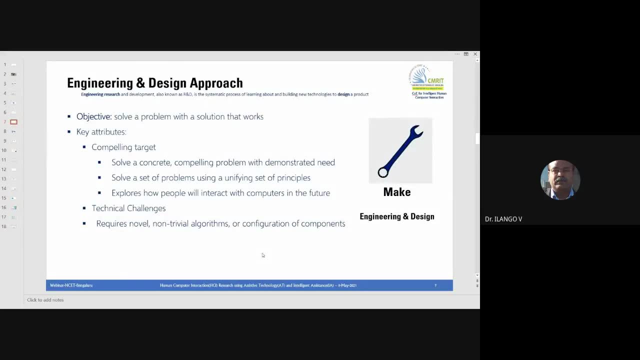 Mechanical engineer also work with coding and writing mechanism, So all are same. now, These are three approaches: Empirical, Ethnographic And Engineering. Okay, Now How do we go for the engineering design? This is another essence of that. 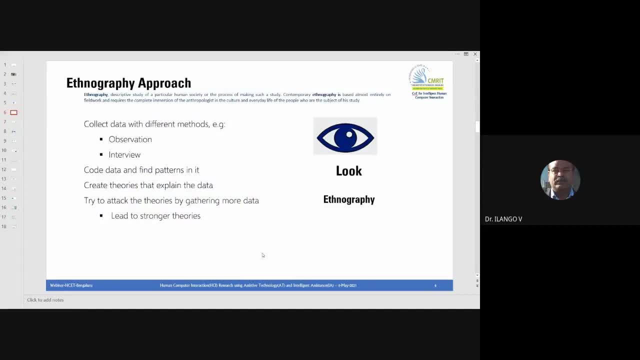 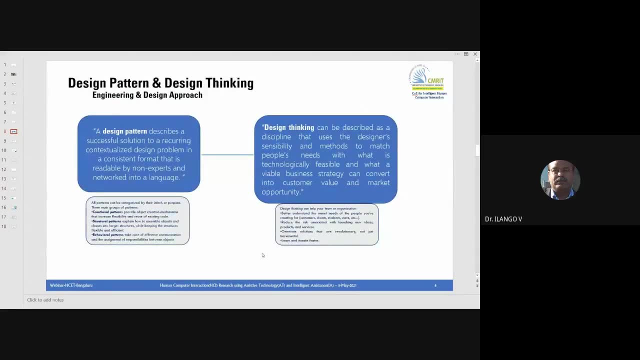 As we discussed, the group Three, group Two, group. We can make together. Individuals cannot do that. As a computer science engineer, if you are asked to make irrigation systems, Piping, Pumping, Automated power pump on and off in the field, 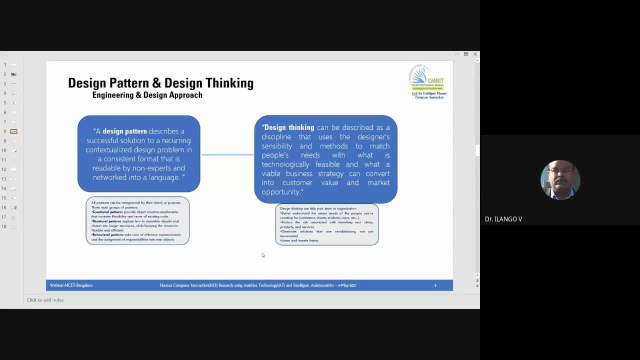 How you will do that. You cannot do yourself alone. So you have to go with BSc Agree, Mechanical Agree Or Agriculture Engineering somewhere, Or you have to meet farmers also. You have to observe it. Then only you have to come back. 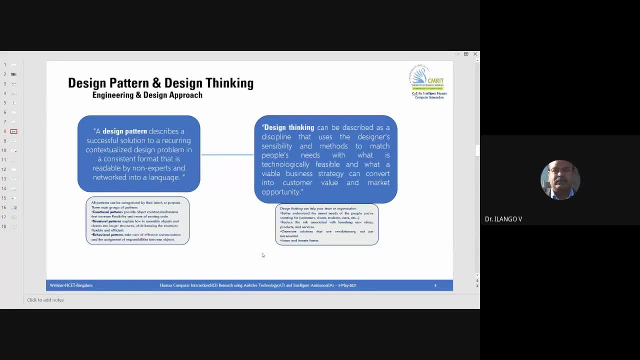 And design this automated pumping system. So, either using GPS or IOT, Without these two you cannot do it. Okay, When you go for GPS, you need to talk to electronics engineer, Signal processing. So after that you go for field implementations. You are going to pesticide control. 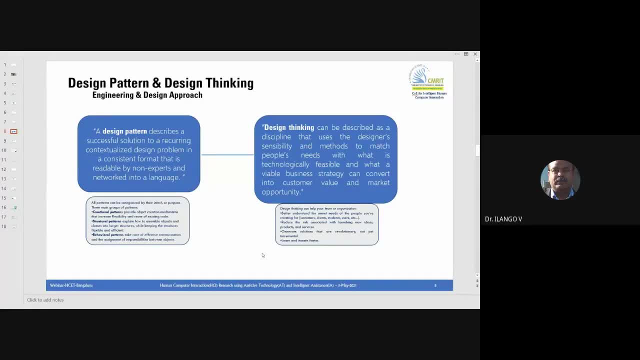 You need image processing. Obviously you need certain biological science students, Botany, who would learn better. So this is the integrated way. When you go for integrated way, Design pattern and design thinking is very important. So design pattern, Design thinking, Both are hard for engineering research. 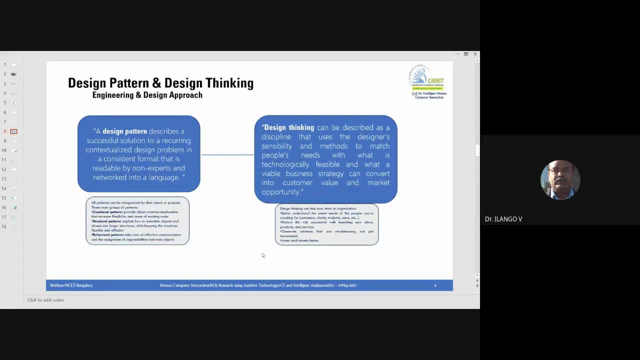 Engineering, design and research Very important. Both are two. I's Design pattern and design thinking is very important. Design pattern is nothing but Describe a successful solution to a recurring contextualized design problem In a consistent format. It is readable by non-expert and network in real languages. 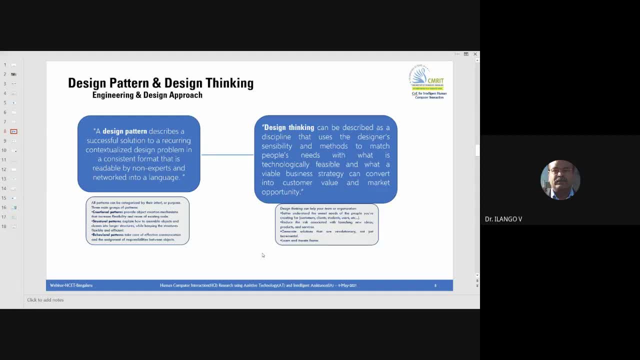 Very simple, The design pattern. Any illiterate people see your product. They like They should appreciate it. Take mobile phone Now everybody, even in the street Vendor, has mobile phone. Different type of mobile phone, Maybe backers also, Maybe they are. 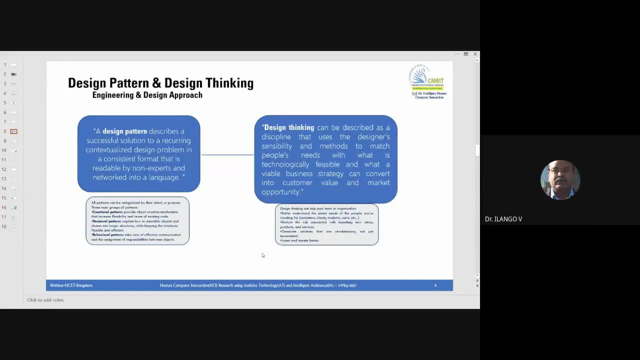 Maybe, having the mobile phone, They are able to operate it. High level people also operating their Apple iPhone. Low level people, Profile people also operating iPhone. 5 years child, who is not having any profile, operating iPhone. Even CEO also Microsoft Bill Gates also operating iPhone. 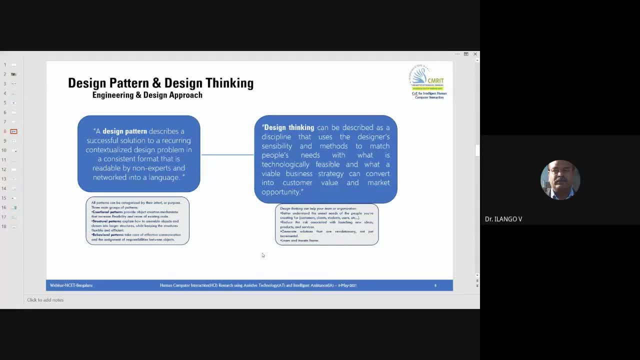 Both are operating efficiently, effectively, So that means That's why the design is being successful, Why Apple iPad is very successful: Everyone who is using Without having any background knowledge. So any design you do from illiterate perspective, They observe. 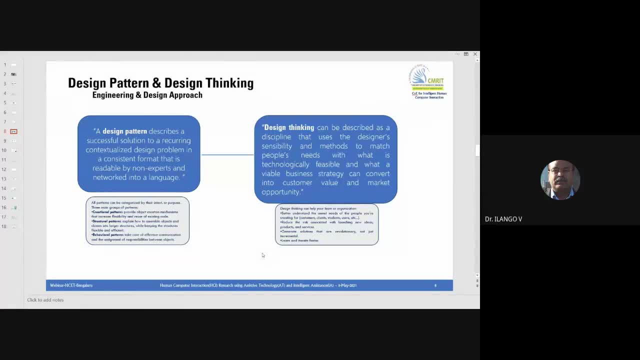 They should be happy, They should accept it And it is called successful design pattern. There are many ways Successful design pattern. You can have structural pattern, Behavioral pattern, Creational patterns, like that Three way of pattern approach is there In engineering side. 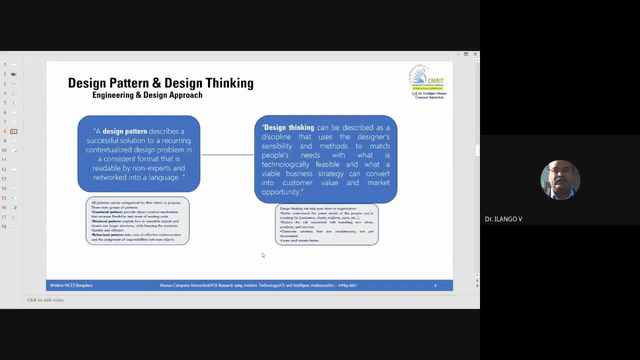 Computer science We used to study object oriented design and methods. We will study MVC controllers like that, So that subject has more depth ideas How to make use cases. also, We can learn from the design pattern. So that's it, Thank you. 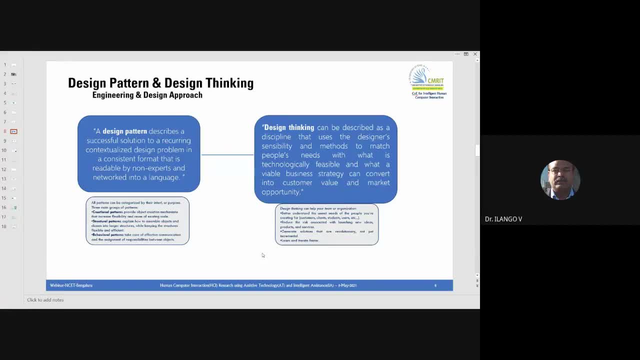 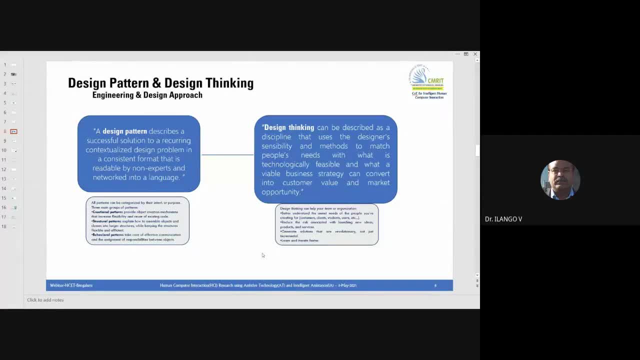 For the design pattern. This is one approach. Another approach: Design thinking. So when you think properly, only you can come back to the design. So without having thinking, you cannot come back to the design, The proper product. How do we have design thinking? 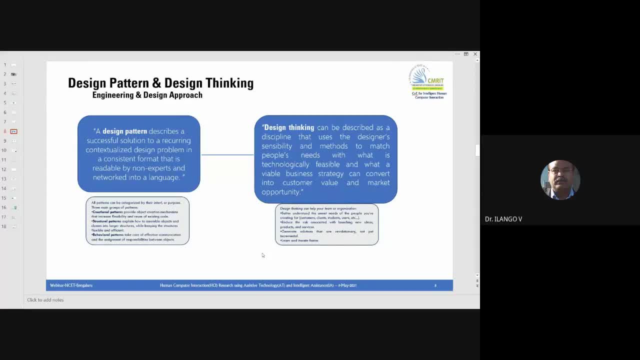 Design thinking is very interesting thing Described as a discipline that use the designer sensibility and method to match people needs. People needs- I stress this word- What is technologically feasible and what a viable business strategy can convert into customer value and market. 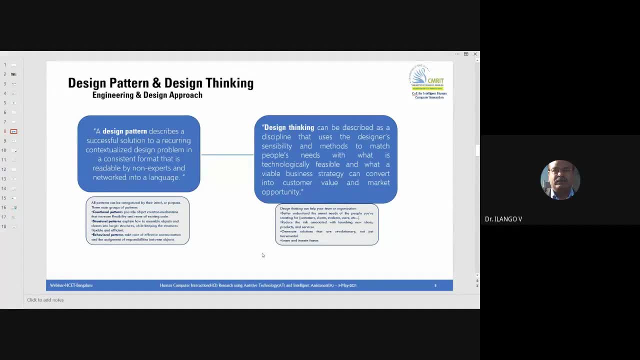 opportunity. so I told earlier, empathy is very important. you think about some community as we learn our ethnographic research, some community needs certain technological devices, then you have to go and observe what is required for that community. you are developing or designing the product, for example. again you come back. so now the grocery shops available, the street vendors for the 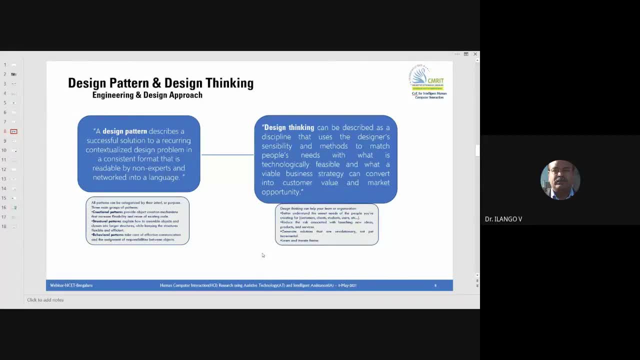 street vendor. they are having different type of transactional mechanism. those days we- maybe five years before- we used to give cash and they give the changes. now. even the street vendor have the Google pay, paytm and phone pay. these are all the one sticker they will have. 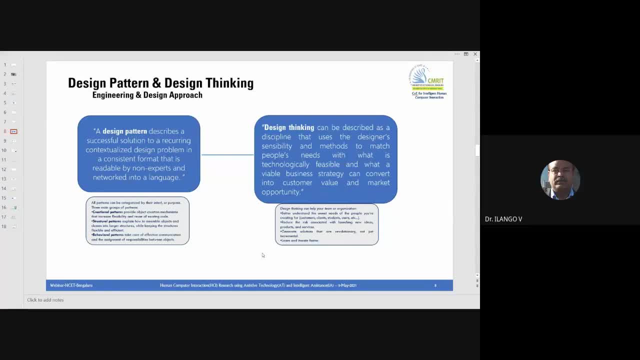 kept in the four-wheeler cycle. we will buy some banana or something will show the QR code. it will be taken money. you see to that. what is the standard of living four years before? so he has to have the chain and everything. now he does not have any change. even fine, everything is digital currency, is it? 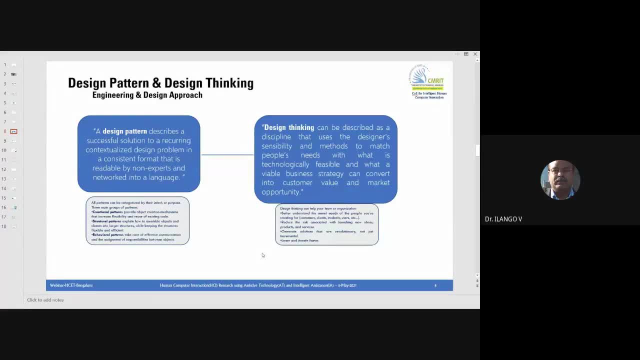 needed for the street vendors. it is successful or not. so what is the benefit of this? who is getting more benefit of this? who is getting more benefit of this? who is getting more benefit? so this is what? that? the challenging mechanisms. we supposed to do that so the street vendors already will not have. 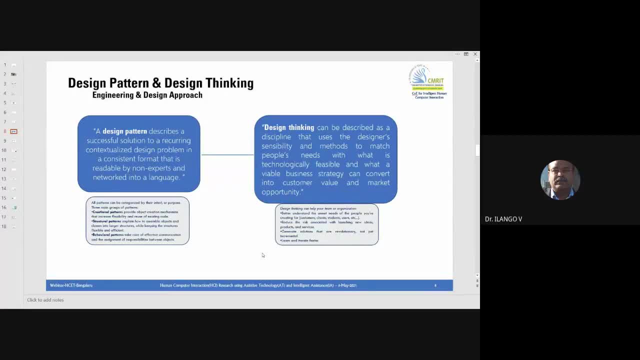 more profit. so if you go everything digital currency, they have to pay the tax or some other mechanisms. also, they have to withdraw the money from the bank and come back and place for their life, a day-to-day life. there may be a. social challenges will be there. emotional challenges will be there, as it. 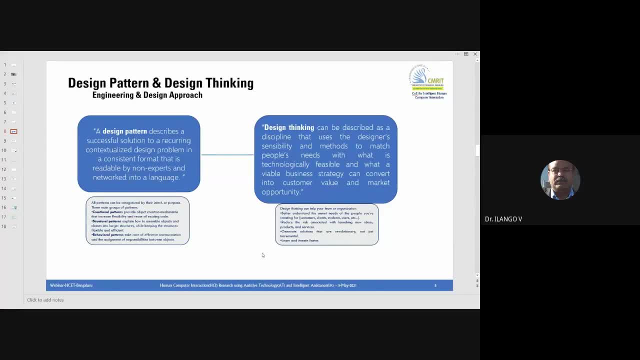 require. we don't know, but we impose of that. it is the care so like based on right. another way, there is a handicapped person. the handicapped person. now they are able to walk and everything on the street plain area. yes, suppose they wanted to climb up in the staircase. it is very difficult. now why. 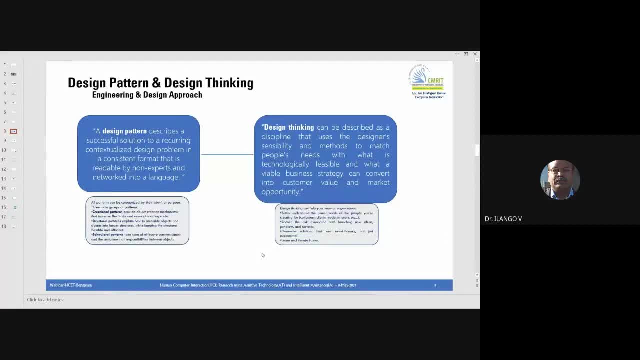 don't you find an interesting device? they are in the home. they wanted to go first floor. the staircase you make on conveyor type sitting machine they can sit and press the button. the conveyor taking along with your bodyguard is there the staircase it will take. under which floor should go that? 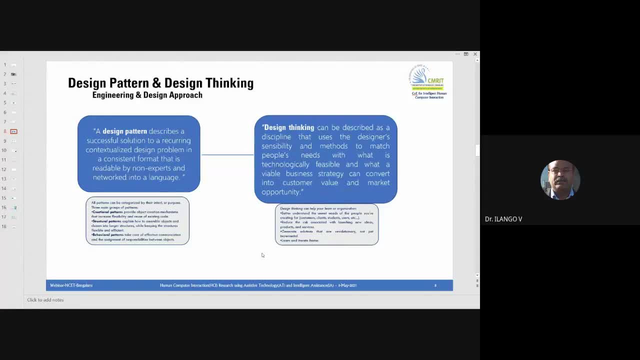 will stop that. it is on lift without having the cabin but it go with the conveyor. so this is one way people invent already invented. I'm just saying that it is really highly reached in the market today but it is very cost effective and space consumption. for that they have five by five size lift it came. 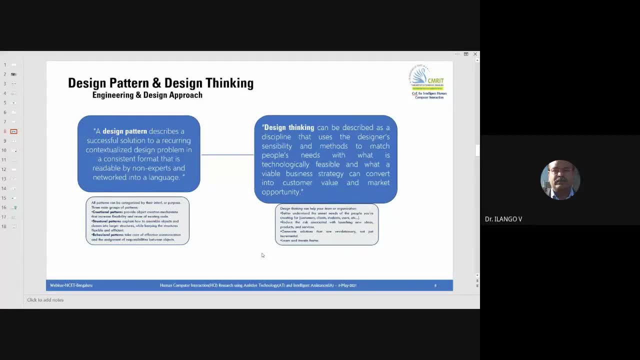 in the market: ready-made lift. bring it and install within one hour time. use the lift which ever floor you want to put it in in your home itself. this is one interesting things for age people. they are very happy, David, people are. who has a problem, a new pain problem? those who 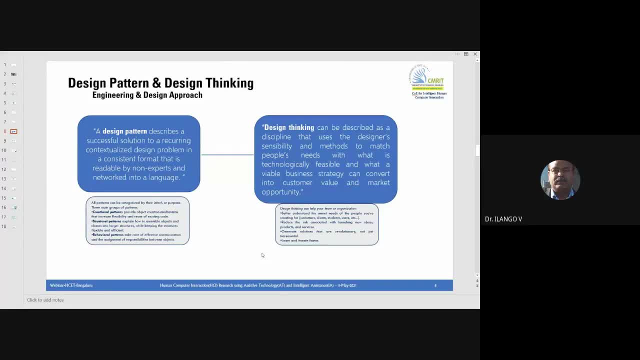 are not able to claim it very successful in the market today. so this is the community who's having after problem. this food device helps staircase climbing, conveyor or lift and we're like vertical boxes. it's there costly, but in people are buying it, installing now. so the design thing is very important is 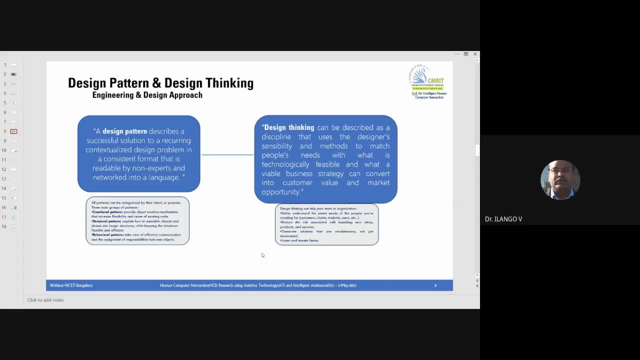 talk about something like community upper their need. is it feasible, able product, happy to buy a, happy to use it comfortably without anybody assistant? this is the one of the interesting intelligent assist, the assistive technology helping a. the people has a problem not able to claim second result, or in the home or 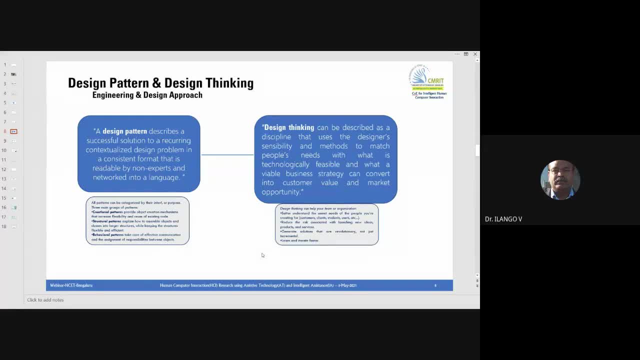 this device, Chevrolet elevator from there will help the lift, vertical lift box, half a deaf cular lift box will helpド länger than ten readers can climb. 근데 you know its very complicated, act them. so this is the thinking. with iot or mechanism, computer science, you can find. 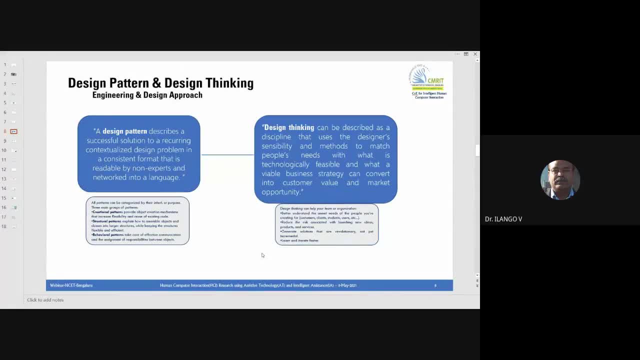 but the same thinking cannot be done individually, it can be done as a team. as a team, you can do brainstorming work, explore the idea, draw sketches, make some drawing, finally come to the design, then map with the design pattern. is it the design? okay, oh right, like that. 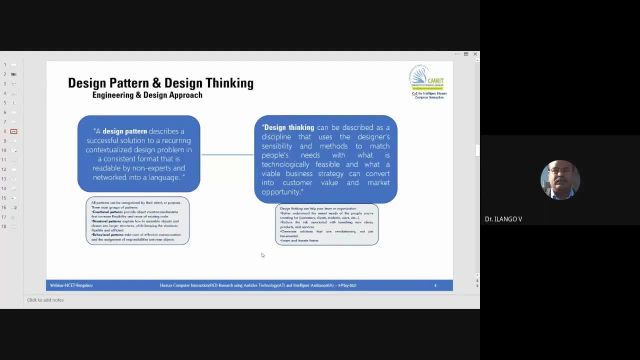 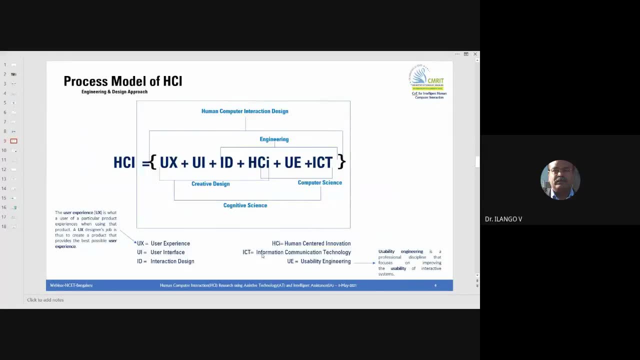 you can go. so these two design pattern, design thinking work together to. i go with the interesting modeling, interesting design, before we go for human computer interaction. okay, so after all that, the process model. uh, do i have time? excuse me? yes, sir, please continue. sir, no issues. oh, right, right, fine, i may be take another. 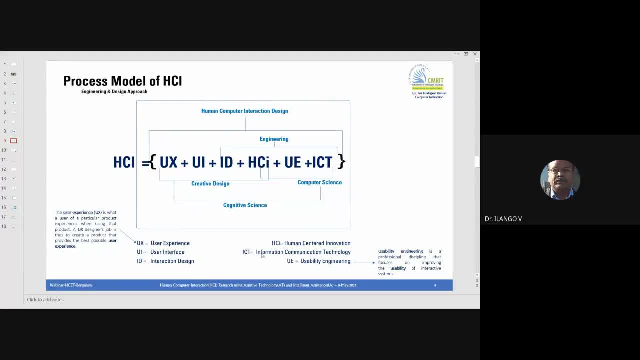 20 minutes. we are in the climate. this is a very important slide. after that i'll show the case studies right. so the process model of human computer interaction. how do we go? i told earlier human computer interaction is not the single domain, it's a model of human computer interaction. 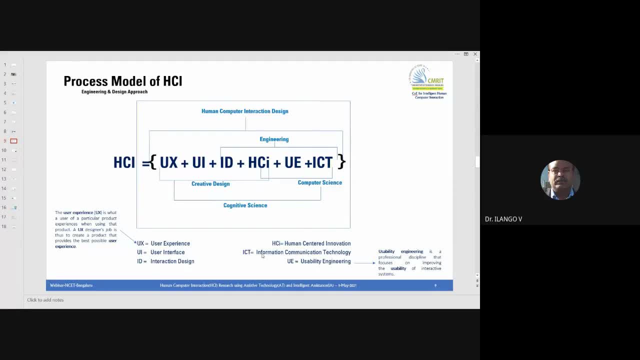 multidisciplinary approach work only. what are the research approaches, their empirical approach approach, engineering, engineering itself, like there's so many disciplines are there and come back: ethnographic also, anthropologist, anthropologist also. we have different type of people. are there animal studies available, human studies available, human studies also, African studies depend. 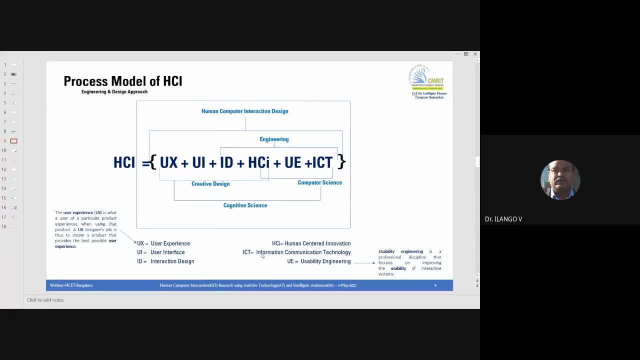 Indian studies depend in Indian itself. Dravidian is different, so there are different things. is there are the Dravidians like that? so many groups available? when come back to Pakistan or UK Europe, different type of studies are there? human culture? even if you take China, they take the food, raw food. 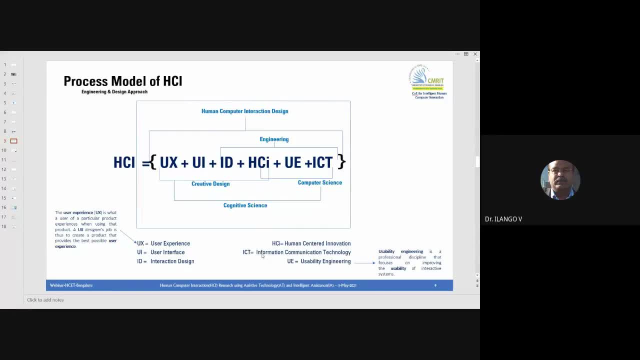 animals or something in India we could not eat. that this is. cultural differences are there. we need to talk to the people with this animal right. so, when compared to that, this is a very important thing: that we need to talk to the people with this animal right. so, when compared to that, this is a very 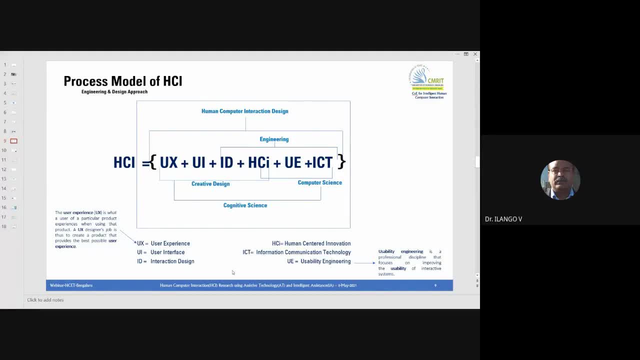 interesting mechanisms available. first, I told cognitive science. so that is a major role it's play. how we can have cognitive science? it can come directly. no, it cannot come directly. it is a collectively formed as a group of engineering. what are the engineering? we need to have creative design first. so 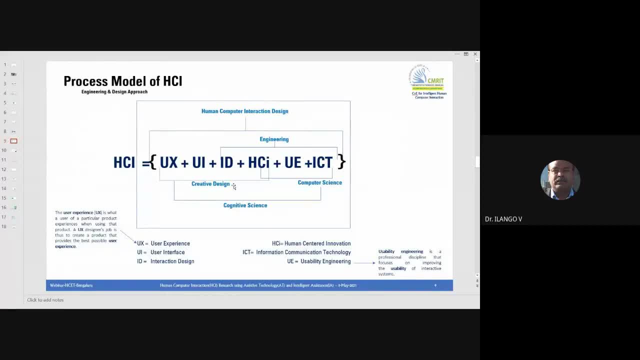 any product you wanted to launch, any process you wanted to learn first, you need to have discussion. you come back with a great idea. how do we make create idea? whether the process you wanted to launch first you need to have discussion. you come back with a great idea. how do we make create idea? whether the 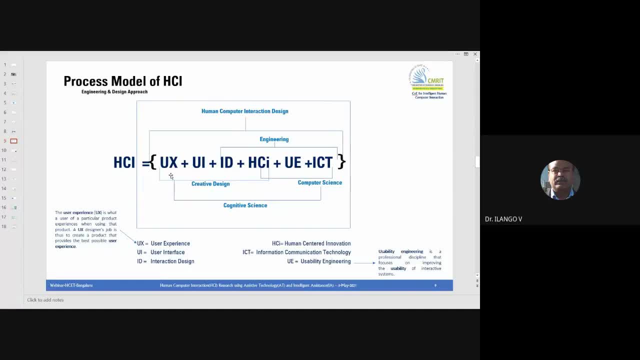 product is edges in the market or not, so we need to have UX study. user product is edges in the market or not, so we need to have UX study. user experience study. if you designs like that, the user will buy or not already exist in the market is a very tough to place, very complex to place. 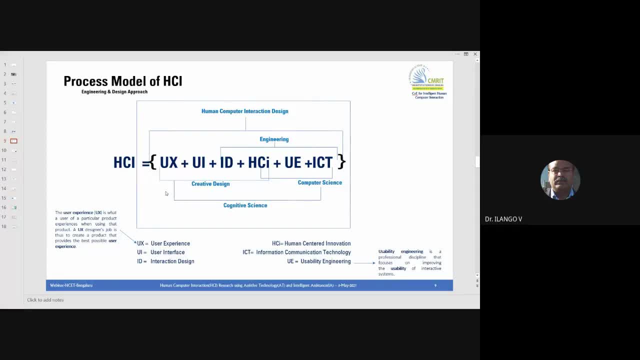 we'll go further, blimey or not. so we are not aware of that oxymeter. till the last year there was there oxymeter. many years we go to doctor to consult the pulse rate. then we'll talk to say pulse rate is like that, we be selected oxygen will. 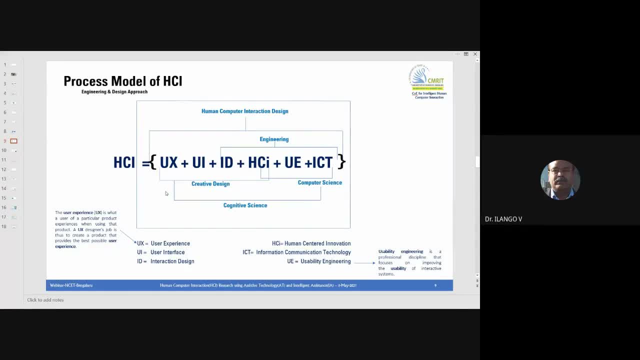 come down, But now, due to the pandemic, the innovation is we have the finger. we can put one small oximeter in our main finger. it will show the blood oxygen level in the human body. New device very successfully moving in the market as and today. high sales could also. 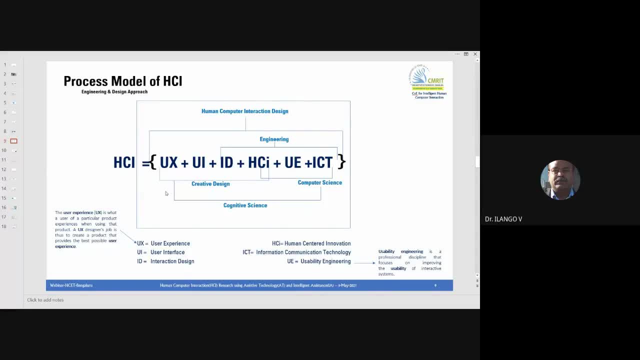 produce in the market today. And thermometer. earlier we go to hospital there will be a glass type thermometer they will put in our mouth or arms. like that they will find it now in digital handy pressing thermometer. 1000, 500, 700, like that it scale every people are buying as a first aid kit. 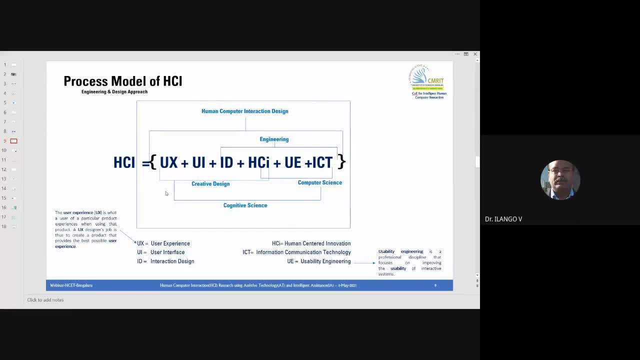 and they are kept at home. how they are found. this is usable. user has got wonderful experience. Even now digital stethoscope came into picture. sorry, pulse testing machine earlier, BP testing. you have to go to doctor now. need not to go. you can buy the baby checking machine. 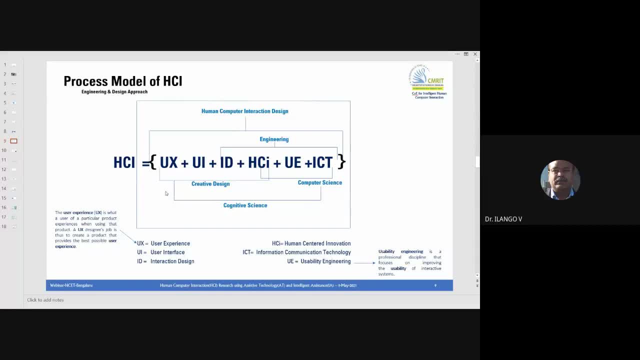 digital machine at home. it is also for 2000,. 3000, may be another 3 years. it will come 1000 also. more people will buy and keep at home. So this is the right time. the innovations came during pandemic people- how they thought. 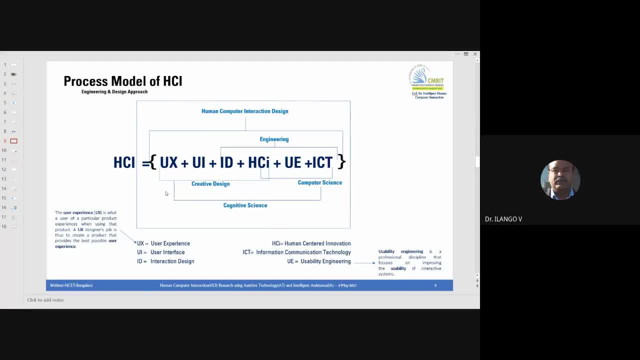 they designed. they successfully launched it, moving very fast in the market: Streaming machine. now different mechanisms came due to COVID people suggesting that export. they are buying it. So user experience is the major phenomena in the market: How user can accept our product. what would be their experiences using our product? we 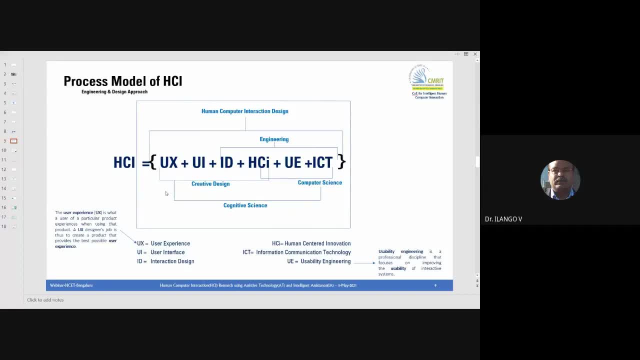 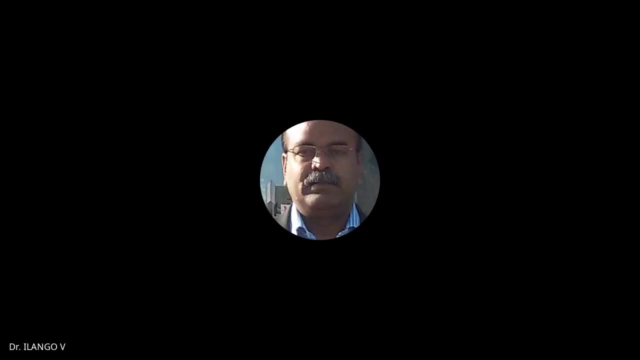 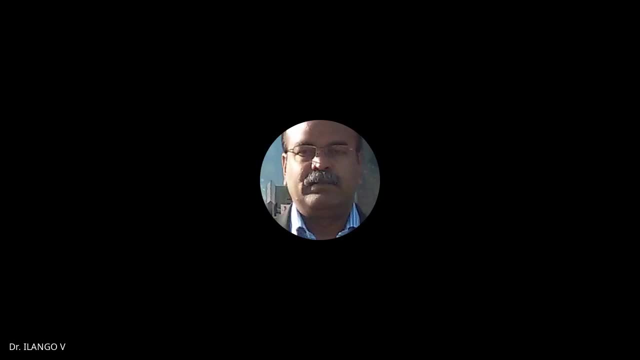 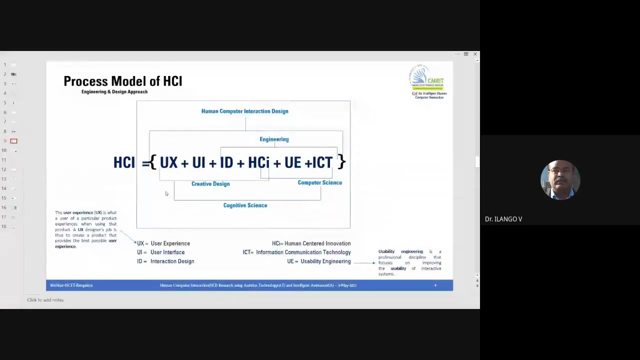 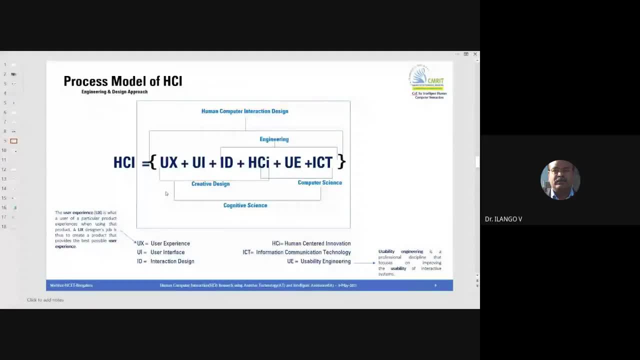 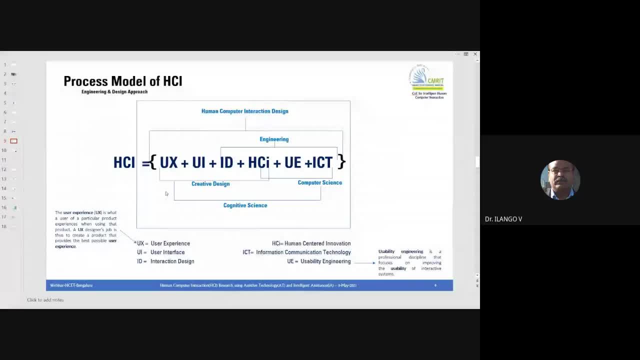 you can see the light. One is for cumulative pulse rate, another one is for blood pulse rate, another one scientific term, I am not aware of that. The three statistics will be displayed in the single screen with the white colour 98. 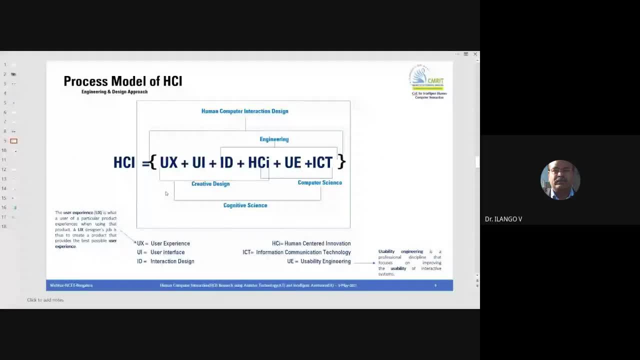 means if you are on 98, it will come orange or red colour. If it is less than 95, different colour will come, less 92. So people will go and see, consult them to get the first aid. So this is the interfaces system. 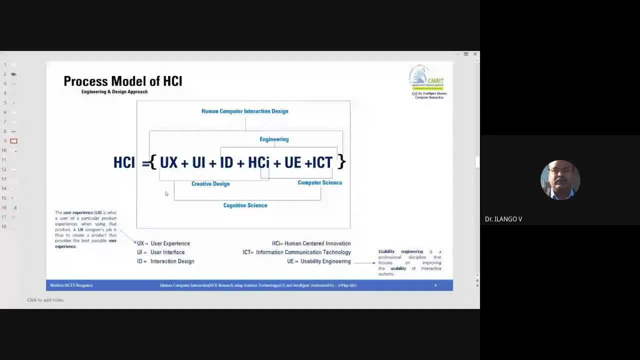 Like that, able to understand the output, even input. okay, it's very important experience and interaction design. so are you interacted with any people or people are interacting with any other devices? so how the devices are going to interact it. so it's handy able to interact like that. you need to go for study in the market. 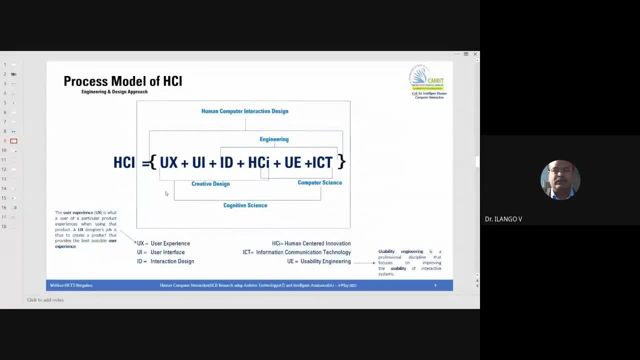 and human centered innovation. anything you invented, it must be for human being, not necessary. it must be for human being, even for bats, animals, plants, also available. we talk about human computing fraction like that. only these are all associated. the millions are associated. only so human centered image you invent. 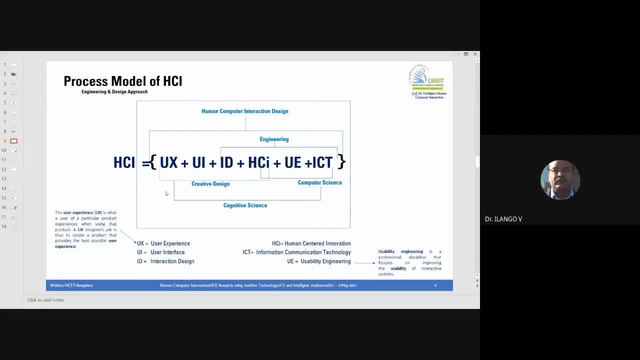 you think about, because I am, but ethnography is anthropologist will talk about particular community, communities of people. people is nothing but human, human centered innovation. everything is for human. we are inventing by the human being. of course that can be used in the animal side plan said also depends a requirement can modify the prototype is 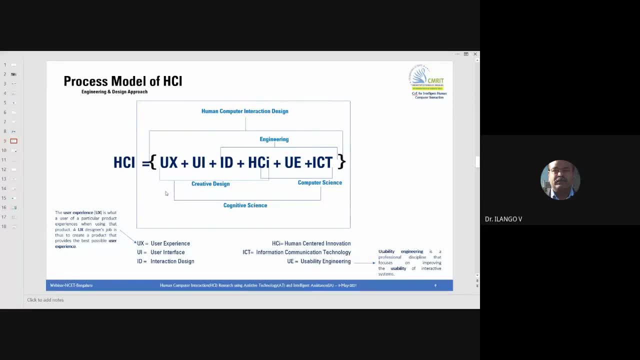 very, very important. you can just invent no use right and information communication technology. without that you cannot go anything. presently, that to the cloud internet- we can't survive. and usability engineering. so this is very, very important. so many products are designed launch in the market is not usable. people are not buying it just like the 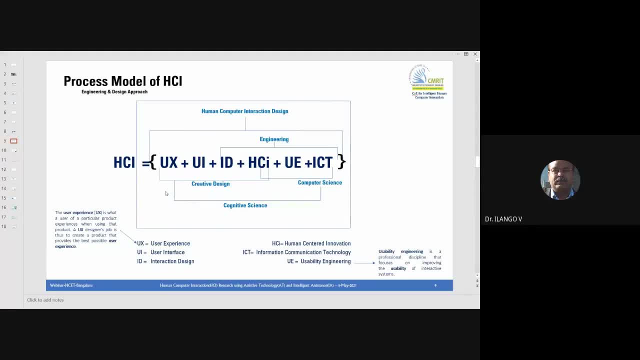 design in the market. various reasons. you can have many China product came into market. if you buy a duplicate product, it will part. that's it. you are not able to use. quality product still has the value in the market. usability engineering is one of the quickest domain and come back engineering design right when come back. 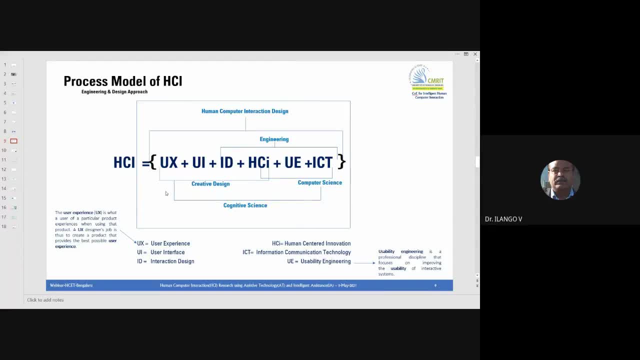 to creative design. there are three. four parameters are very important: user experience, user interfaces and the interaction design, and that all two you should focus for human centered innovation. for human centered innovation, user experience is required, user interface is required, interaction business, then creative design successful after that, without computer science, how? 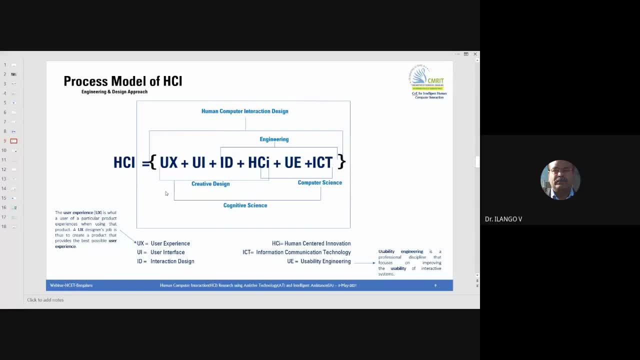 do we go for making into automations or whatever it is so we need ICT. everything is spent product should be successful in the market, moving fast. also, usability engineering must be done. you take a survey whether our post launch, how people using pre-launch also. so these two things should be important. creative design and 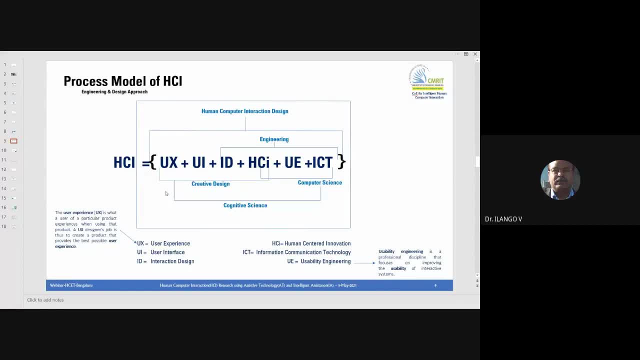 computer science, both together. cognitive science- cognitive science, as we told that human mimics human brain activities, means simulation, so artificial intelligence, so computer science. produce that human thinking artificial way with the help of creative design. finally, engineering engineering means robustness and portable safety, security. all will be fine in the engineering mechanism, there only people. 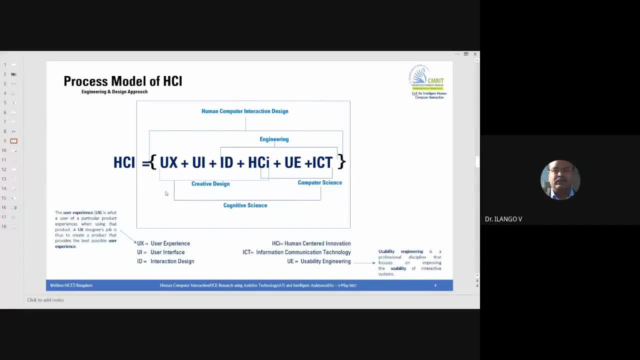 fix, warranty and guarantee that ID, I, HCI, EE, ICT all together command engineering. all these six elements, yes, yeah, ID, HCI, EE, ICT together come to succeed a mission activity, that mission activities. human-computer interaction: when human-computer interactions would happen for any other innovations come to market for usable, the six would be: 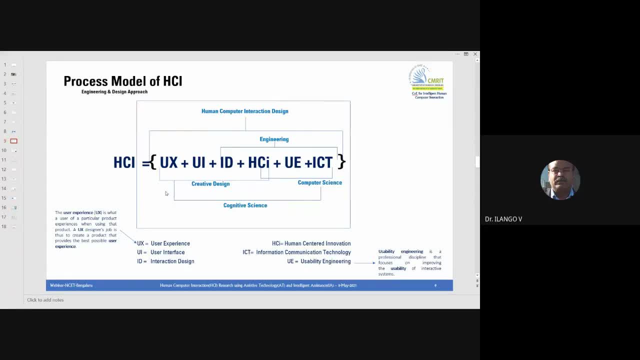 implemented. so this is the very interesting process model: each area: experts are there, engineers are there. scientists are there. engineers are there. it is not by one people. so where you would like to fit yourself, you want to be in the creative design? yes, stick into yourself. you want to be computer science? 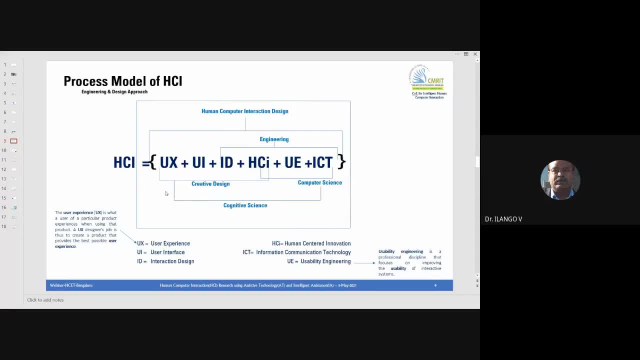 supporting the creative team. yes, you be with them. you want to be cognitive science engineer, a psychologist or expert- something knowledge of expert systems want to fit. yes, you be there, you provide the solutions to them. you want to be only engineering engineer or engineer, hardware engineer? yes, you be a. 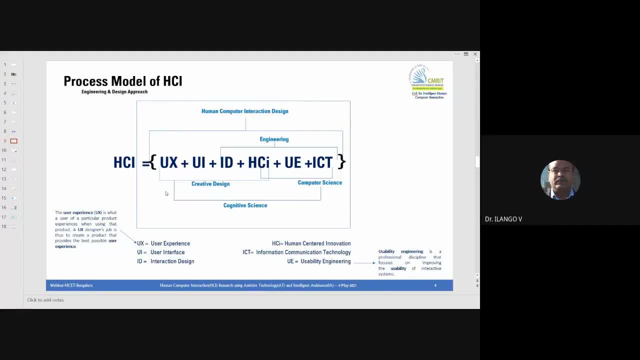 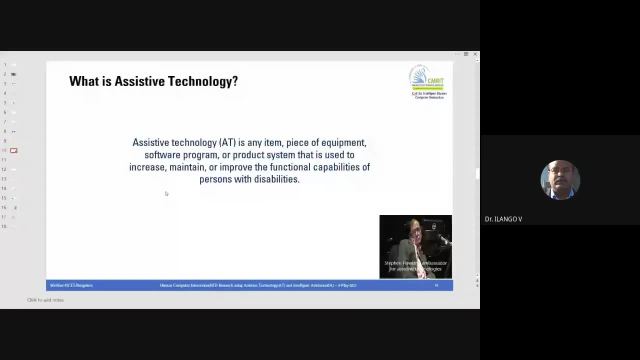 backbone for all the three elements and then you fit your. you would like to process knowledge or succeed yourselves. this is the biggest framework. this has to be done successfully. and come back to process model right. so now we move into assistive technology. so assistive technology is any item, piece of equipment, software program or product. 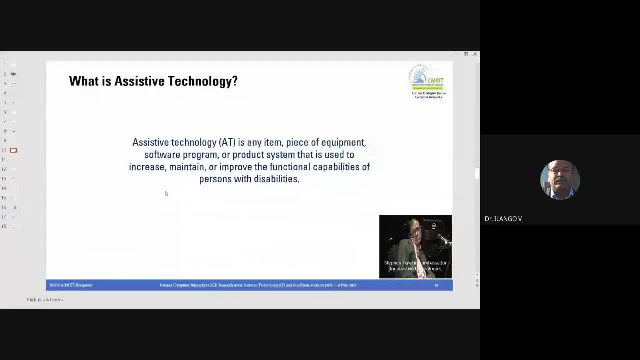 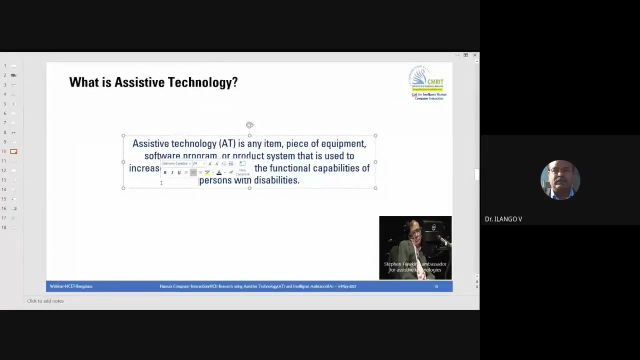 system that is used to increase, maintain or improve the functional capabilities of persons with disability. the main assistive technology came for the disabled people. not necessary. only disabled people only should use the assistive technology. other people also able to place that. that is a interesting phenomena. so wheelchair was there. now, 25th century, automatic. 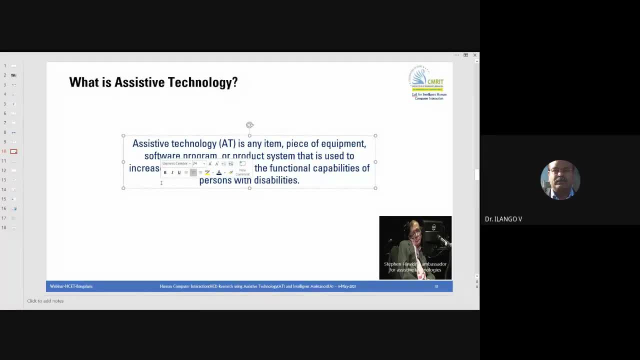 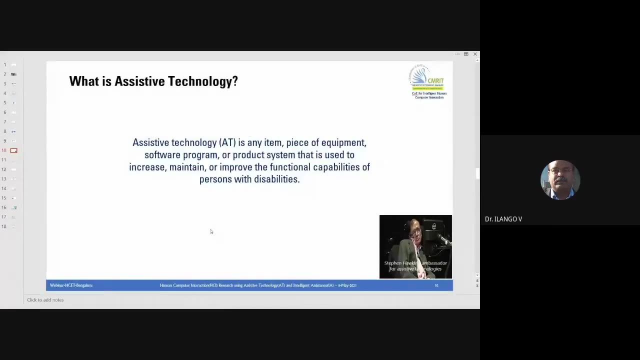 wheelchair. it recognize the people. see this person, Stephen Hawking, is ambassador for assistive technology. he was living in the wheelchair only so many years he invented and so many ideas are so many product. how was possible is mechanism so assistive technology? initially it was launched for disabled people, but now 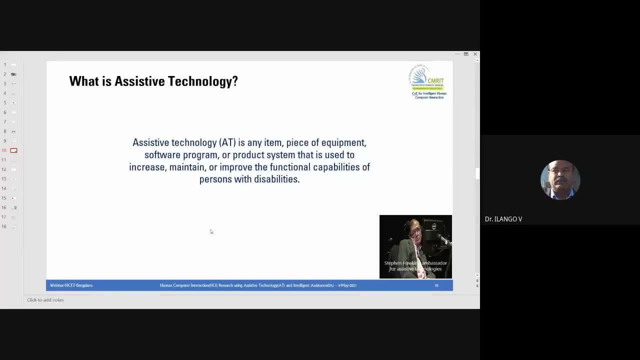 Now everybody is using everything. It's not only for disabled people. but particular design is there for particular people, For autism people. certain types of designs are there If polio or something a handicapped right hand is not coming for them. different types of walking sticks or shoes are available: automated shoes. 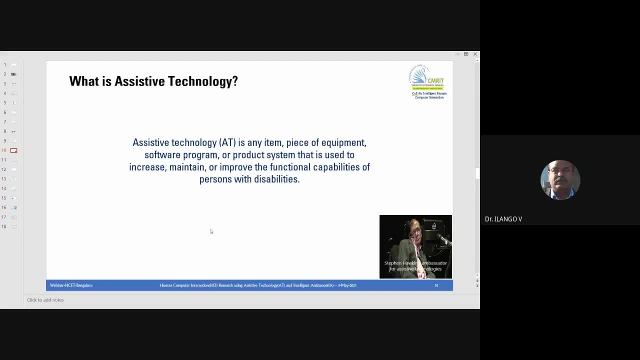 Like that eye system: blind, partial blind. Now recent technology came for full blind also. they would like to give a third eye. New technology came third eye mechanism. Through that they are able to visualize something. they are able to show certain visions also. 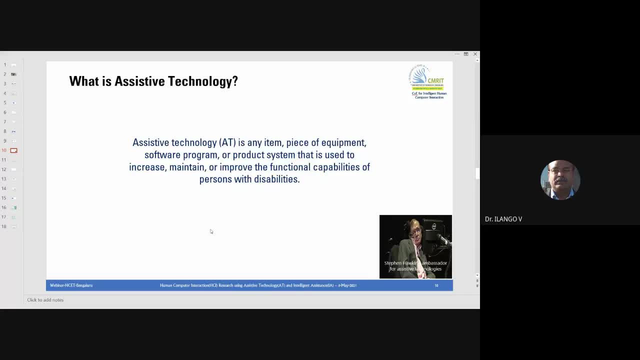 This is interesting things. assistive technology- So any people, even presently, online education. we talk about normal people. online education is okay. We are able to hear audio, we are able to see the video, But how the blind people are able to see the video. 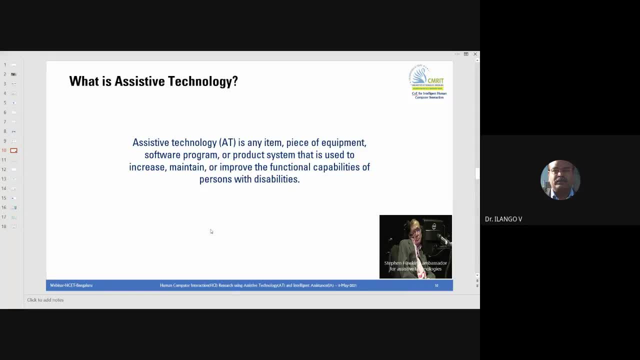 How the deaf people- or dumb people, deaf people- are able to learn this online education successfully. What is the solutions we are going to provide? Is there any device for them? Is there any solutions for them? Are we going to ignore them? Are we going to include them? 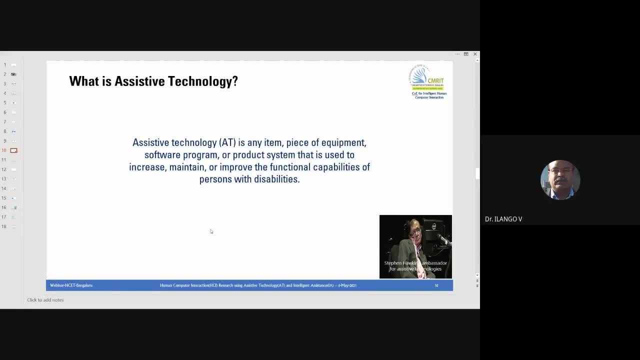 This is the biggest challenge in 2020.. March we started online education. Huge challenges was there. They were totally neglected for 2-3 months Later. later, small, small solutions founded. Still, it is not in customized 100%, But at least solutions are provided for some extent. 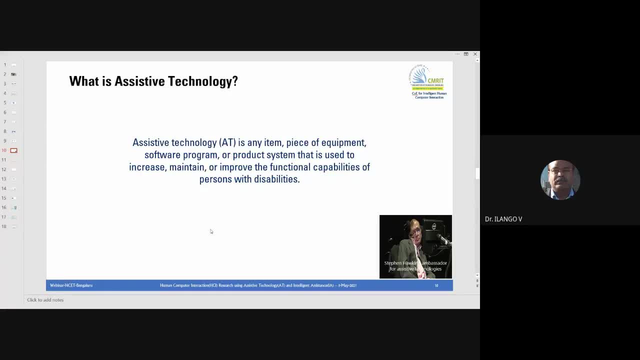 This one year: innovations, But still there is a gap. Some complete solution is required for this people. handicapped people, Particularly visually impaired or hearing impaired or speech impaired people Need solutions in the online education system, Online learning, online business system. 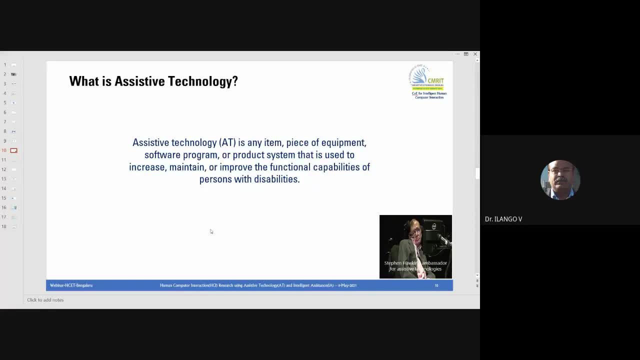 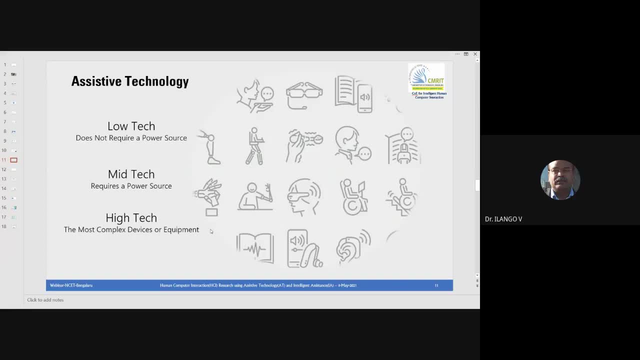 So there lot of gap is there. You can find assistive technology, design assistive technology, You can come up to the market. So assistive technology, low level, mid level, high levels are there. Low level- there is no need of any power sources. 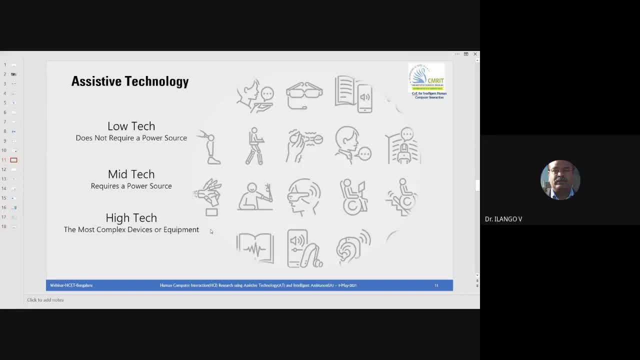 Like pencil, pad paper, notebook. These are also very comfortable. They can design and provide And mid level, little power may be required. Calculator like that devices. Also assistive technology solves certain problem. High tech mechanism means like laptop or computers we are using. 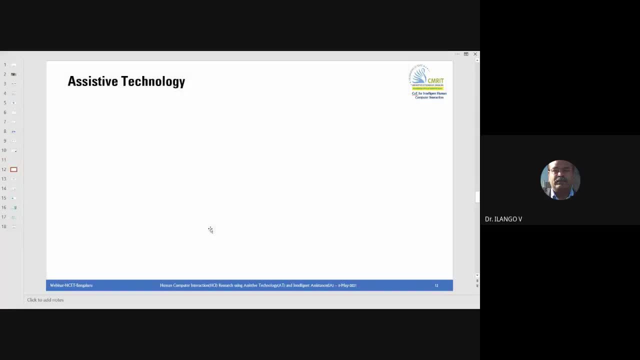 We may need more machinery things. Electricity is much required. Electricity is required very much. So these are all the high tech team. Electronic dictionary alpha smart keyboard. I just read one minute Audience. please read one minute. Like that. low tech also there. 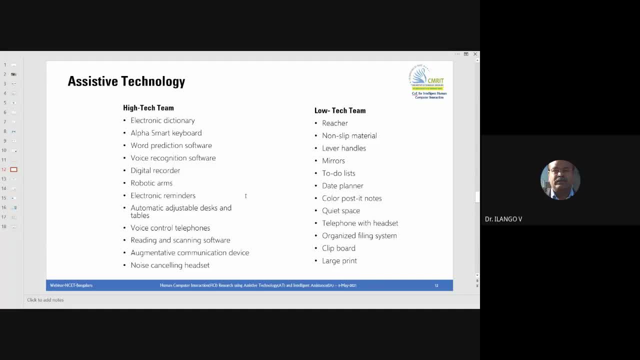 Assistive technology When compared to high tech team: Electronic dictionary, alpha smart keyboard, Word prediction software, Voice recognition software, Digital recorder, Robotic comms, Electronic reminder, Automatic adjustable desk, etc. Voice control telephone- So many. 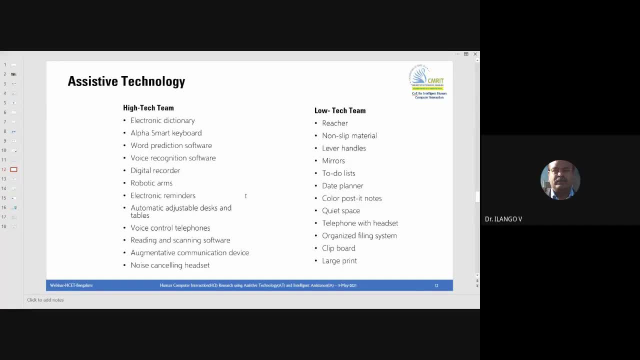 So many are there. These are all the only things I could bring into screen effectively. These need more power consumptions maintenance. We will come back to low tech. This may not require much power sources. It can be easily carried forward. Anybody can operate it. 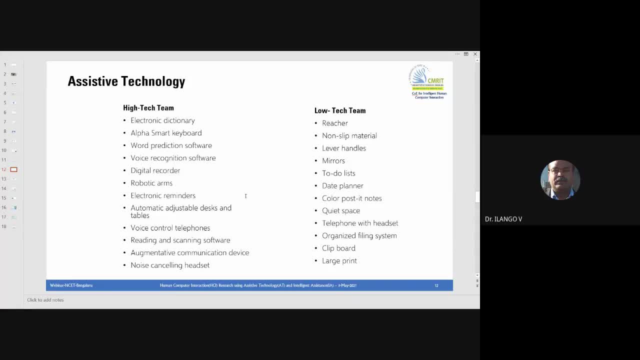 Even it is lost, not a problem. There won't be much damages. Also, cost is not much. So this is non power sources Or minimum power utilization. So this is not a problem. This is not a problem. This is not a problem. 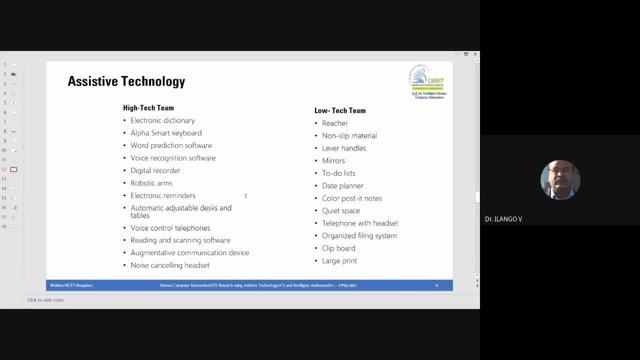 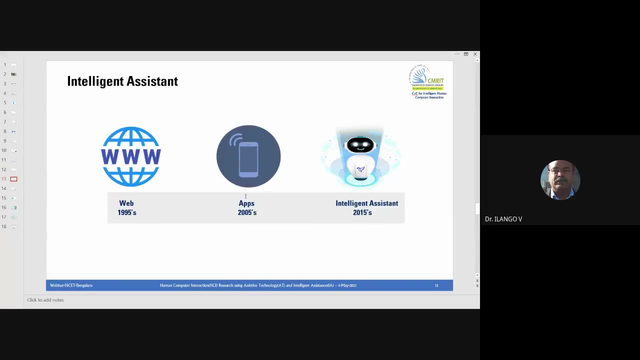 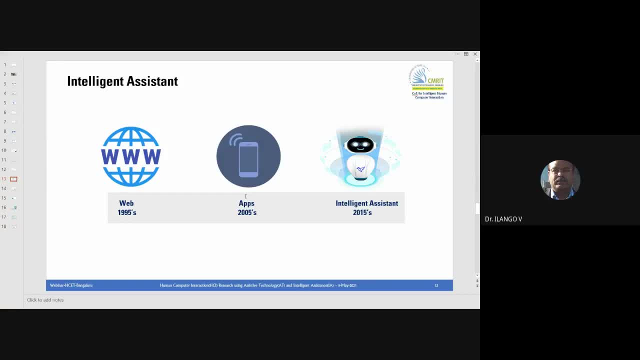 Are you able to see this screen, Excuse me, Ok, fine, So again in 25th century, only the web technology came into market. People started to use. internet was very popular in developed countries. later, 80 developing countries, later, 95 later, only this system came into market to windows operating system. 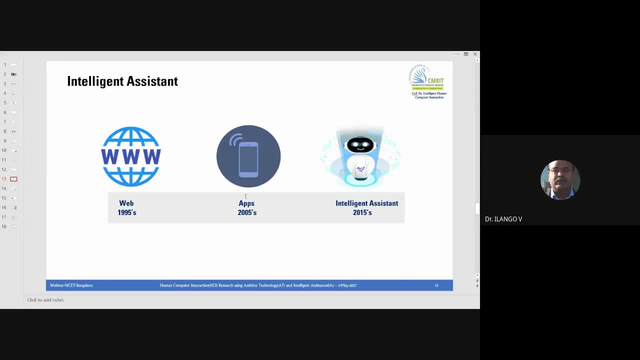 95 graphical user interface successfully launched. thereafter developing countries were using effectively, efficient, not only developing, all the whole world universe. so from there it started the era. late 2005 in poor system developed country people started to use mobile app system. late 2010, we can say in developing countries. 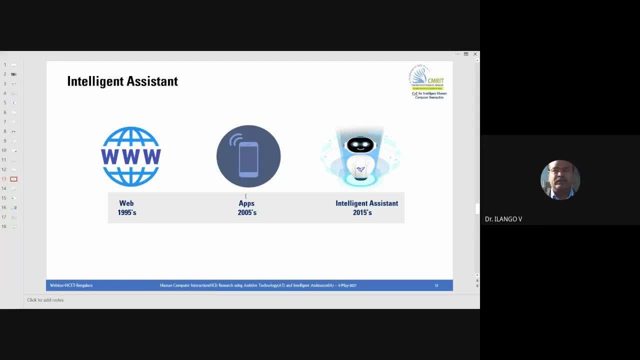 then not. well, everything is begin the mobile app systems. mobile app is the mechanism nowadays for every teach and everything. mobile app only. anything you do you want to mobile app, mobile mobile computing, okay. beyond that, using this web, using this mobile app, something else is their intelligent assistance. so why? 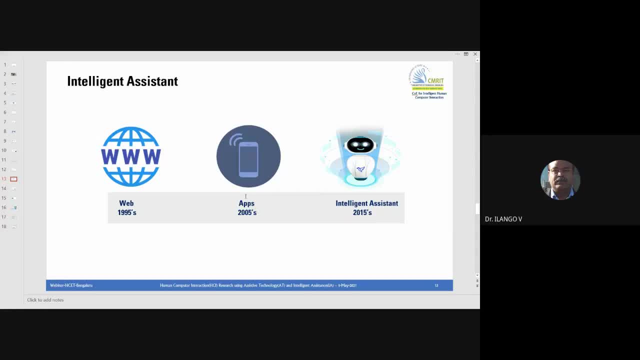 don't we amalgamate that web technology and mobile technology will put together mobile computing, web computing, mobile interface, web interfaces put together, then we will make some assistance system which will be carry forward, which will be portable, which can be used by any community. one device for any community, any community, many community for many. 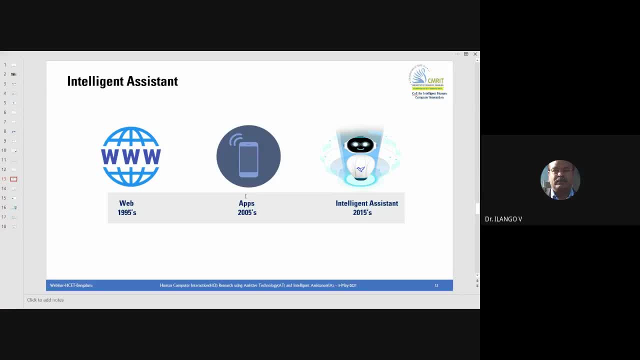 devices, one community, many devices like that mechanism scale to assist the day-to-day activity efficiently, effectively. intelligent assistance play major role and trust and scenario. without this we are not able to use access. many examples let me tell you today they are searching for our position, options in our business. 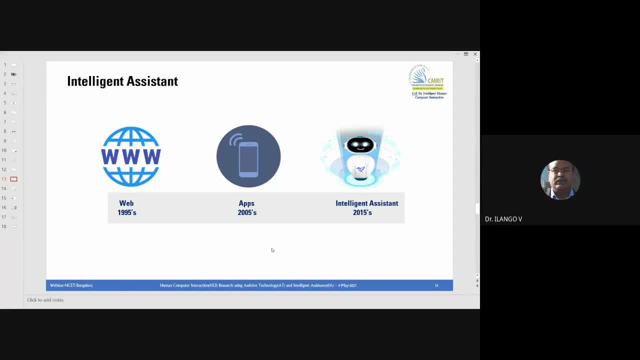 cylinder. already last week, two weeks before, one company has invented to produce an audition machines. it is 40,000 rupees. people buy this device. install it your home for one liter water. in the glass plate they have kept one container. it will producing within half an hour the audition. you can consume the. 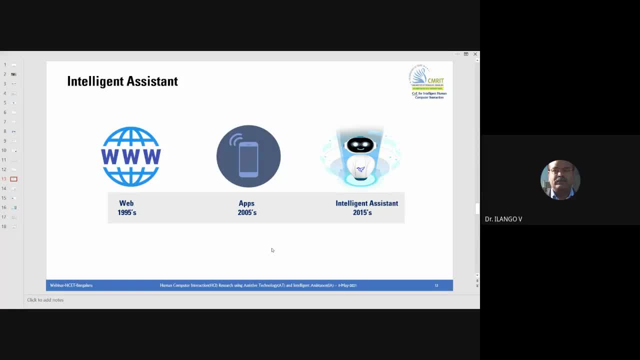 ambitions for your business, for your safety, but instead of going to hospital, spending 40,000 per day, one device for many years it may come. it has already launched a timely, launched it as far as the claim and air purifier systems also launched. now here, people's 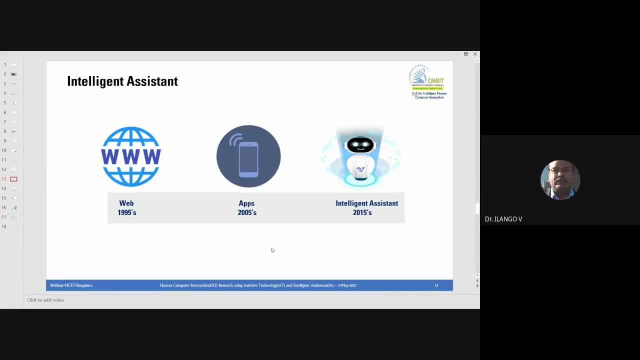 is Tyson, come up with a new mechanism. assist- these are our intelligent assistant- very fast and it is purely installed at your own place at home. it wherever you go. that need to be checked at the best year and feel bad giving back to your home, not buying it now due to pandemic like. 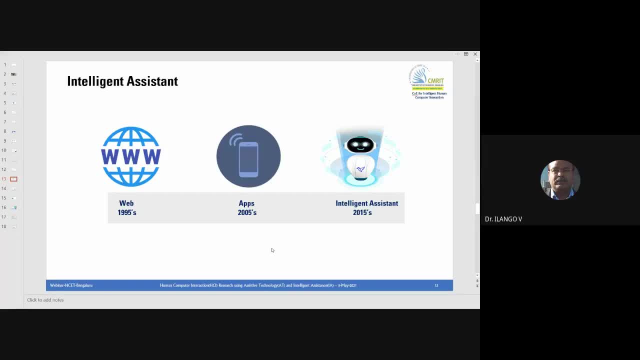 many, many assistive technology came, which is display devices, which their display will be there. air purifier data will be displayed there. how was the air before around? how is the air before that? are you able to inherited eco like that? messages will be display effectively, efficiently. so I told aximeter: let it. 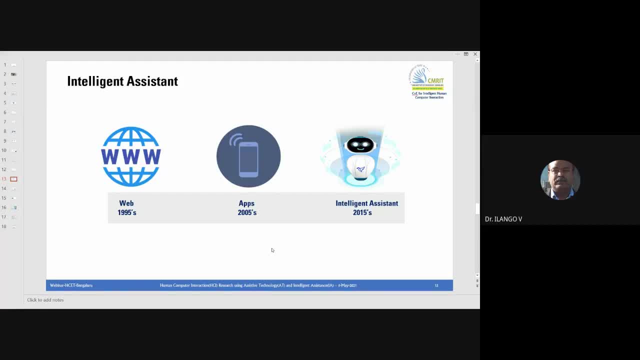 many, many devices also right. so this is a interesting things available. assistive technology simply say. I use a software agent that can be performed task or service for an individual. it can be customized, it can be personalized as per the requirement so we can use and come back to see our 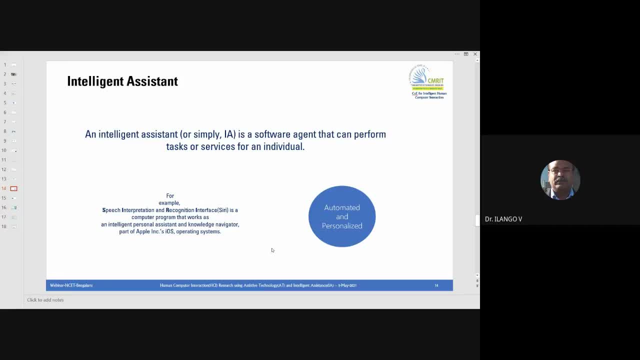 speech interpretations recognition interface. it's a computer program that workers and intelligent as a personal assistant or knowledge navigator. part of Apple industry iOS operating system scheme and Alexa also one of the individual assistant. it helps for people. many of software oriented devices which enhance their hardware performance also available all group, all group for that. 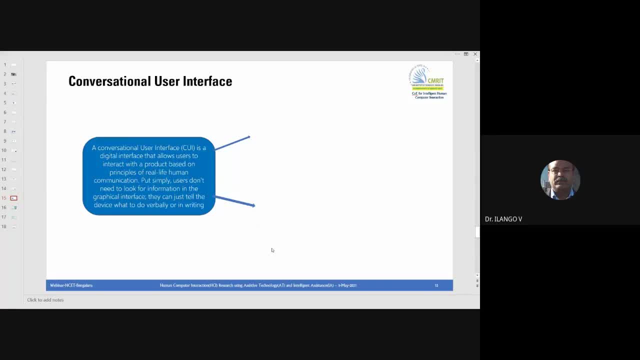 one backbone is conversational user interfaces. this also play major role to activate assistive technology and intelligent assistant. the conversational user interface is nothing but it's a digital interfaces that allow user to interact with the product, based on the principles of real-life human communication, but simply use. don't. 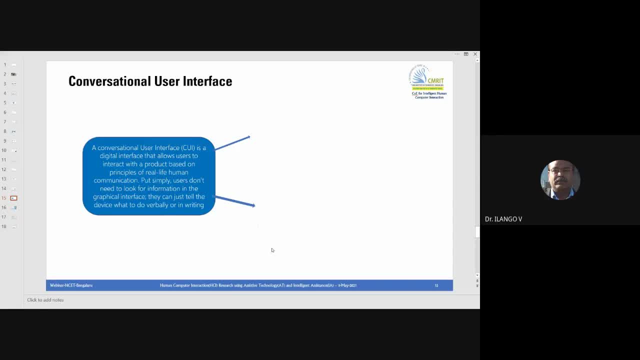 need to look for the information. they can just tell that device that what to verbally or writing, so you can talk as you talk to Alexa, so you talk, it will convey the message to other end. you can type the text. it convey the message to other end. you get the replay. so like that presently. without that they are. 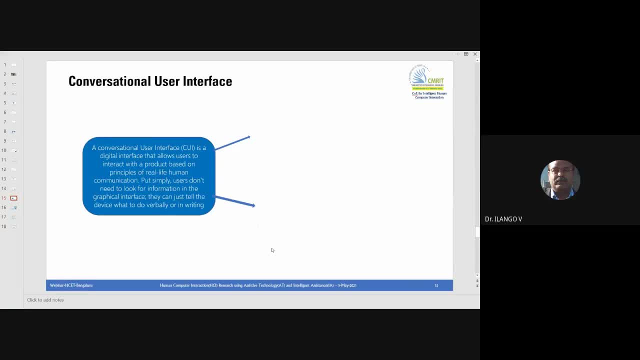 able to. we are not able to survive. you can have whatsapp also, you can have chatbot also, but many other things available. certain things for one only corporate level, organization level available, certain things for personal level available. So let us see what is for corporate, what is for personal. 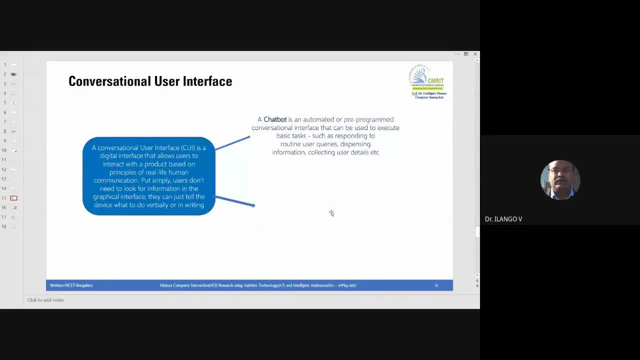 Right. so one of the important things, chatbot. Chatbot is an automated and pre-programmed conversation that can be used to execute basic tasks such as responding to routine user queries, dispensing information, collecting user details. This chatbot is for an organization level. 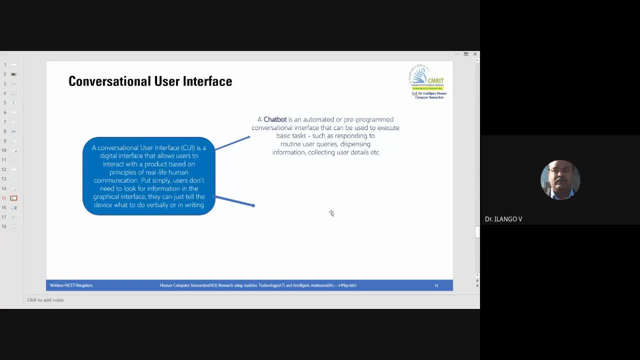 it will be there, any of even your organization. also, some chatbot may be there. When you open the website, it may come with you looking for any admissions. which course or shall I help you? like that? Automatically the messages will come. 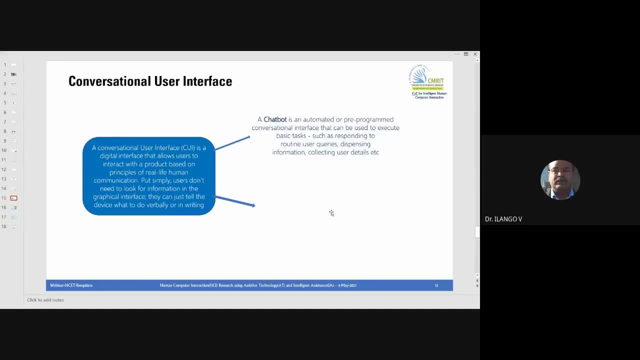 If you replay it will come from pre-recorded information should be displayed to you. It can be captured and customized for a particular thing, for organization level. So this is a chatbot. it is very familiar presently across that many are trying to construct their own bot. 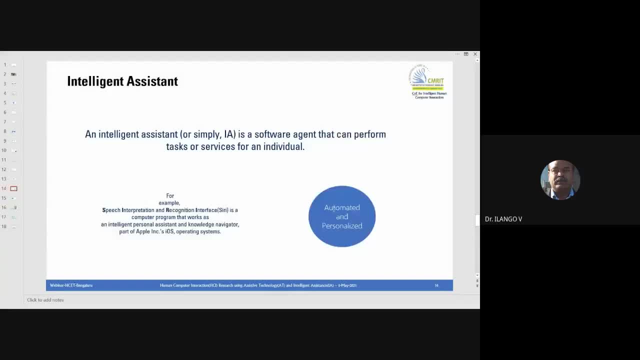 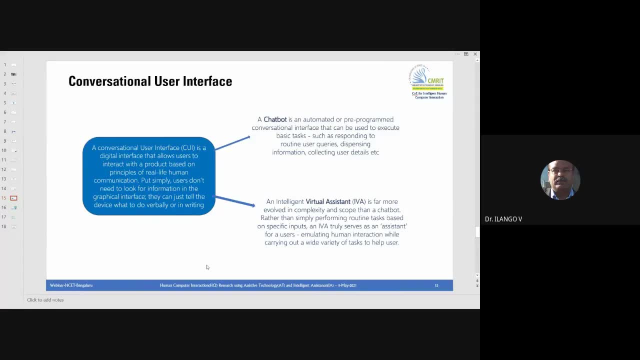 they're using also successfully. it is working very well, right? So next interesting thing is intelligent assistant. Intelligent assistant is also far more evolved. it's complex things. It is better than chatbot: Simply perform a routine task based on specific input. 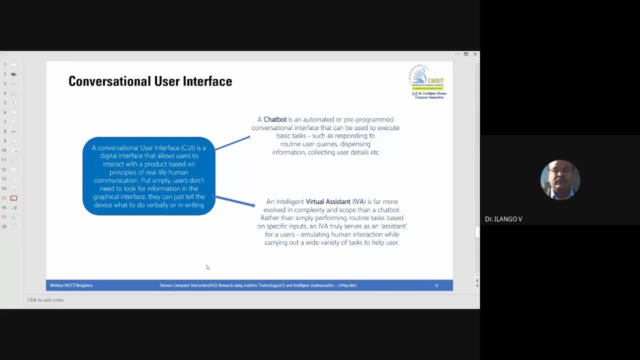 The virtual intelligent assistant truly serves as an assistance for a user, emulating human interactions while carrying out a wide variety of tasks to help user. So this is not only for organization, this is for a specific user, also For specific organization, this intelligent assistant. 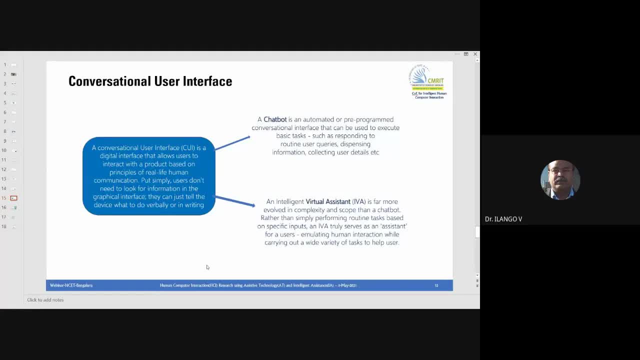 is for particular individuals: handicapped people or blind people, partially blind people or a deaf, partially deaf or not able to hear, partially able to hear, According to the level. the assistive technology- software as well as hardware support, will help to picture. 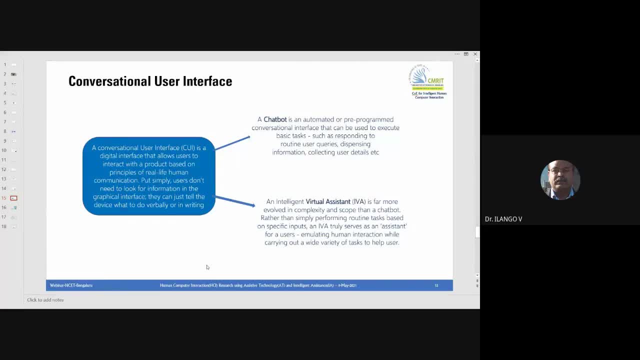 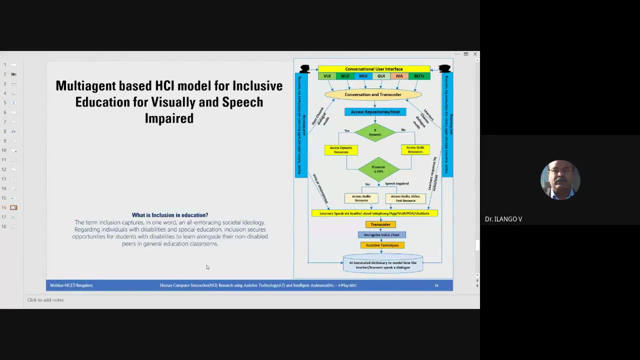 these two conversational interfaces and to stop chatbot as well as assistive technology, a virtual assistance also. This will help to assistive technology as well as intelligent assistance. So we have done some projects and it has been patented also. So I'm just saying, due to some confidentiality. 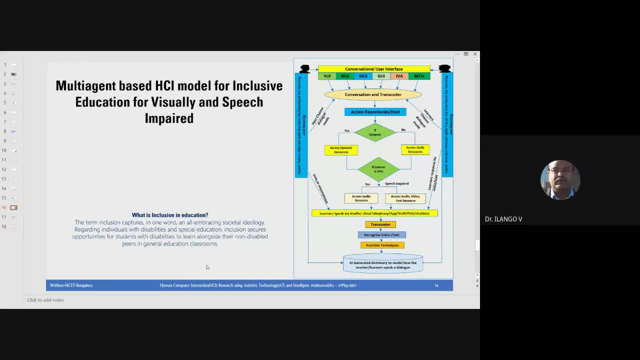 I cannot explain in detail, but I can show only the block diagram here. I'm not able to copy the prototype. This has been patented. So from our lab we have done what we have done was inclusive of that. we've done the. 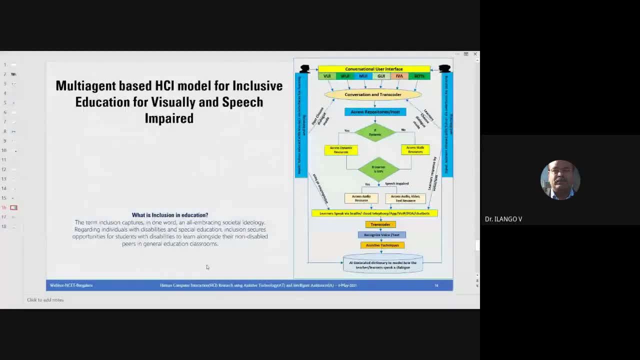 online, So we've used this. So this is, for example, the mobile. This is for a child, So it can be your laptop. Use a with the keyboard So you can do that on your laptop. user multi-agent based human-computing interaction model for inclusive education for visually and speech impaired. 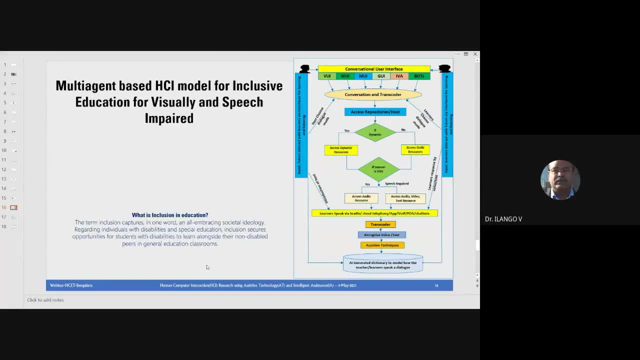 Inclusive is nothing but as students come for computations class, algorithm class, normally he is a normal student. He does not have any kind of problem with hearing Along with the student. how one blind student, complete blind, partial blind- can learn Along with that normal student. how partially hearing or no hearing student. 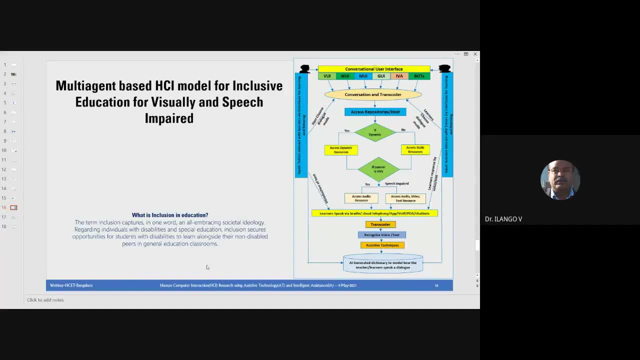 how, partially talking or no talk, that type of students can learn as if the regular students learn. This is the biggest challenge. So we could not do completely the third eyes mechanism. Our approach was something different, But we have succeeded partially. We are not able to succeed completely. 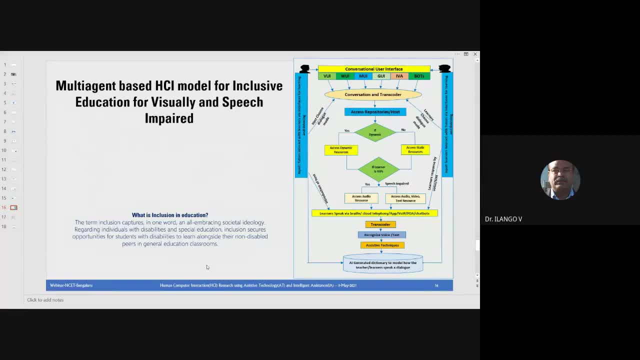 It was a big challenge, But some extent we could succeed. Still, there is a gap. Maybe other generations can do that. So inclusive education is the biggest challenge. The term inclusion is captured in one All-embracing societal ideology regarding individuals with disability and special education. 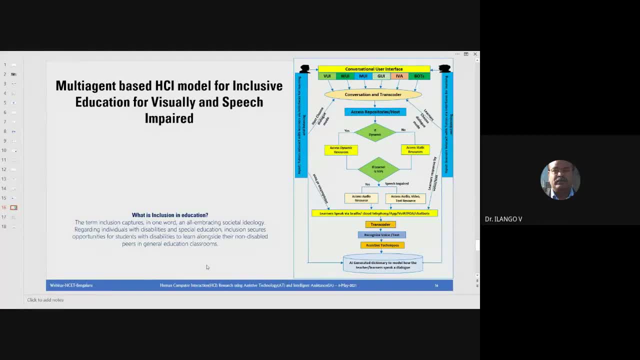 Inclusion is a secure opportunity for students with disability to learn alongside their non-disabled peers in general education classrooms. This was our aim: to develop the event. What we used? We used conversational user interfaces, So voice user interfaces were used and web user interfaces were used, and mobile user interfaces and graphical user interfaces were used. 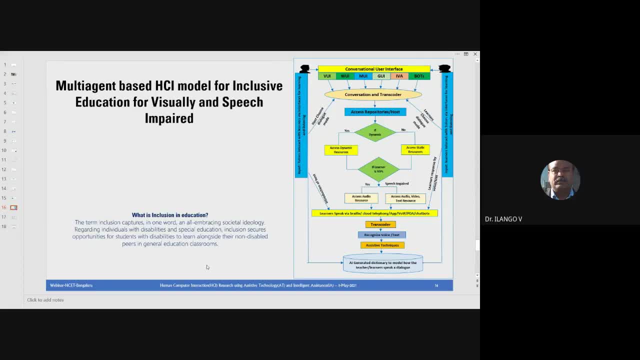 We also used an intelligent virtual assistant and chat Also, we used it. So there are all devices. It comes to one converged place. There, normal students will pick up what is the care for them. The partial blind or speech person will pick up one of the parts. 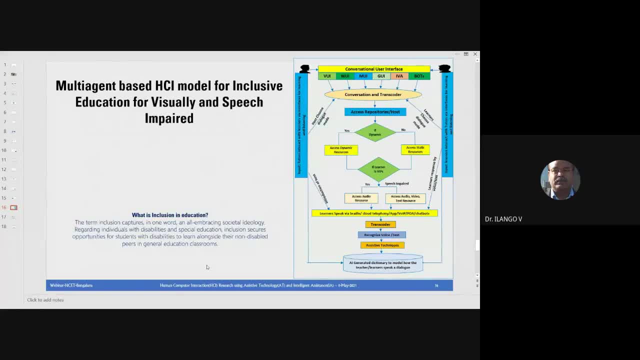 Maybe he may need chat. The person who is able to type Vision is there, Not able to talk. Hearing is there, He can type. He can chat for you. Vision is not there, But he cannot type. Vision is not there, He cannot type, He can hear. 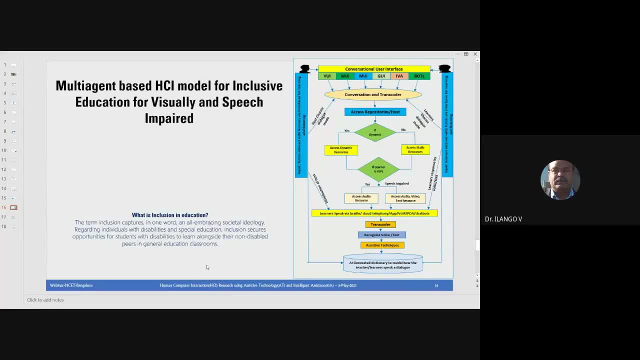 So he is using intelligent assistants also Like that, who want to use which type of tool they can pick up from that common portal. They can utilize it. Then you input what is secure from the first site: Delivery lecture or pre-recorded lecture or online lecture. 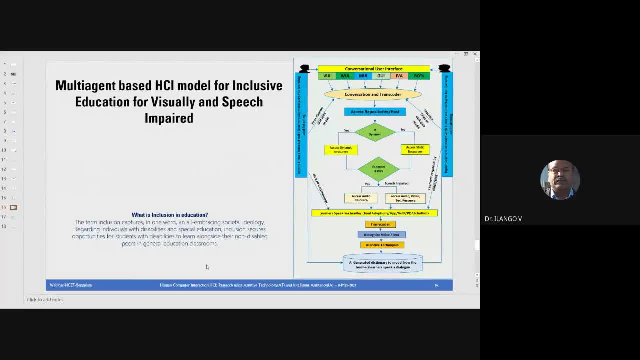 Both they are able to access it. So they are telling that. dear my tutor, please- I said blind talking- Please give me operating system software. There was a subject: Tenth day lectures. I lost it. Then, system lost. Tenth day lecture: Which semester? Tenth day lecture? 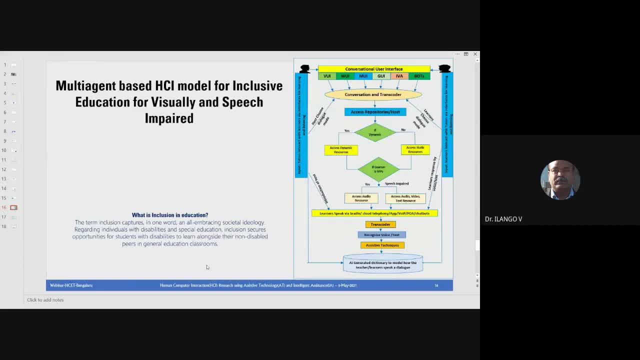 You are in present even semester. This subject was there: Hard semester, also Hard semester, also Tenth day was there. You are in even semester. Which one I want? I want even semester tenth day lecture. This is the lecture title. This was the tutor hosted that. 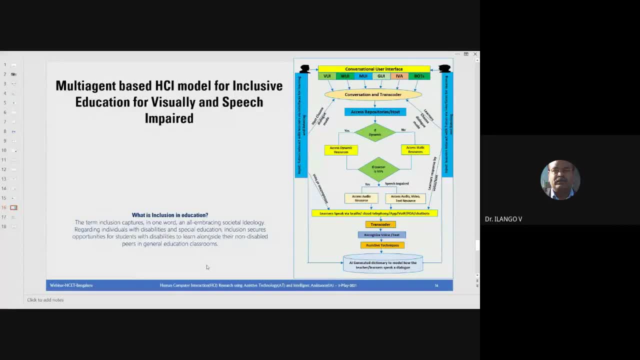 You can access it. Can you play it? Yes, I will play it. Keep the audio system and play automatically While playing. you can stop It will stop. You ask posting. It is pre-recorded, But you are asking posting It replay to you. 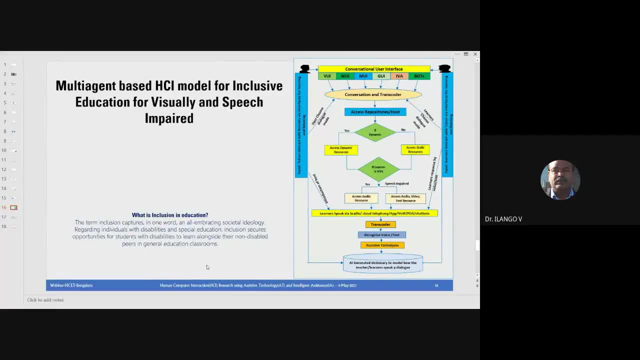 Either immediately or maybe subsequent time. This was the ultimate object which was there. It was very successful: demonstrations, Product. when come back to product, we struggled a lot. There is a big challenge, But prototype was very successful. But likewise, any people can. 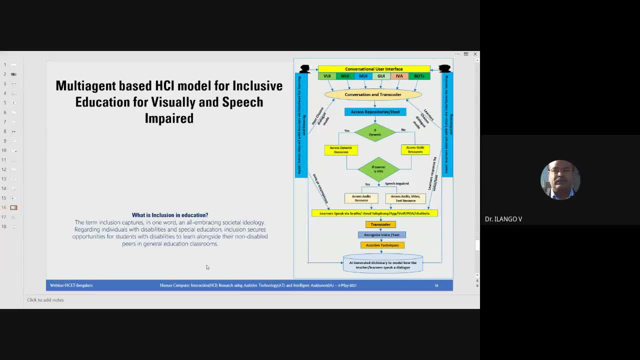 Live session. no problem, I have entered in the class. Yes, Confirm you entered in the class. Your attendance are given. Okay, You can start lecture. So the tutor is posting lecture. He is observing online Online, no problem. Question asked that. 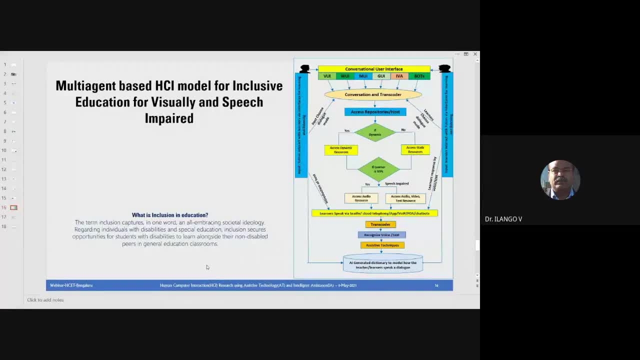 They will be able to interact with you also, Not an issue. So this is happening When they want to see what to do. They will not be able to see, But we can make them to visualize As if they are able to see the normal students. 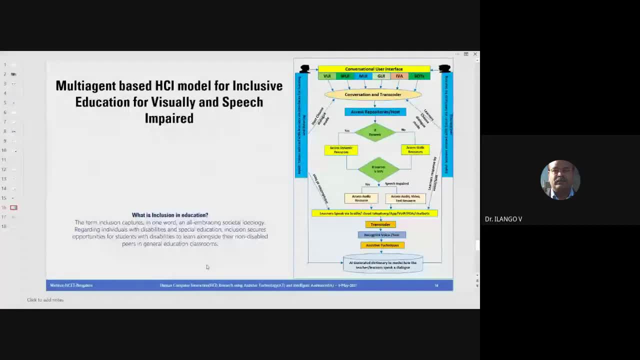 That is very challenging. It is done Likewise. there is a mechanism, Both the side- interactive queries are there, The dynamic access also, Static access also If it is virtual implant, dynamic accessing What to do. Audio or video can speak. 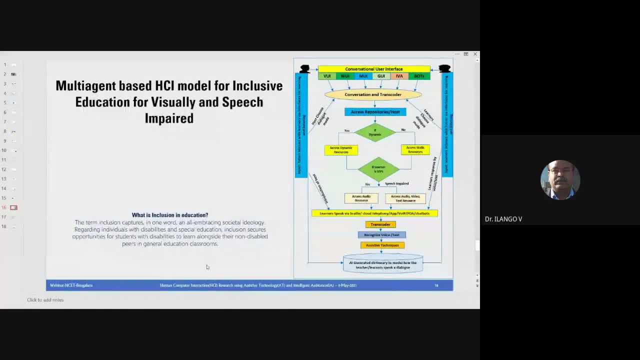 Or three things can speak. There is a converter which should be there In the middle: transcoder. The transcoder will convert whatever language it can be. The person knows only Malayalam. You can speak in Malayalam Immediately. it will go through natural language process. 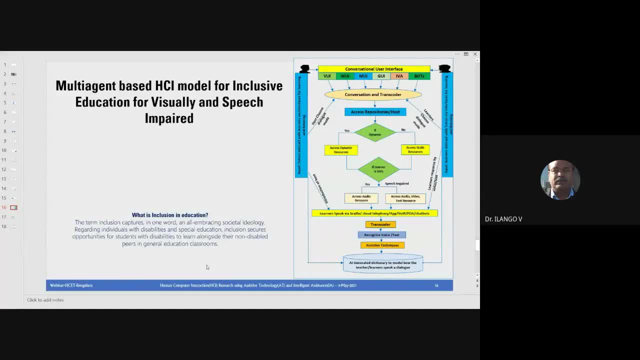 It will capture the video Automatically. it will be putting the captions or label. It will translate to them, Or audio will translate Or text will translate. Video will play, as it is only Mouth. operations will be there. Movement will be there. 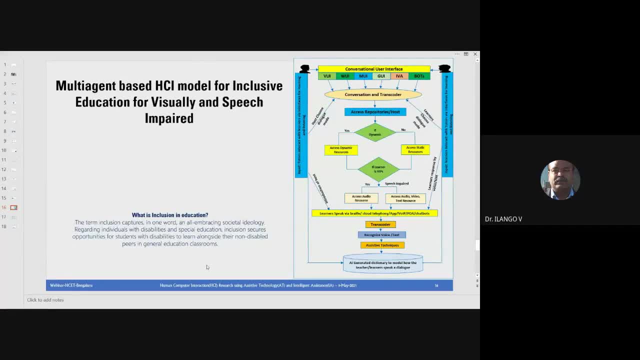 We will be able to understand what the speaker is speaking. Like that the transcoder will do quickly. The real time Least time Latency is very, very least It will be taken. Then move forward. So there are assistive technology. 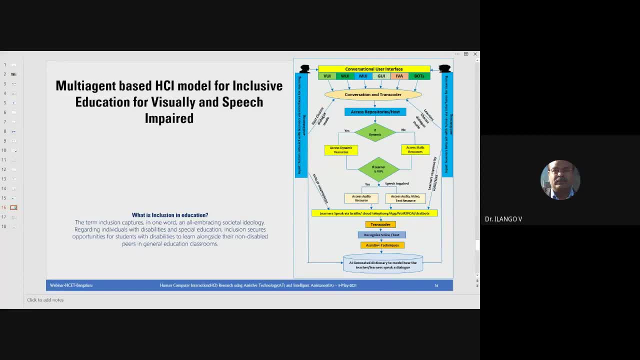 The technology assisting Either with the software support of hardware To respective people: visually impaired, Visually impaired Or hear impaired, Deaf people As well as speechless people. So partially pulling there, According to that, it will segregate and provide. 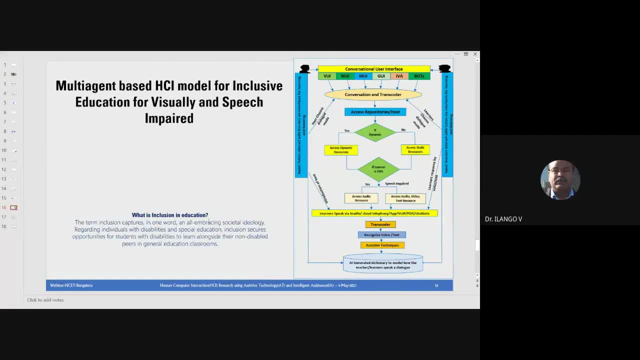 So this was the things we have taken care for 12 months duration- Successfully. we completed. We find the patent. The patent is also accepted And published. also, Now we are in prototype. We are not able to move further Because of the investments. 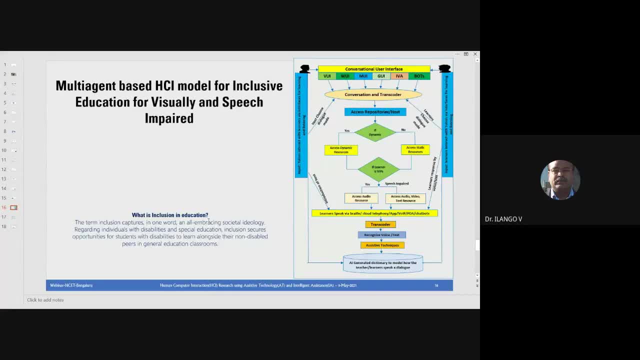 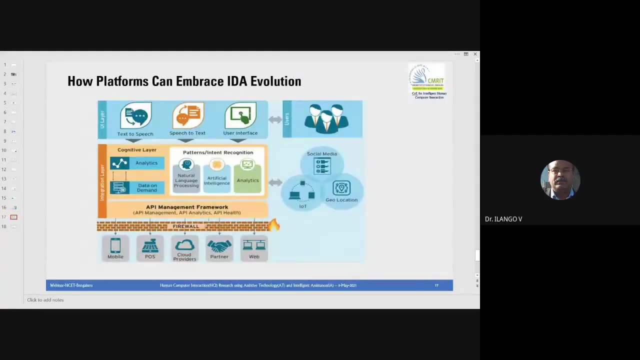 We are approaching the different vendors. Vendors are even accepting. We go approach, The device can be built And the device can come into market. May take some time, But when we do not know. But it is successfully accepted. This is what the interesting things. 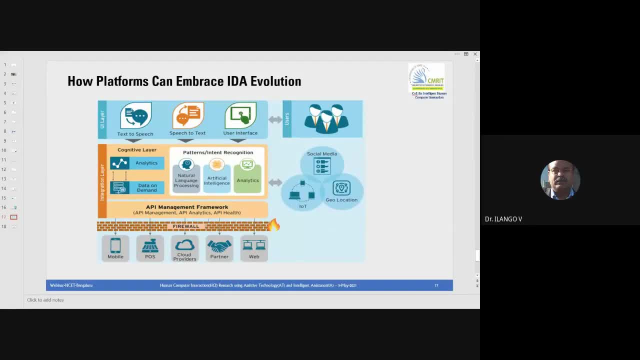 As we do it, We are coming to the last slide: How the interactive assistive technology is helping. From user interfaces: Text to speech, Speech to text. User interfaces are there: User convey. They can type text Text, can convert as a voice. 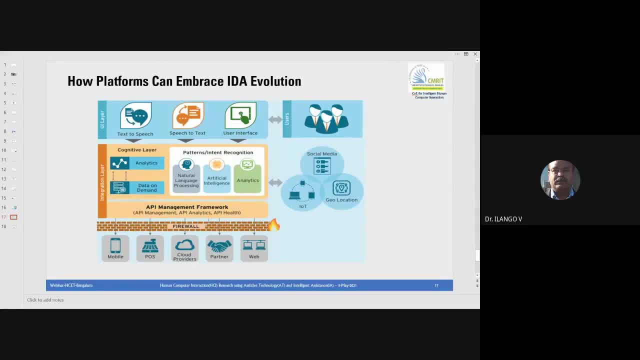 Voice can convert as text Everything. It comes to that middle layer, Middle layer, Cognitive layer. It analyze that. How many people send the text, How many people send the voice? What I supposed to do? This many people are supposed to convert text. 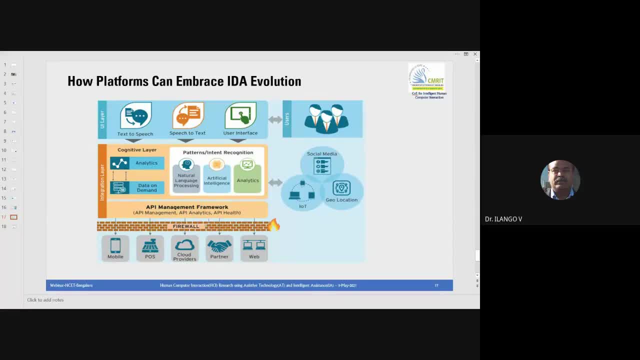 This many people are supposed to convert. as a voice, I get recognized. There is a segregation. There is a patent for it, Using natural language process. Then come back to artificial intelligence, Deep learning system. According to that, Customized algorithms. 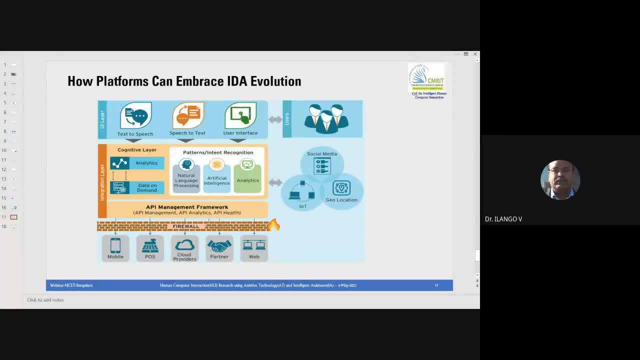 It will be performing successfully. Then it will go As a input Output To perspective mechanism. So this is way We have things: Mobile And previous point of scale And cloud provider And there are various sub partners And web also. 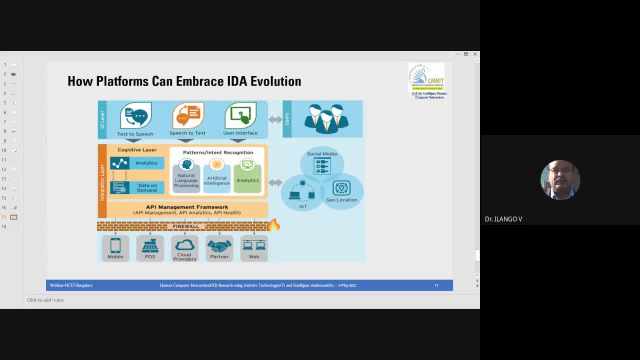 Mechanisms, IOT, Social media Sites And geo locations- All will be utilized there. Geo location is very interesting. This person is in Nagaland, But this person is in India, And this person is in India, And this person is in India. 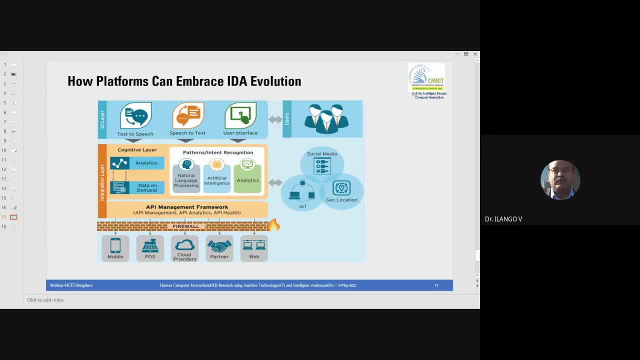 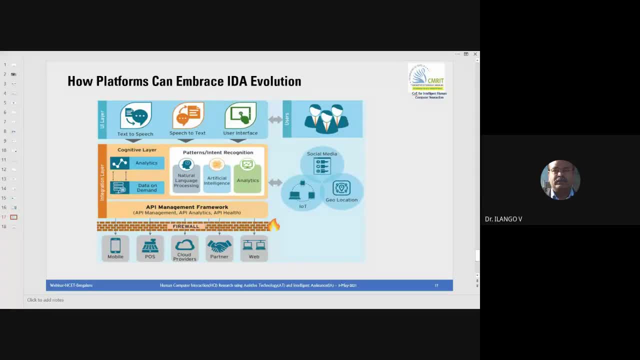 May not be Feasible to reach The network issue, Technology issue, How you are taking to that, And vice versa also. So it is been done, Customized the prototype. So these are all the mechanisms, As we did it. 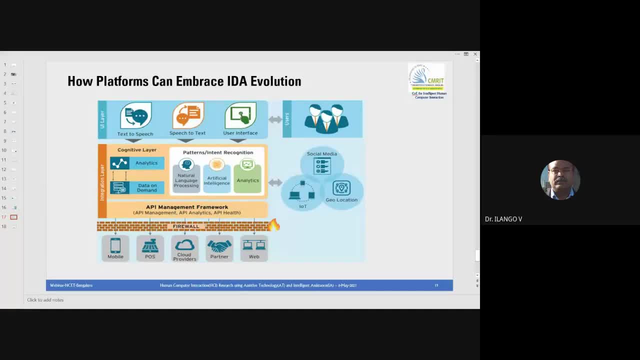 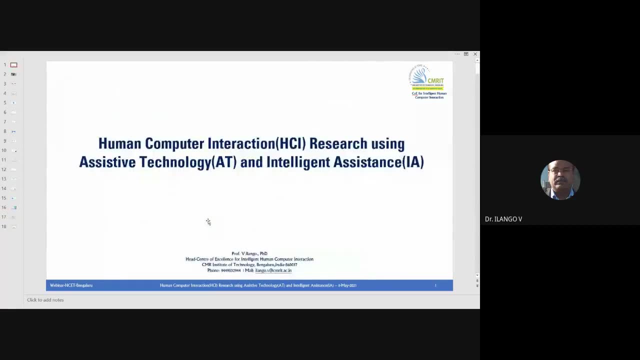 That prototype Or that This is a Internal structure Architectures, How it is performing that. So I will conclude with that. So far we learn Very interesting mechanisms, Computers, human-computer interactions and research using assistive technology. and 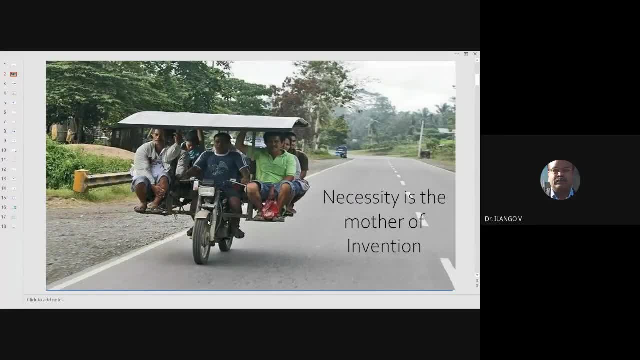 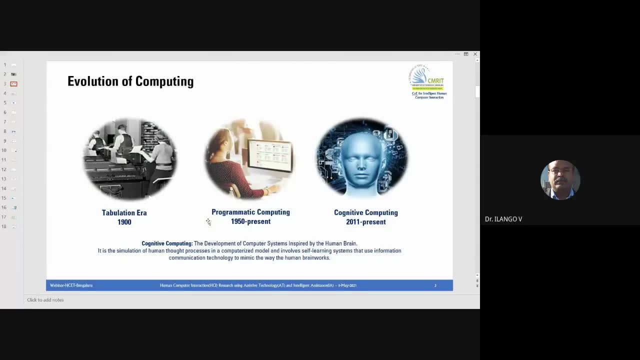 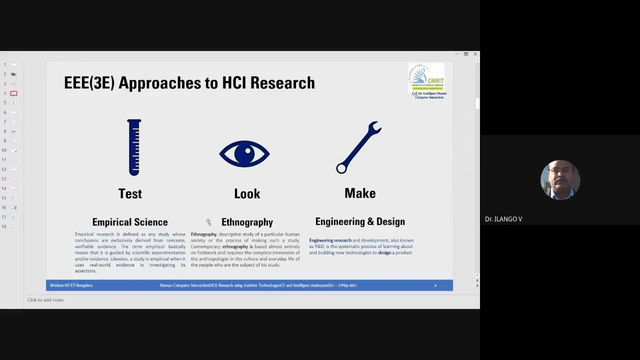 intelligent assistant. why we need to study. we learn what is a innovations require, how innovations can bring into market as a customized product. what are the challenges? is there we have gone through, then? evaluation of computing based on their cognitive computing is a nature of things play in the present. 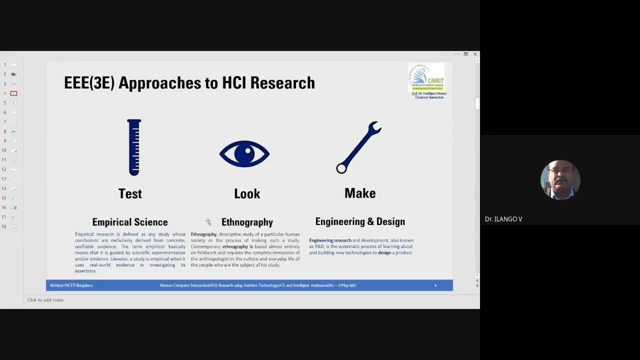 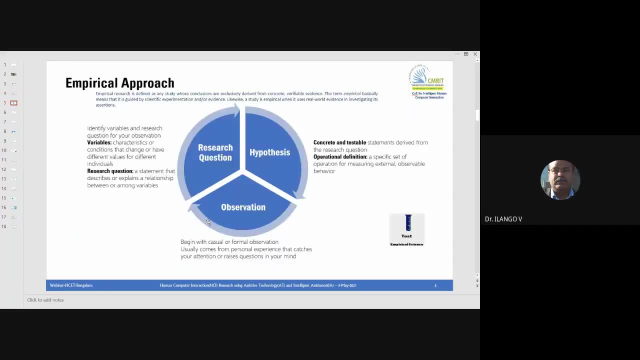 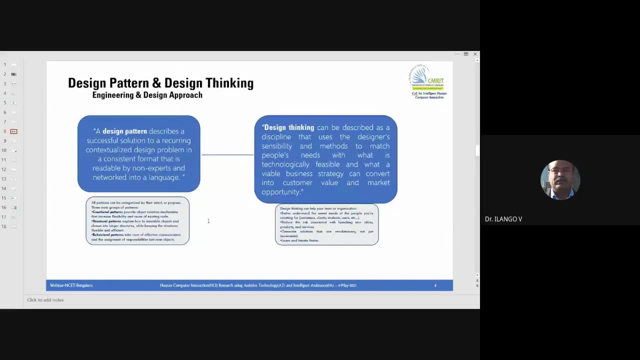 market we learn. how do you go for implementing computing, their human computer? in fact, research 3d was their medical research research approaches, engineering approaches. how do we do empirical research, ethnographic research, engineering research? we have discussed it. for this backbone is design pattern and design thinking. how to do design thinking out of the design pattern? 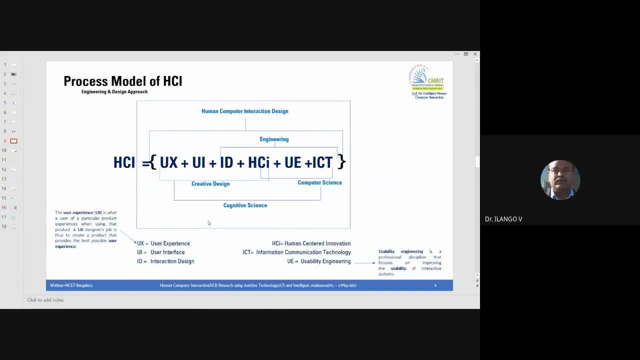 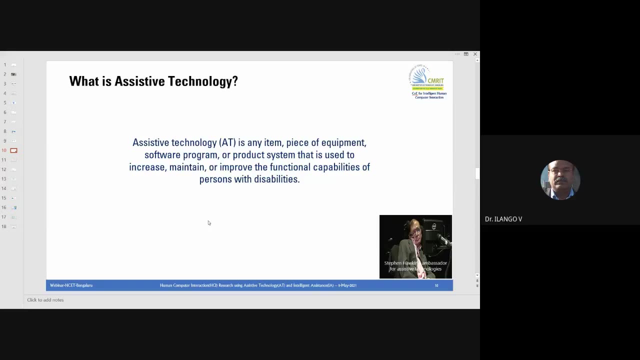 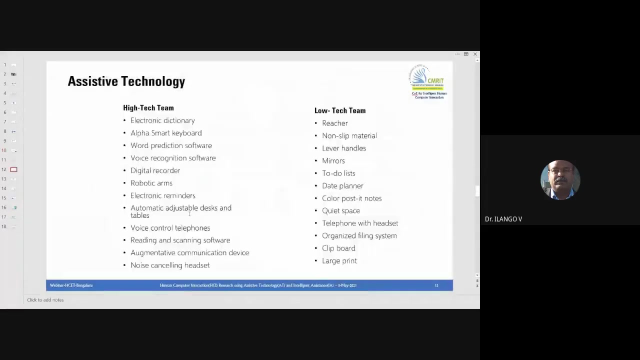 discussing beyond that architecture how to construct a process model of human computing patterns we have discussed with the six element years is an interface, user experience is an interface, interaction design and human centered innovation and use of it. engineering and information communication technology together can make assistive technology and can make intelligent assistance. we have 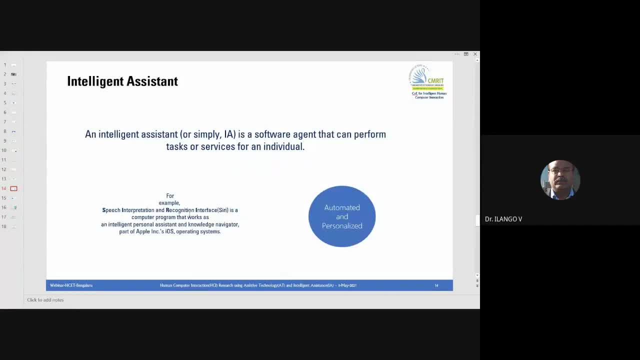 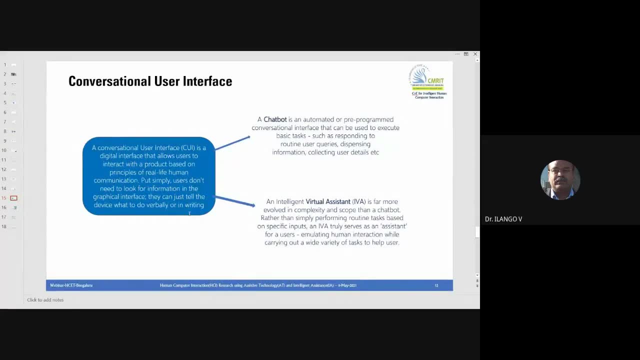 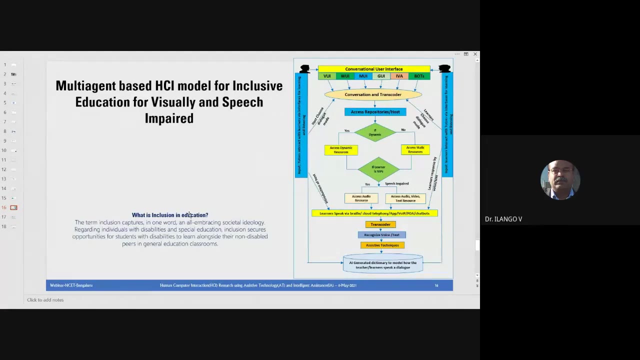 discussed that then. how intelligent assistance came to pictures- already discussed that then. conversation is play major role to make a communication agent between intelligent assistant as well as assistive technology we have discussed. we discussed the real project which is been pretended I actually done in the or in center of excellence. many more projects are going on I have 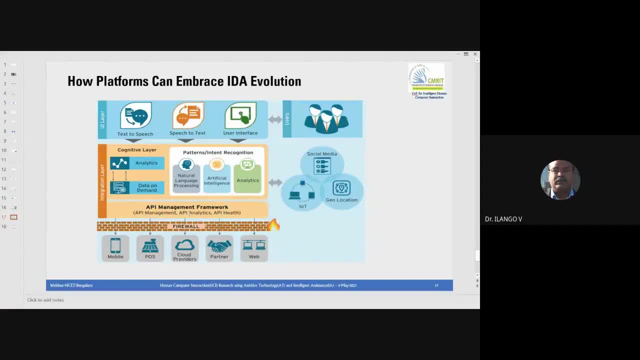 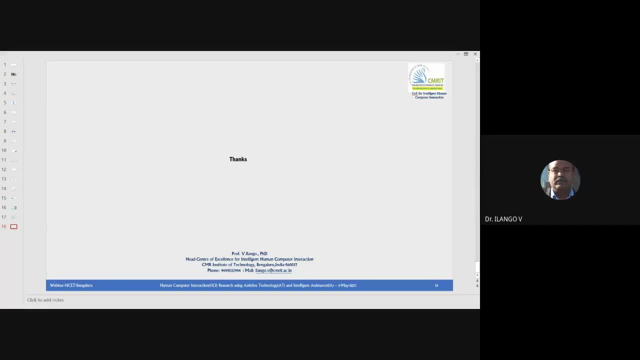 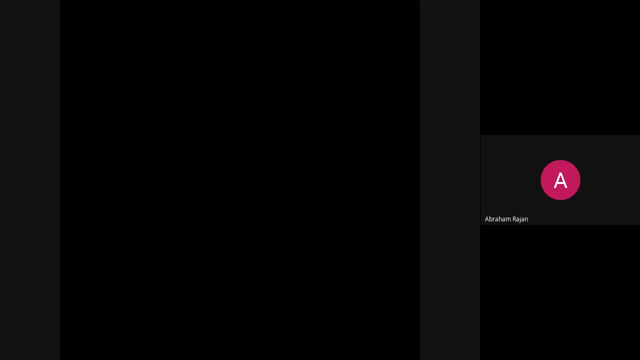 demonstrated, just not that typical solution due to confidentiality. so this is my presentation: this forum for asking questions. anybody has any questions come forward? thank you, sir. thank you, sir, for giving valuable insights regarding the topic human computer interaction, research using assistant technology and intelligent assistant. now we will go ahead and take some time for questions. forum is open for questions. 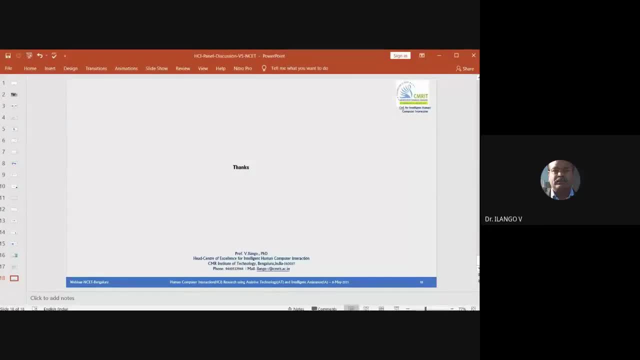 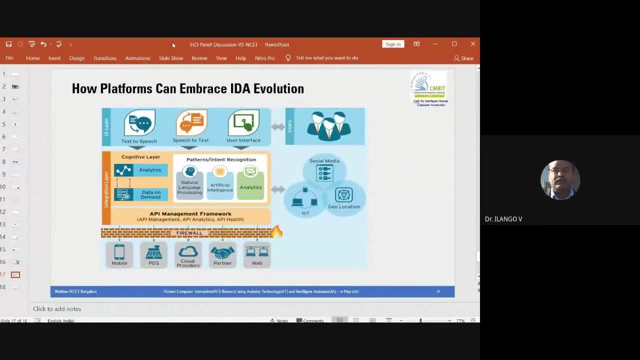 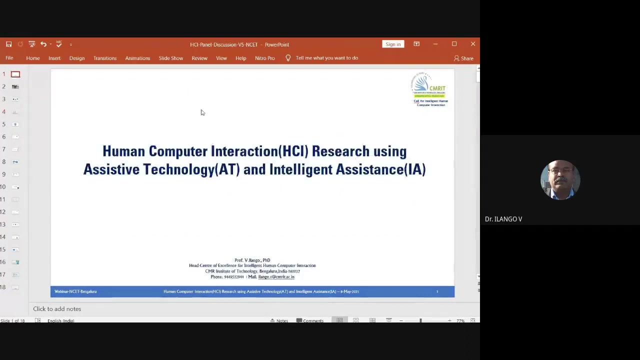 so audience participants, professors, students, we can ask questions. if you have questions, you, you, you, you, you is you youth a, they are chair, they, they are doing the, if you feel that, I think. thank you very much for your very informative preparation, sir. we can understand by seeing your slides how much effort you put for preparing the. 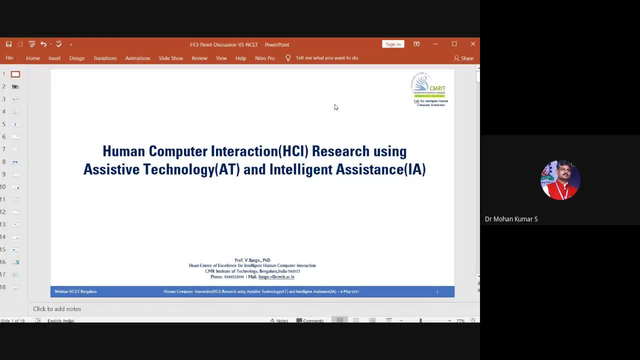 slides and, from starting to ending, without losing your energy, you presented all the content, whatever you prepared, to all our audience. we are very grateful to you. we will share our resource: persons, email ID, students and staff members who wanted to clarify doubts. if you wanted to have any support from professor you. 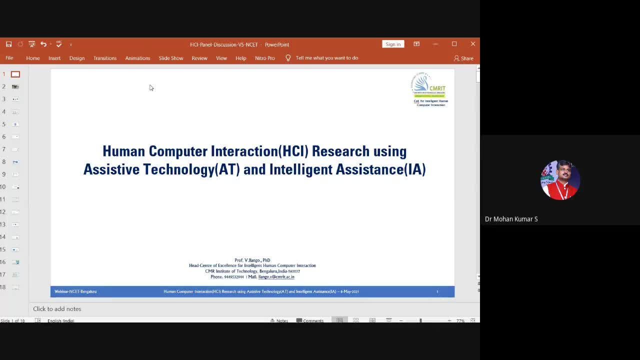 can approach him through email and even mobile number also, we will share already professor shared. you can approach professor through this email ID and mobile number. I would like to thank our processor for accepting our invitation and presented this wonderful webinar. thank you, sir. thank you, sir, thanks for. 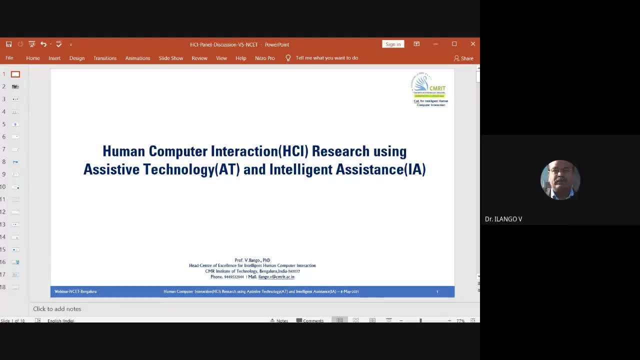 giving opportunity. and here's the entire department come to change the point. thank you, sir. thank you, sir, thanks for giving opportunity. and here's the entire department come to change the point. and quality, students, department and management and special thanks to principal sir and Dr Mungadara. sir, please convey regards to everyone. thank you, sir. we will intimate, sir, we will intimate. 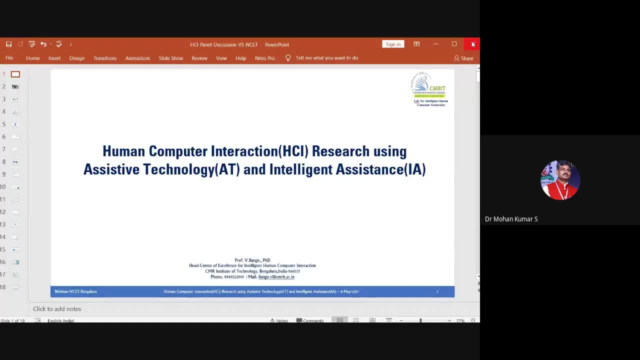 the feedback form we shared. please, I request all the participants to fill the feedback form and we will share the certificate in a short while. shall I exit, sir? thank you very much sir. thank you very much sir. yes, we can log off, sir, we can log off sir. thank you very much sir. thank you very much, sir. we can log off. 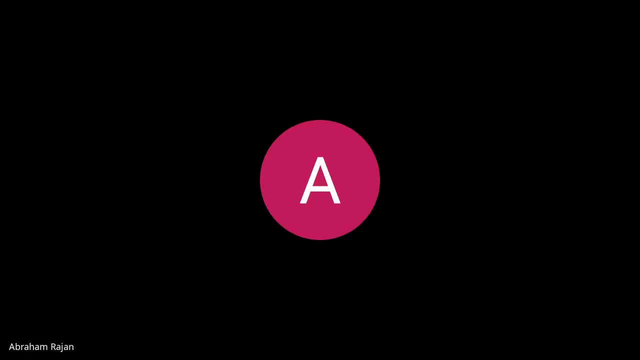 sir. thank you very much sir. thank you very much sir. thank you everyone. thank you professors who are all join and professor Abraham, you can complete what of thanks if you. yes, sir, thank you everyone. it was a pleasure being with you all today through this online platform. I would like to thank everyone who made this meeting possible, especially. 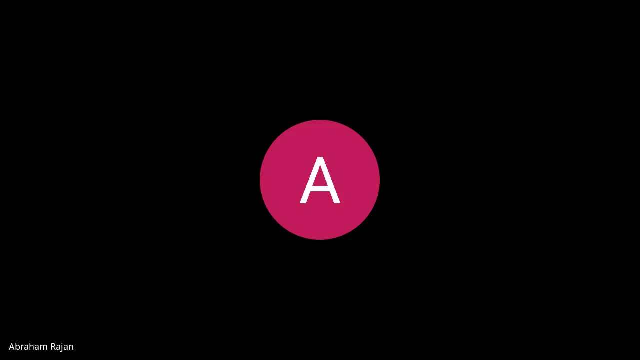 platform. I would like to thank everyone who made this meeting possible, especially platform. I would like to thank everyone who made this meeting possible, especially thanks to our dr B Elango sir and our principal. thanks to our dr B Elango sir and our principal. thanks to our dr B Elango sir and our principal, dr Jitendra Mungaro sir and dr. 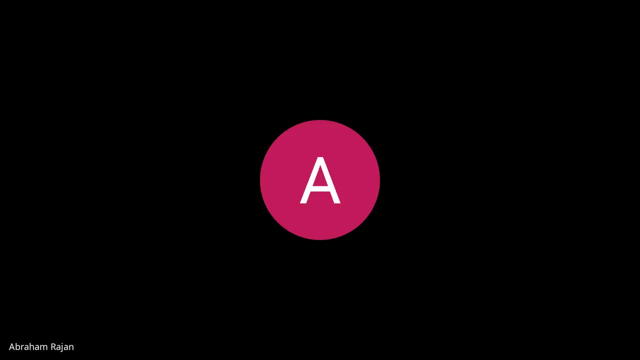 dr Jitendra Mungaro sir and dr dr Jitendra Mungaro sir and dr Mohan kumar sir, and I also like to thank Mohan kumar sir, and I also like to thank Mohan kumar sir, and I also like to thank all participants. and one more thing: we 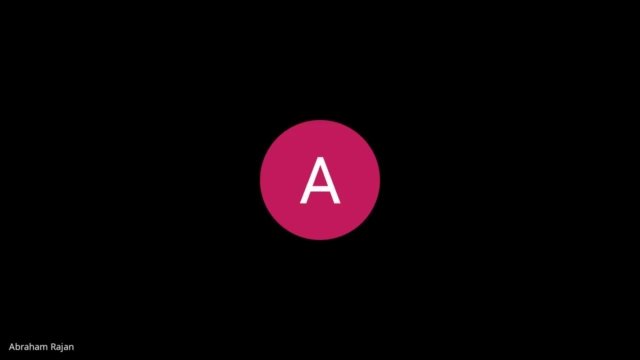 all participants. and one more thing: we all participants. and one more thing: we have posted the feedback form link in the. have posted the feedback form link in the. have posted the feedback form link in the chat box. you can copy that. you can click chat box. you can copy that. you can click on that link and fill in the feedback. 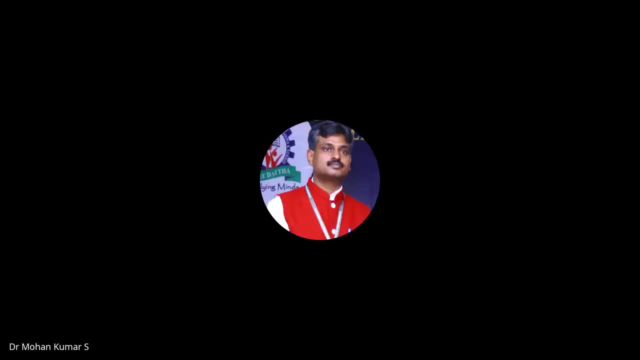 on that link and fill in the feedback on that link and fill in the feedback form, my special appreciation to form my special appreciation, to form my special appreciation to coordinators: streak on the professor coordinators. streak on the professor coordinators. streak on the professor Sandhya, professor Abraham and mr Perry. 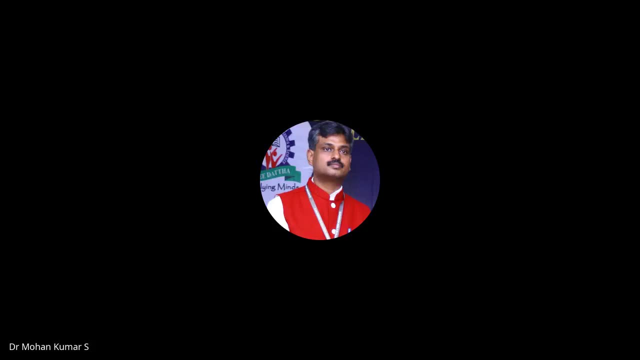 Sandhya, professor Abraham and mr Perry. Sandhya, professor Abraham and mr Perry. Sami and other coordinators who are Sami and other coordinators who are Sami and other coordinators who are supported to conduct this event. a very supported to conduct this event. a very 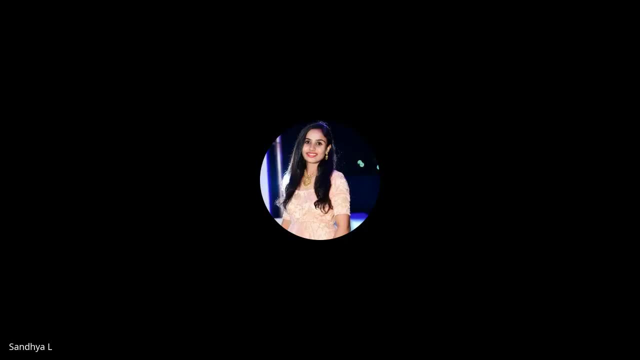 supported to conduct this event. a very grand success. thank you very much. thank grand success. thank you very much, thank grand success. thank you very much. thank you, sir. thank you, professor and all you sir. thank you professor and all you sir, thank you, professor, and all the participants, all the professors and. 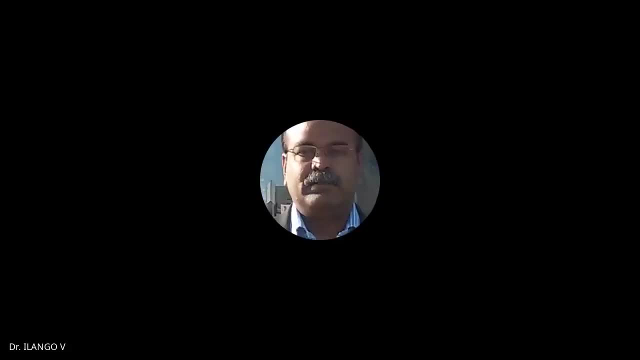 the participants, all the professors and the participants, all the professors and you by the children. yes, sir, thank you. you by the children. yes, sir, thank you. you by the children. yes sir, thank you, have a nice day, I'll sign up. thank you, have a nice day, I'll sign up, thank you.